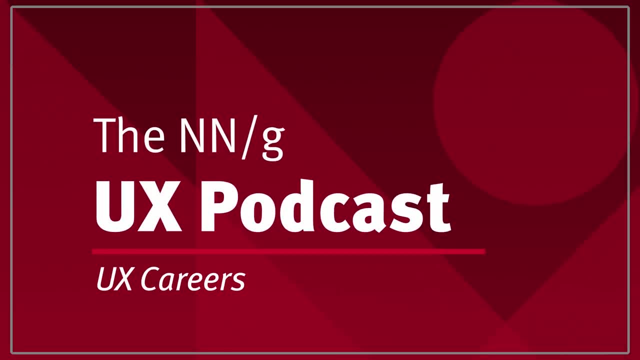 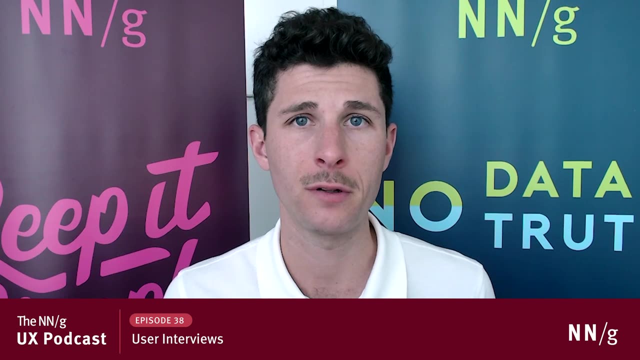 This is the Nielsen Norman Group UX podcast. Welcome to today's episode, which features a conversation between Therese Fassenden and Steve Portigal. Therese and Steve discuss user interviews. They talk about how this research method changed over the years, what the main benefits and biggest challenges are And towards. 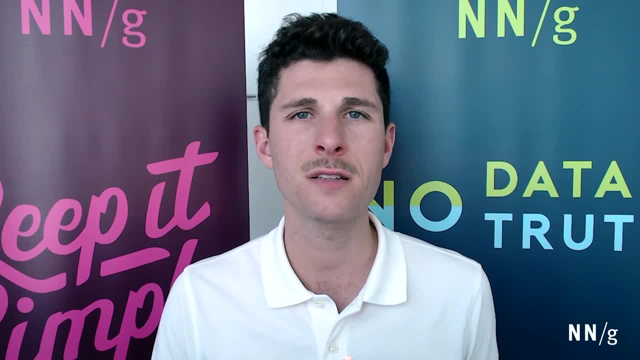 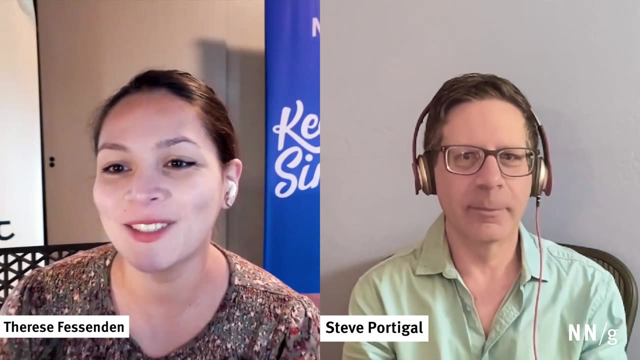 the end of the episode, Steve gives some practical advice for how to avoid some common mistakes many interviewers make. Join us as we dive into the conversation with Therese and Steve and explore the art of user interviews. Steve, welcome to the podcast. I'm excited to chat with you today. 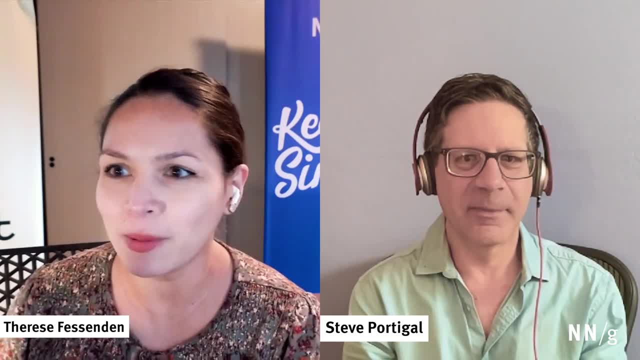 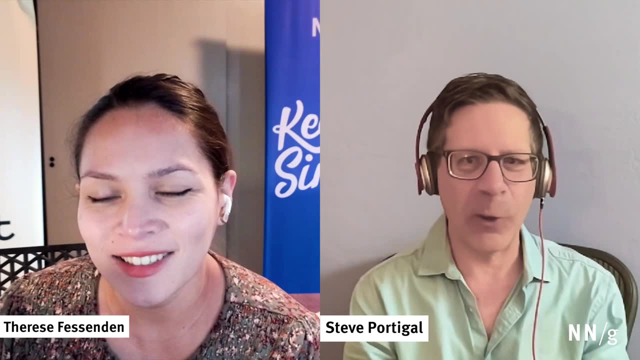 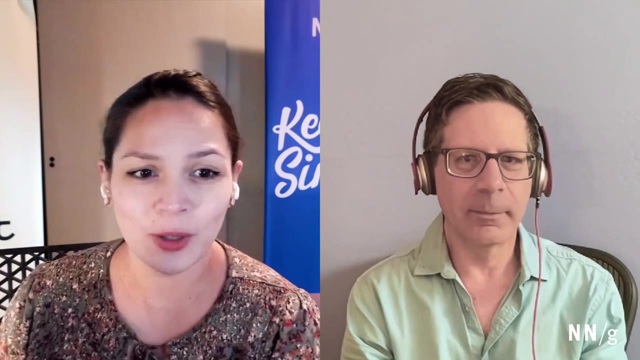 about user interviews. It blows my mind that we haven't had an episode on this topic, and who better to have on the podcast? Yeah Well, thanks for having me. I'm looking forward to our conversation. Yeah, So yeah, and interviews are probably one of the more, if not the most popular methods in UX. 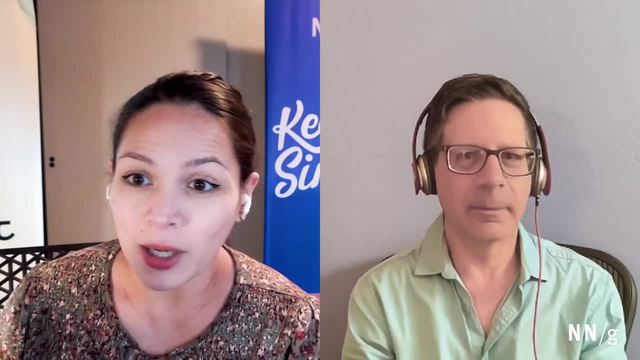 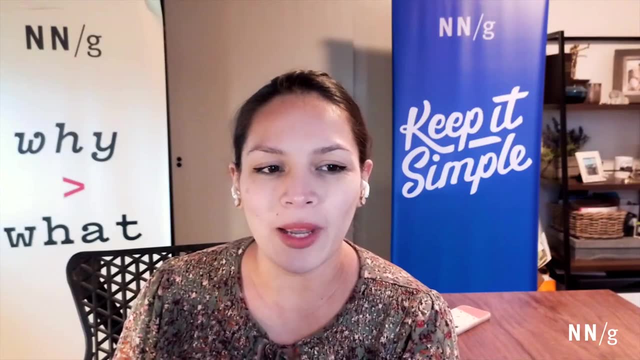 research right. After all, it's if we're going to make better products and services, better experiences. who better to talk to than the people who are going to be using it? I would love to know a bit, just to kind of give an introduction for folks who've maybe never done one before- never. 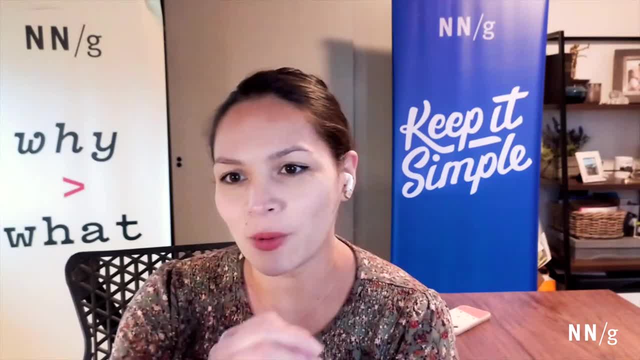 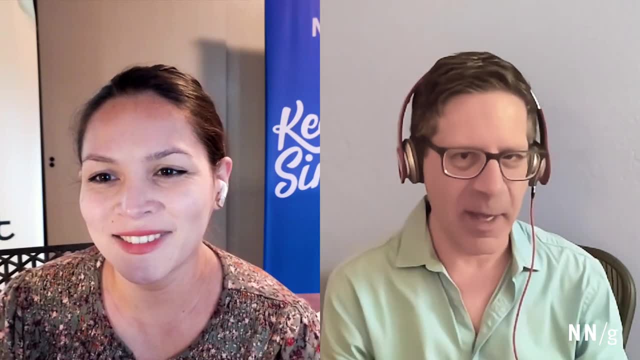 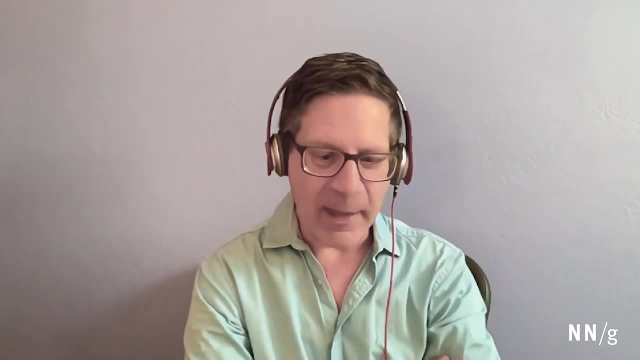 really even heard of these. What would you say? a user interview is. You know, when you look for definitions, there's a good way to start an argument. Well, that doesn't count as this, That doesn't count as that. So I'll give my kind of sloppy perspective, And I think people may have variations And I 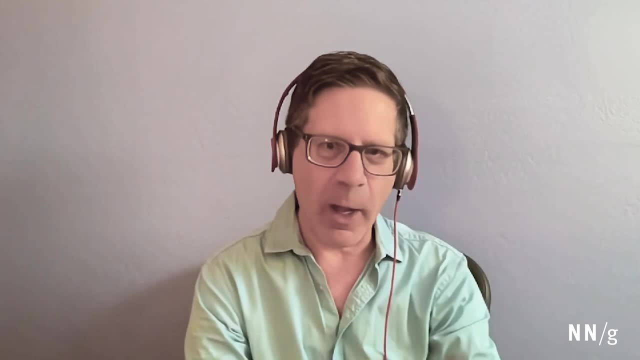 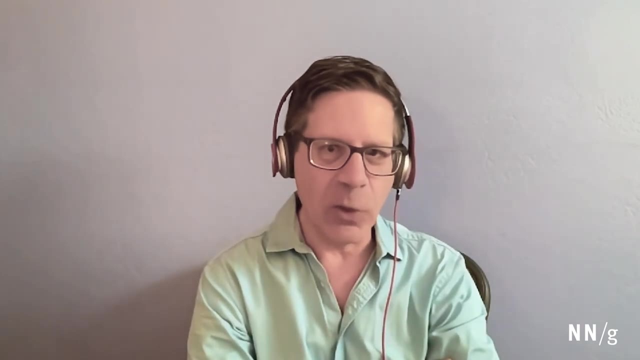 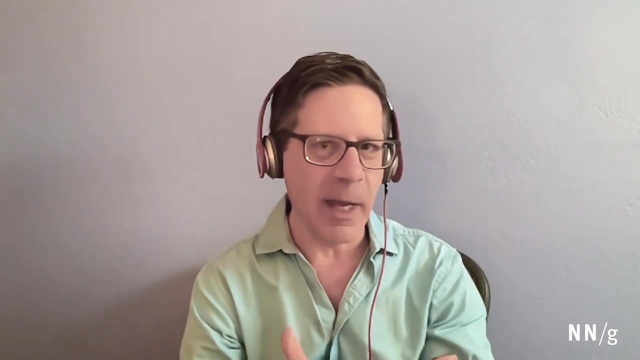 tend to be a little generous in what I include as an interview, And I think it's an activity as well as a method, right, So you can do lots of quote unquote methods that still involve an interview, Like you might run a usability test where you have something that's going to be. 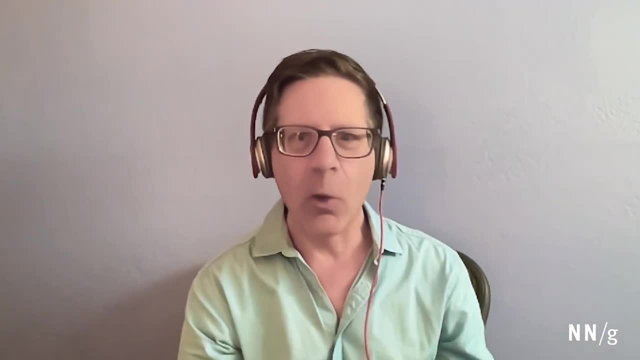 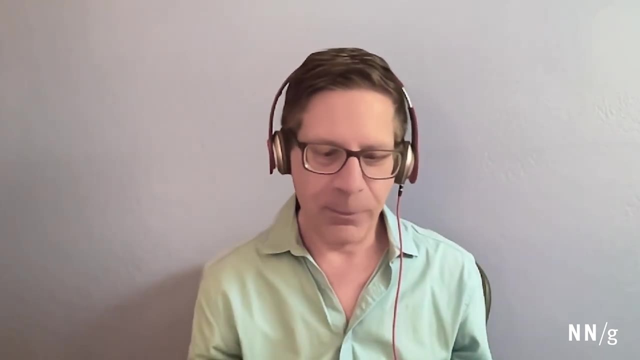 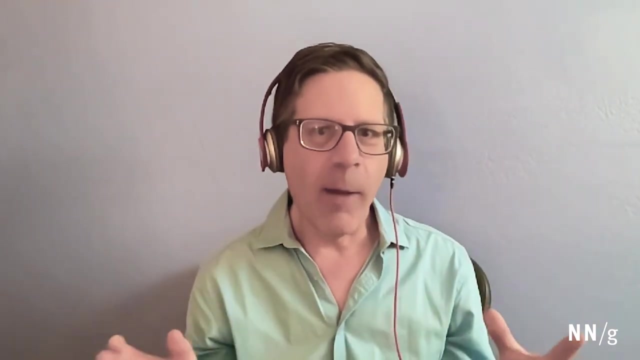 done by somebody, walk through a set of scripted tasks with a prototype, but you might interview them before or afterwards, And so that's where I think I get a little sloppy with my definition. So I guess that's not an interview overall, but you are sort of using interviewing as a process. 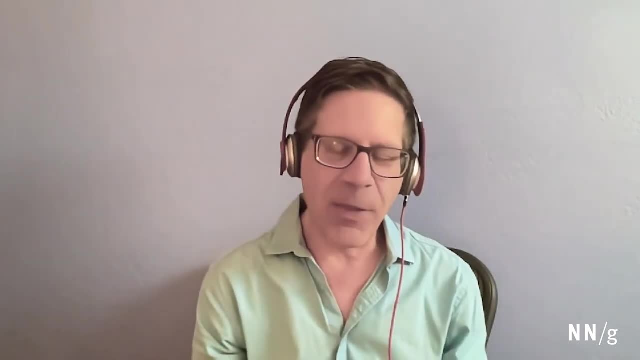 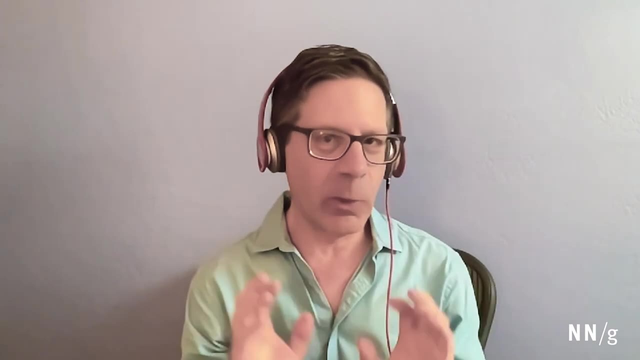 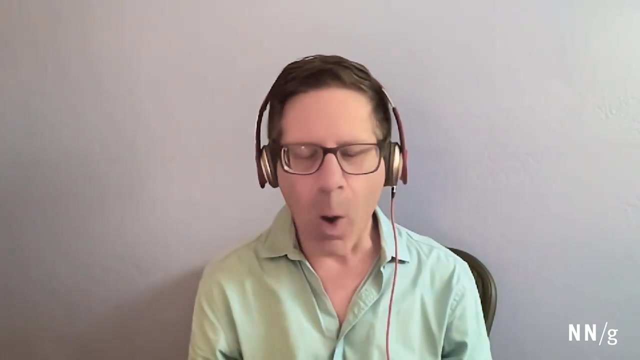 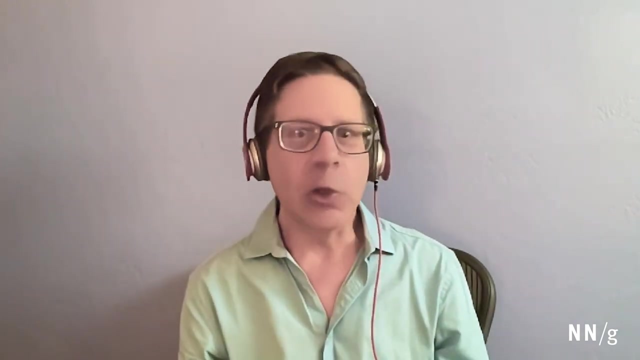 or as a tactic to do that. But I think, yeah, if you step back, an interview is a conversation or it looks like a conversation. We use very different tactics to have this quote unquote: conversation between one or maybe two researchers and one or maybe two users, customers, participants. 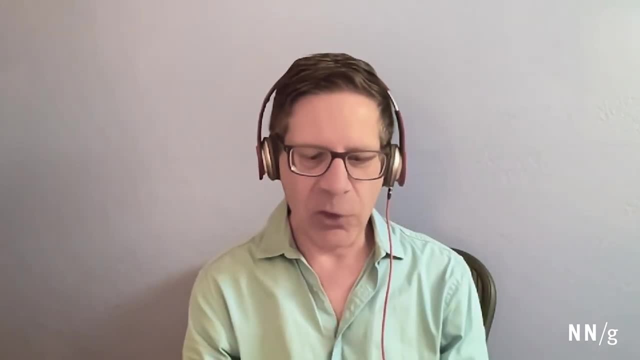 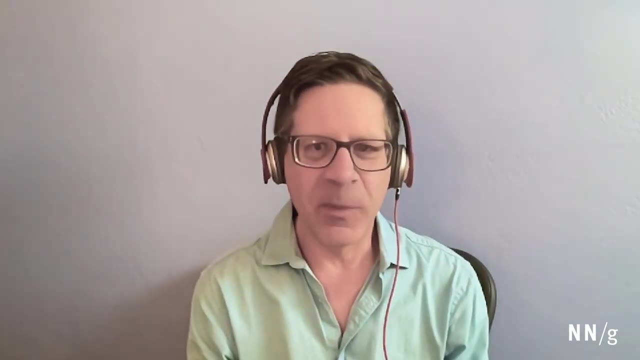 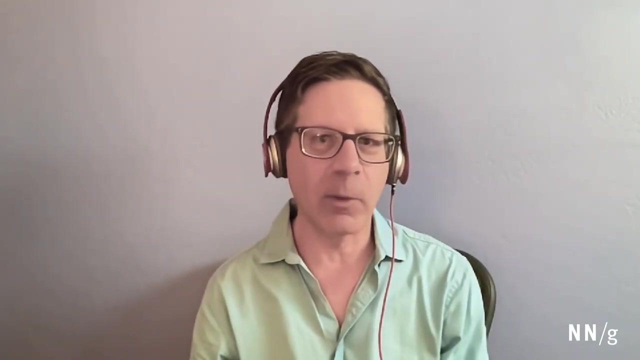 kind of call them what you want. There's jargon that comes up like semi-structured, which I don't even want to try to define open-ended. When you do an interview, you have some prepared questions, but then the conversation goes in different places. You ask: 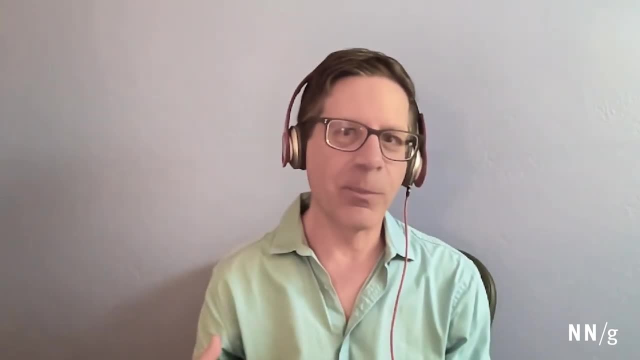 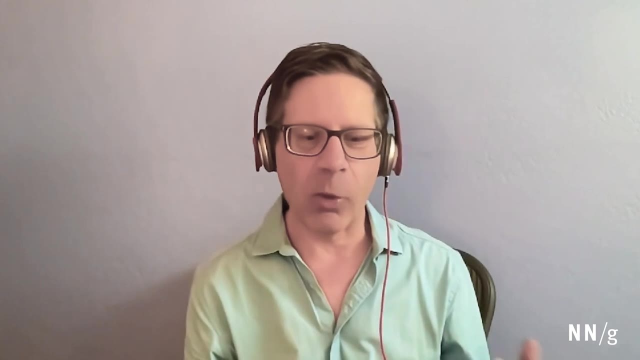 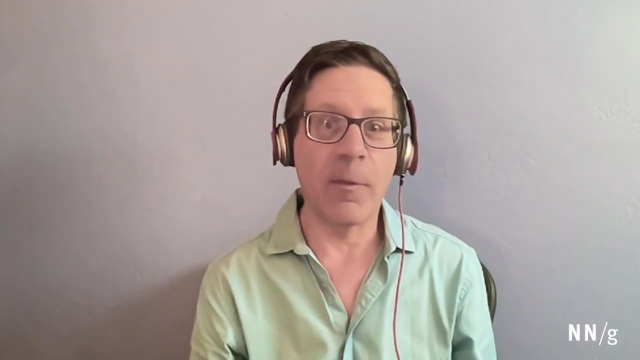 lots and lots of follow-up. So it's not like a verbal survey where it's question: give me your answer. Next question: give me your answer. You are trying to explore, And so interview A and interview B are going to be a little bit different, Even if you have the same kind of population. 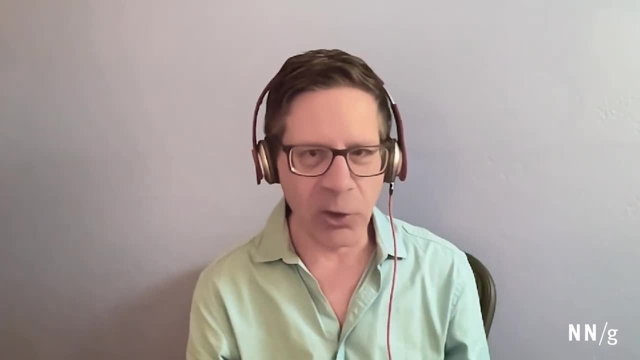 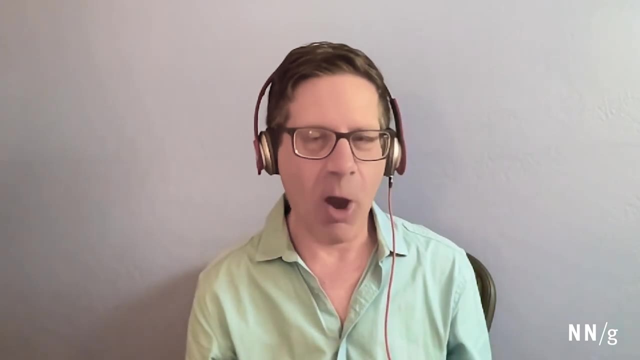 you have the same sample, you have the same discussion guide. So there is, yeah, kind of an emergent exploratory nature to the conversation. Even if your topic isn't exploratory, you still want to explore with that person and sort of ask more and ask more. 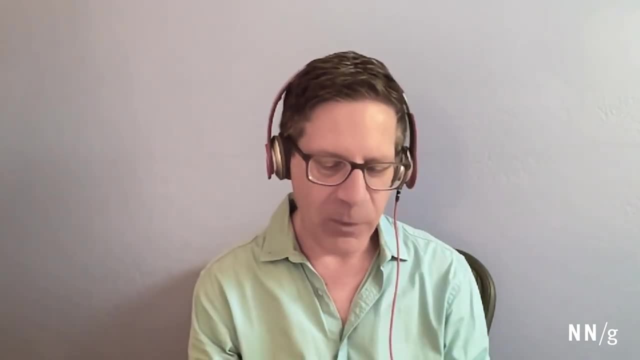 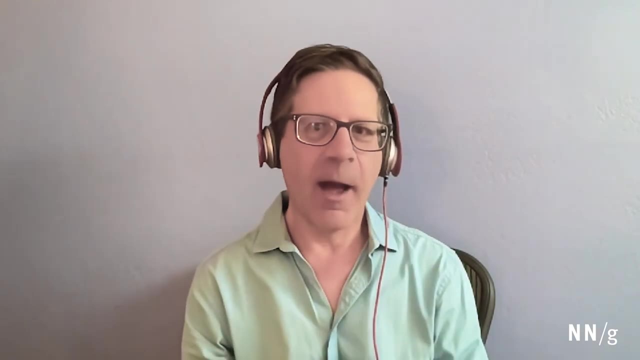 try to get to something before you kind of move on. So that's kind of what an interview is like. I think there are other aspects, like where does that interview take place? And because so much is online now, like the conversation we're having, a lot of that is. 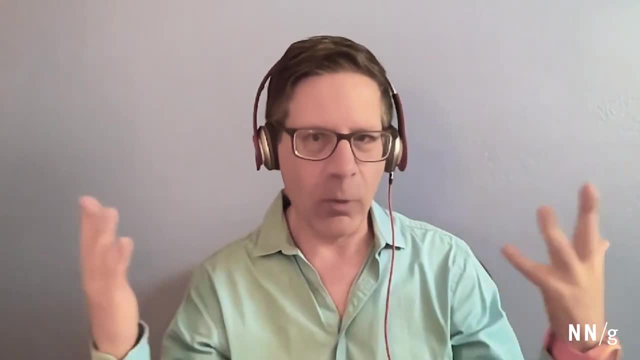 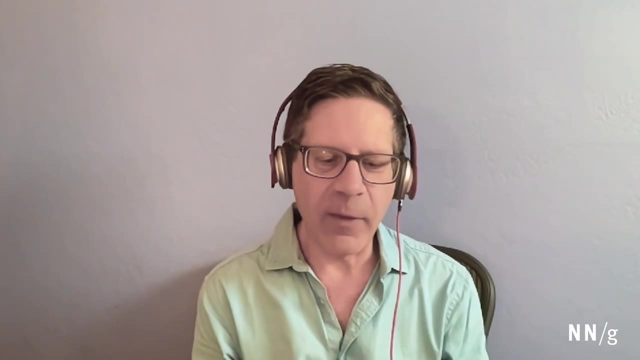 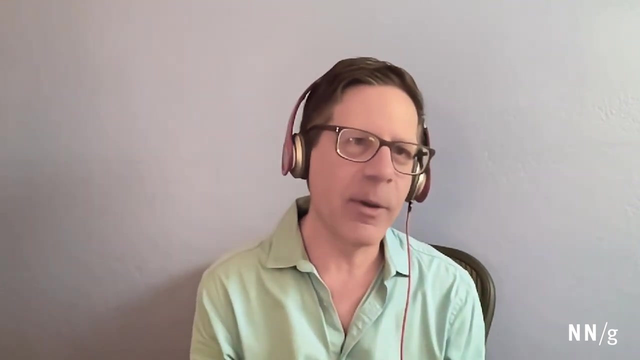 happening. It's happening in sort of remote online virtual environments, I think. if we go back to sort of in-person stuff, I don't think if you bring somebody or have them meet you in a market research facility or usability lab, it's still an interview, but you're kind of changing some. 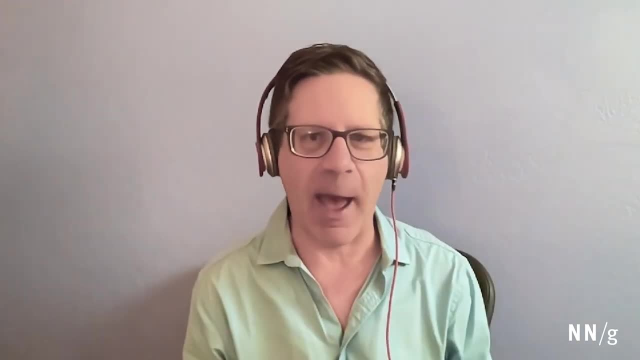 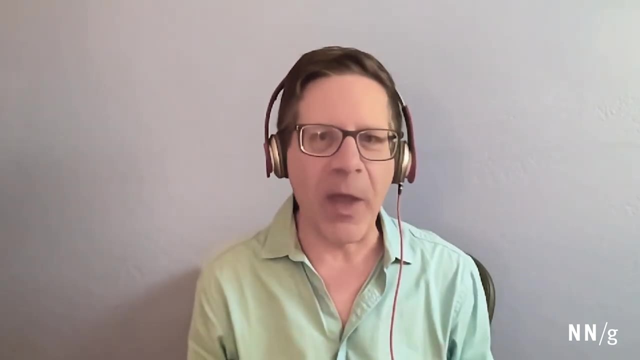 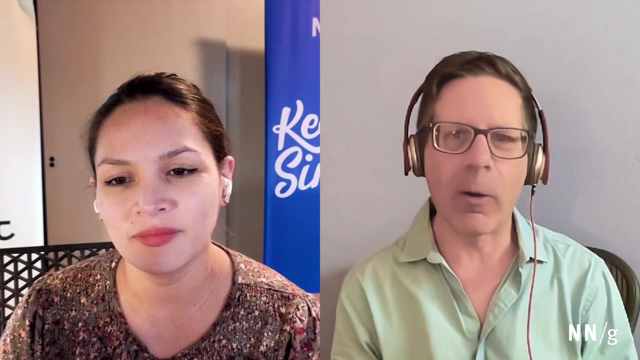 of the nature of it. Ideally there's an in-context aspect to it, where you are asking that person about their experience and you are seeing their things and how they work on their devices and what their process is in their environment and so on. So kind of getting as far into their context as you can, depending on the logistics. 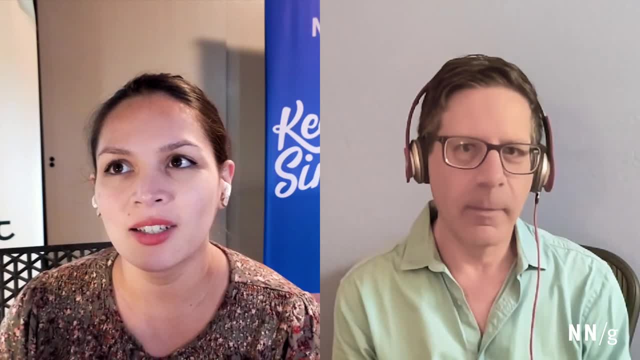 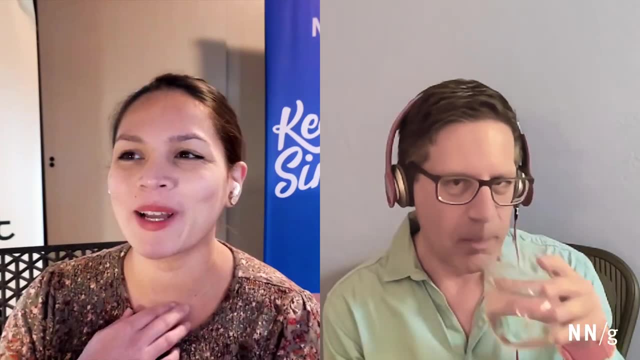 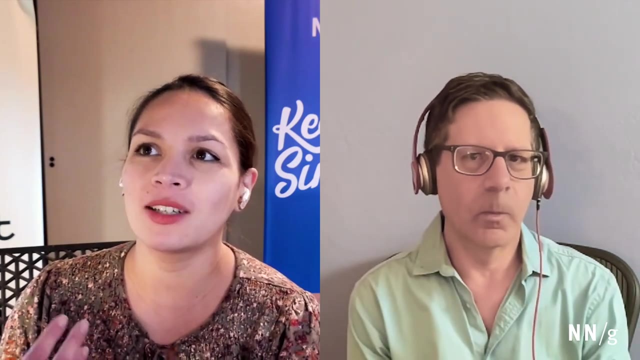 of how you approach it. Yeah, I appreciate what you said about this method seeming like a conversation. I mean, anyway, it is a conversation, but I appreciate that you frame it this way because I feel like there's this expectation around interviews being a certain 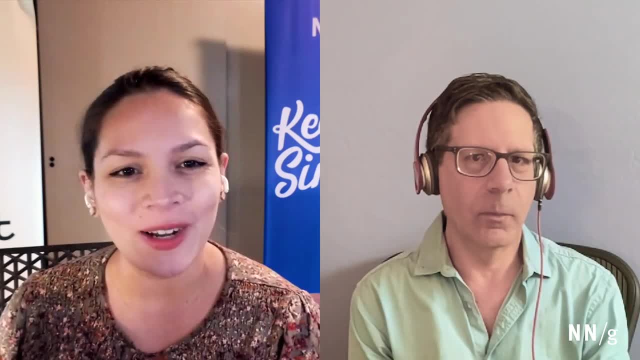 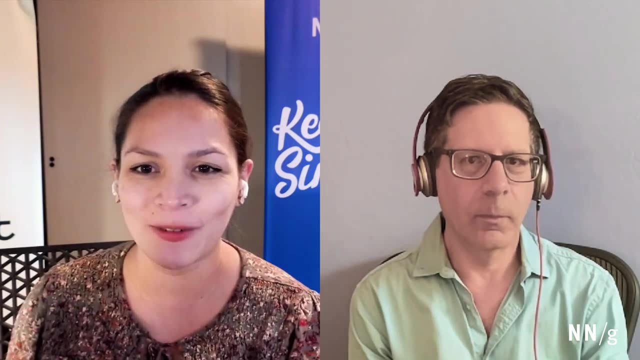 way, And part of that is: I mean for one, we're on a podcast right now. right, We're doing a podcast interview. Podcast interviews are going to be totally different from, like, a research interview, where your goal is going to be very different, And, similarly, where you're having a conversation. 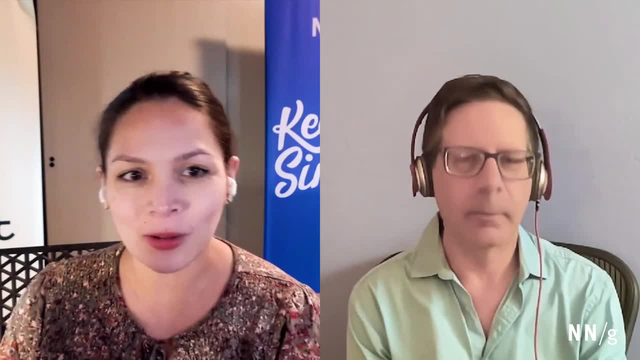 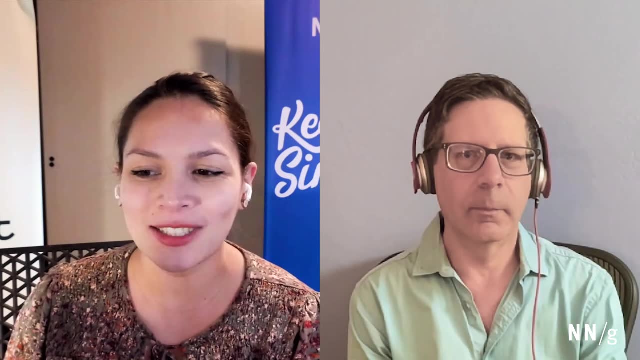 with a friend relating with them on a deep level. that's also going to be a little bit different from, say, a research interview, And I think it's important to note that it's not just any old conversation, but one where you're really trying to get to know that person on the other side. 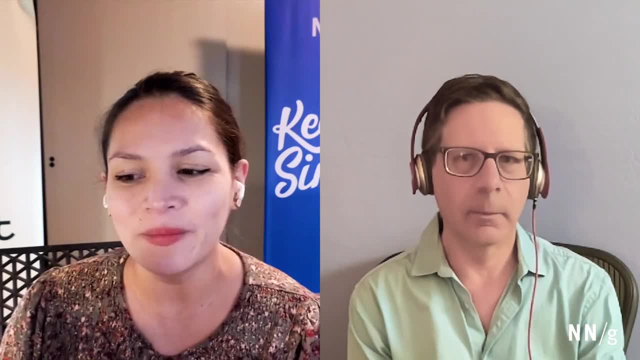 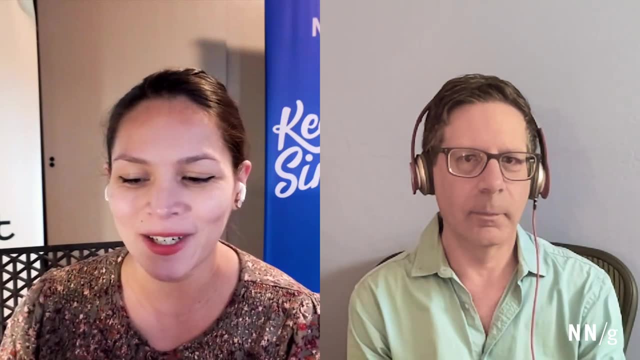 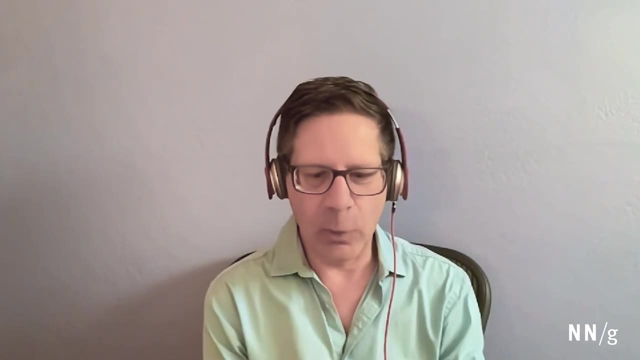 The user, the participant in this case. So actually I kind of want to get to know: how did you get into research, How did you get so fascinated by user interviews in general and just research in general? I was lucky to- I guess I would call it- stumble upon this as a way of 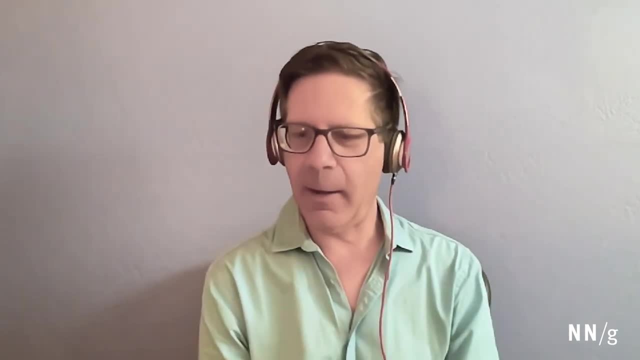 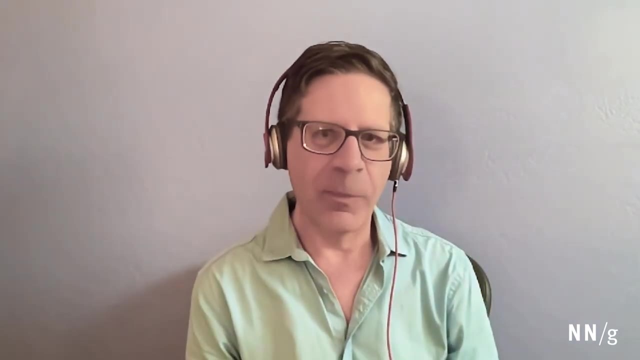 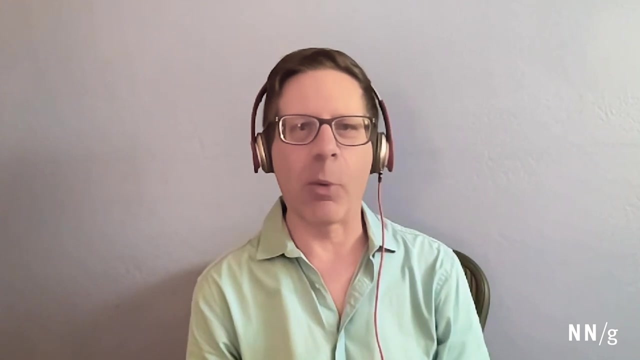 working kind of early in my career And I had a. I had a degree in human computer interaction in the days before the web, in the days before we talked about user experience, where this was a kind of a design activity and people had portfolios and you know and processes and so on. So I had a. 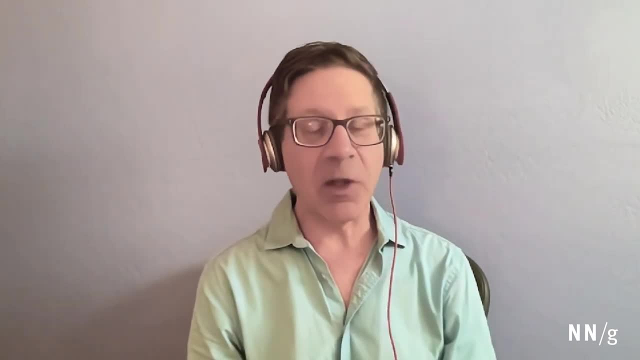 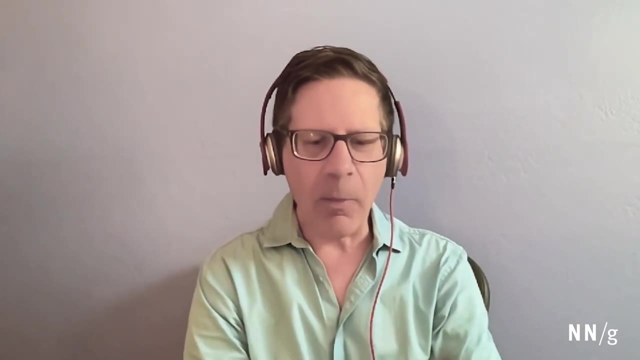 degree but not really, not really a skill or any expertise in making a thing. And I ended up working in this design consultancy that was doing a little bit around kind of software And I don't know. we didn't really call it design, It wasn't really practice-like, But it was kind of a. 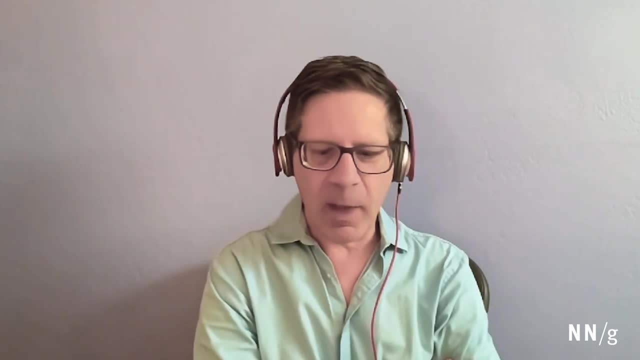 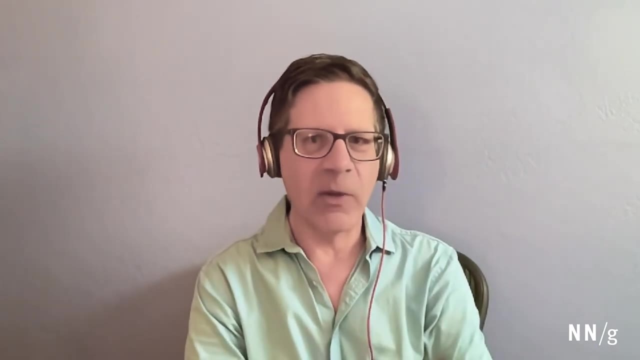 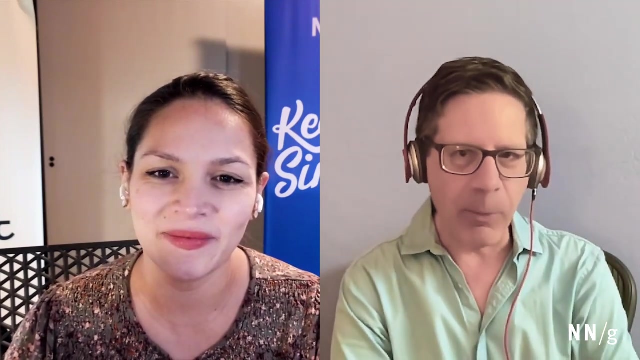 design, But elsewhere in this organization was an emerging practice in helping organizations that they were serving figure out what to make as opposed to how to make it, And it was really saying that, hey, there's work to be done in understanding the problem space, understanding. 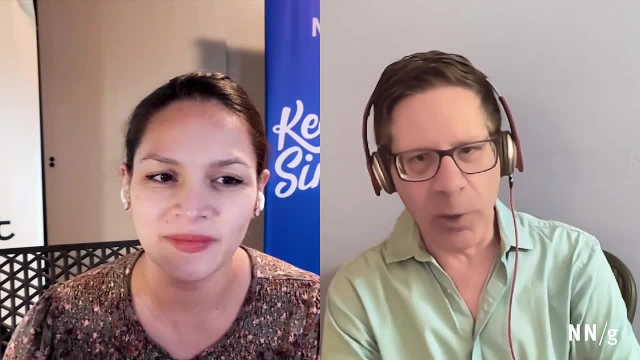 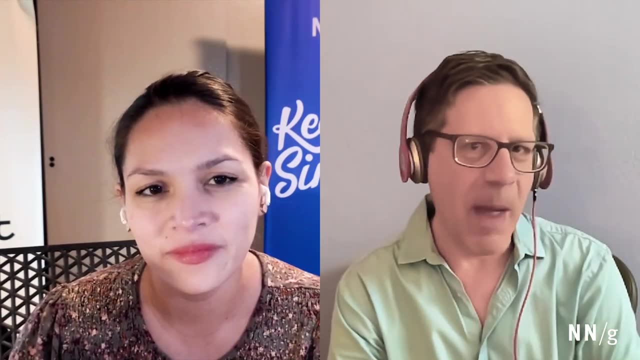 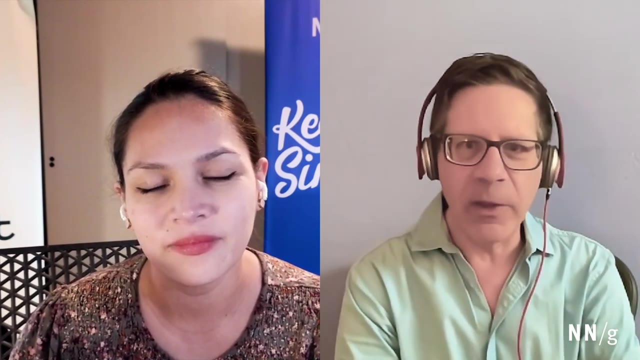 the users. And it was cool because we didn't call it user research. We called it. we called it based on the outcome. What value were we bringing? And research is a method to get to that. So you know, in doing this work and learning kind of on the job and this sort of quasi-apprenticeship. 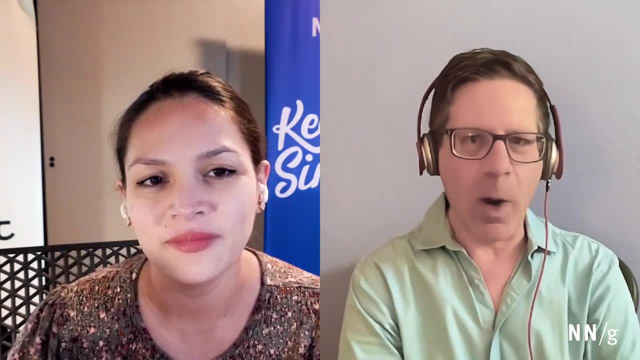 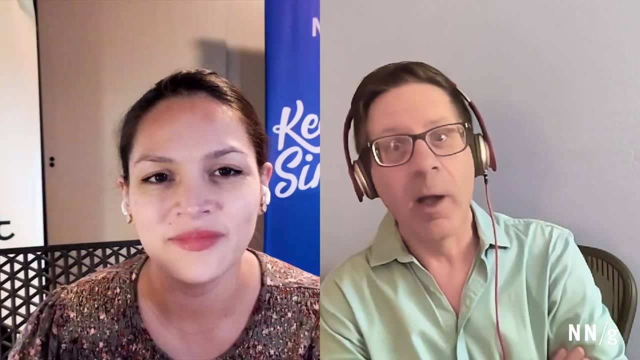 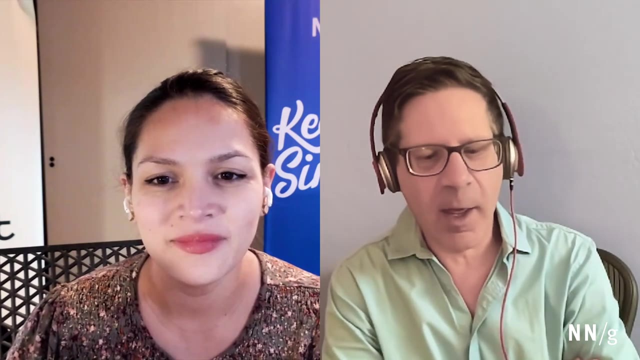 experience that I had, you know I got to see what happened in interviews And I got to kind of tag along in interviews And I got to practice asking a question And I got to eventually lead interviews and teach other people how to run interviews and you know work on a process for how you make sense. 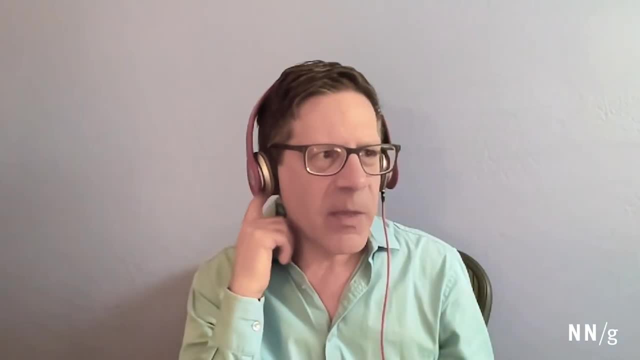 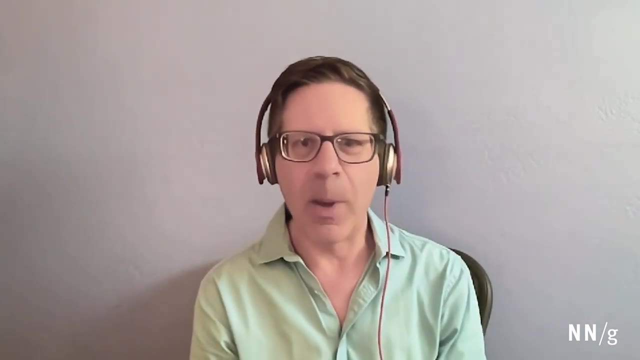 of this stuff that you get in a quote conversation And I got to kind of learn how to make sense of the conversation. I think it was with the interviews where, and you know, I really had to work hard to learn it, But once I felt like I was learning something, there was, I don't know, 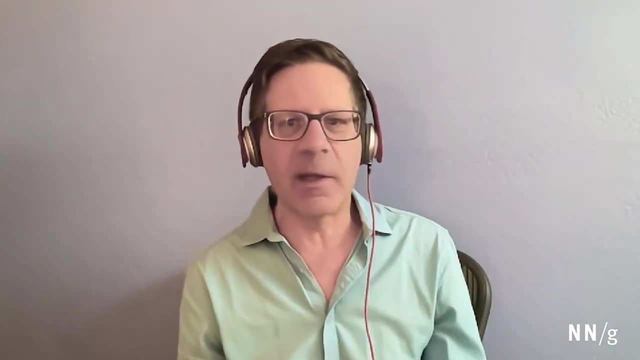 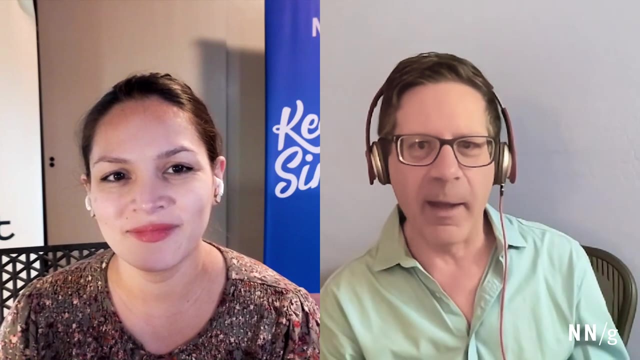 a switch kind of flipped for me, Like, oh, this is this. not only is this a thing, but I think this is my thing. I'm still learning. I mean, you learn about people every time you do that, but you also learn about the practice of asking questions, of interviewing people. 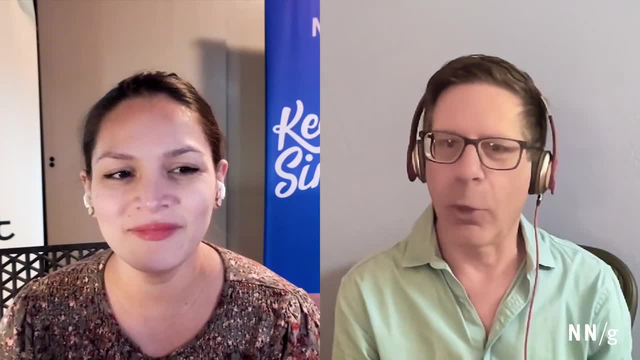 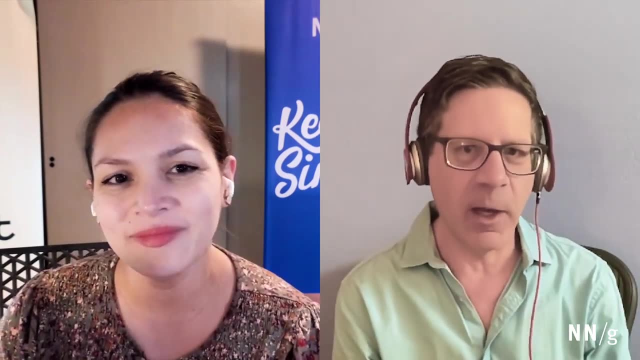 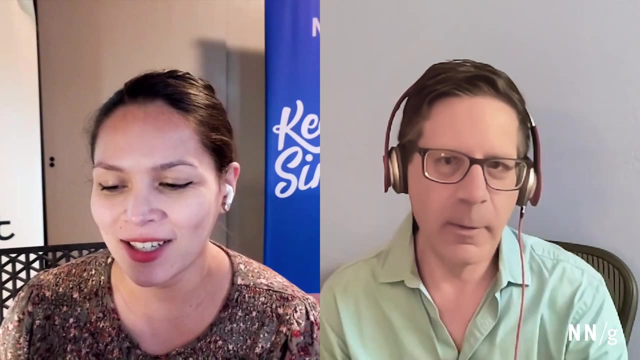 every single time, Um, you know, through making mistakes or just having some reflections about it, So that it continues to excite me and challenge me. you know, as I've been doing it all these years, That's amazing And I agree, This is one of those methods that I started learning Um. 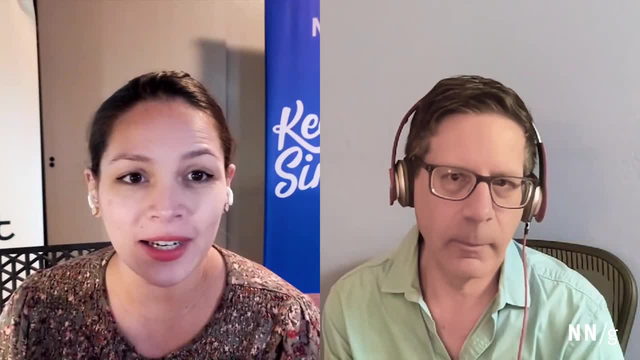 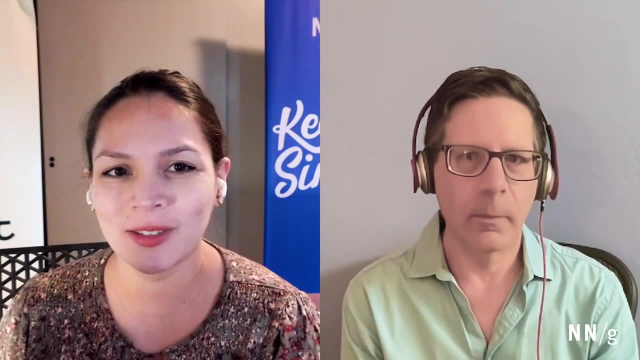 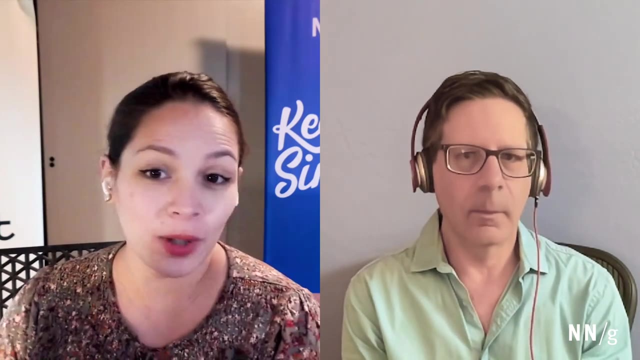 it was not the first method I had learned Um. a lot of the data gathering I did initially when I got into this field was surveys, And I mean, I guess that's tends to be a popular choice for people who work from, say, a marketing type of perspective. Um, and that was sort of what I did. 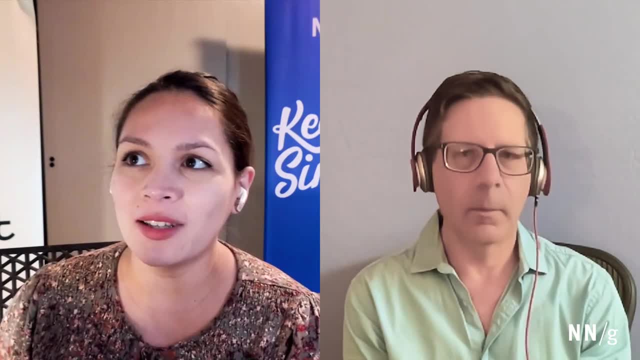 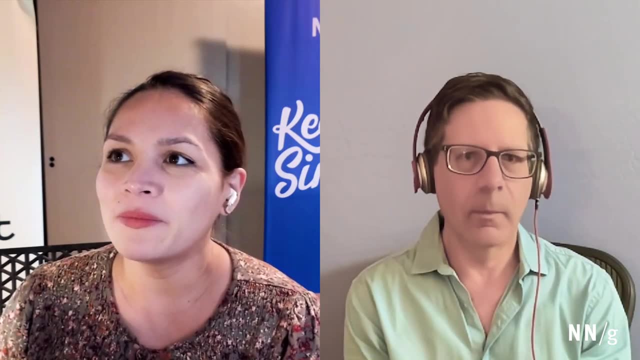 a lot of my undergraduate classwork in, So it was sort of the natural thing that I turned to when I thought, hey, I want feedback from people, Let me blast out a survey. Um, and granted, there was a time and place for surveys. I'm not trying to badmouth them, I think they're. they're certainly. 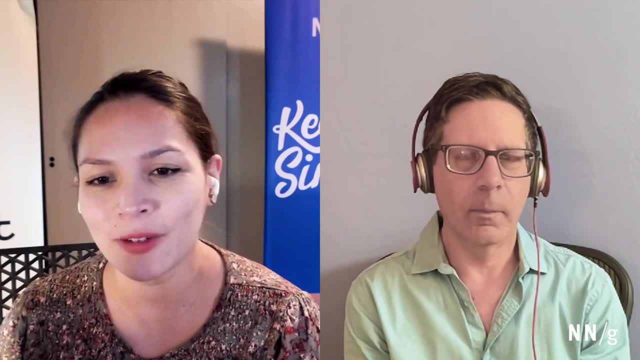 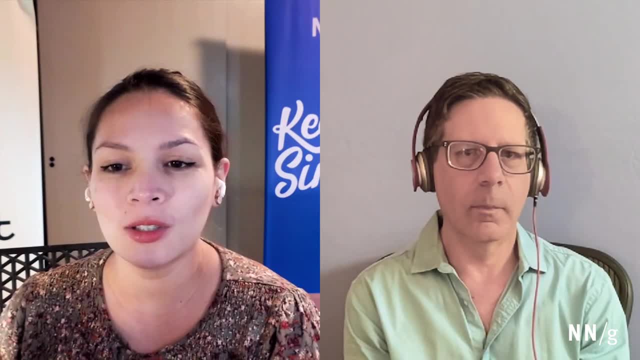 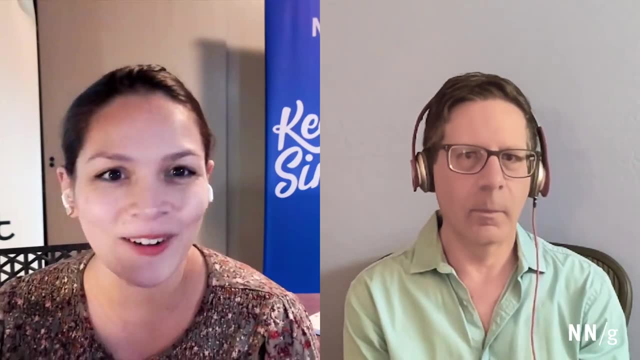 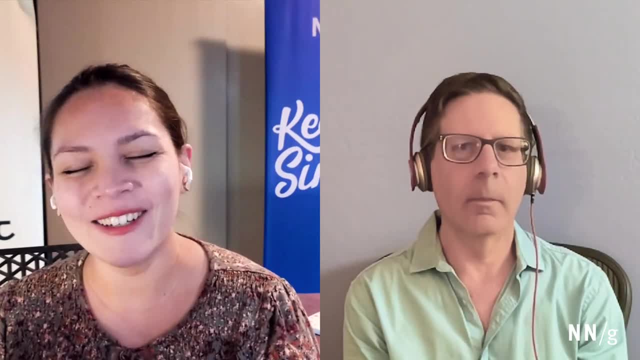 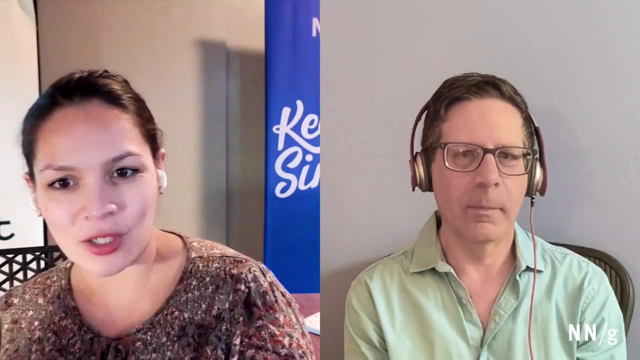 kind of feels like a meta moment because I'm facilitating an interview right now. Uh, but there's, you know, there's a lot to consider, like body language. There's a lot to consider about how you ask your questions or how you probe about a particular topic. Why would someone intentionally 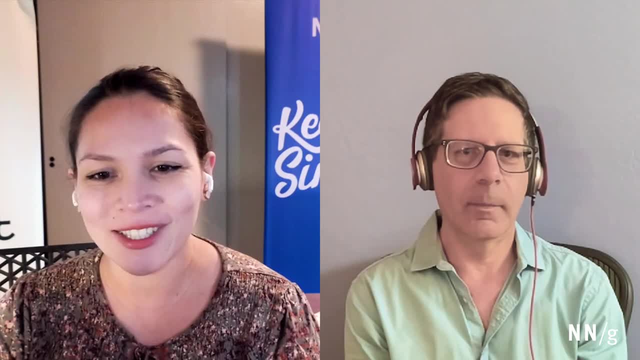 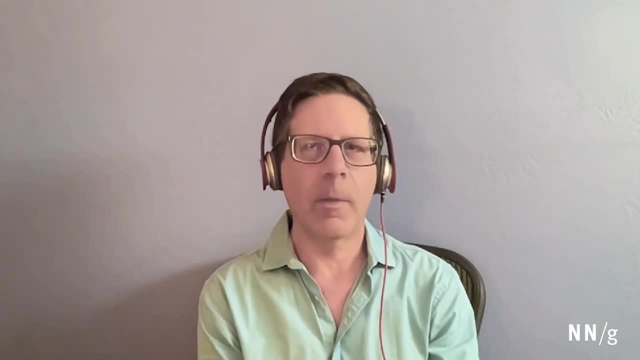 choose this method that also takes longer and costs more, versus blasting out a survey, which is obviously going to be a bit less involved. right, I mean both surveys and interviews. look, they may look easy. It's just having a conversation, It's just. 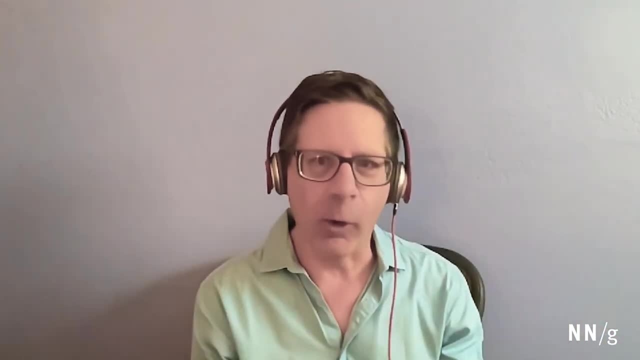 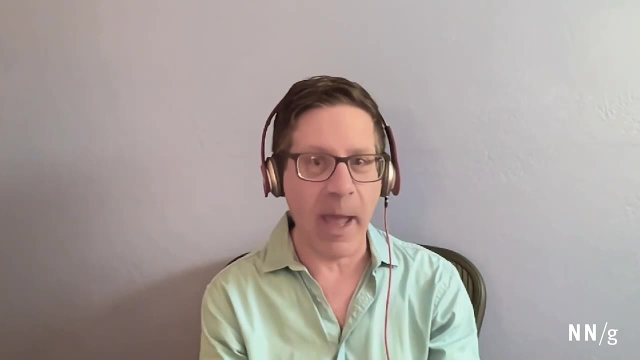 typing up a bunch of questions into, uh, whatever a Google form or whatever platform, And I think they both are deceptive that way because they're. they take a lot of thought and intention and and practice to do well, Um, and I think you run the risk in both cases of 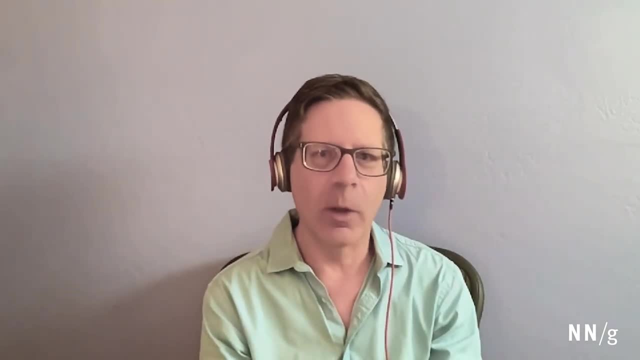 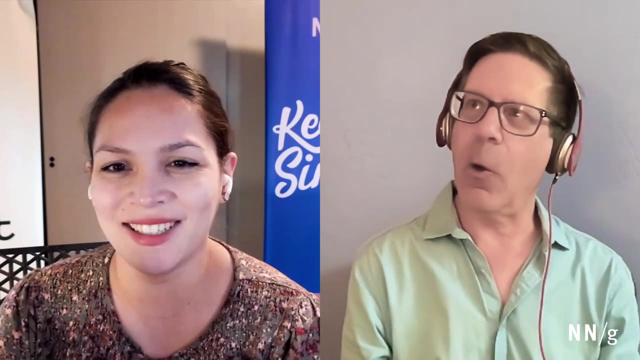 of, I guess, any kind of research. garbage in, garbage out. if you don't, you know craft your approach. Um, now you're a survey expert. You may disagree with me, So I'm going to go on a limb and 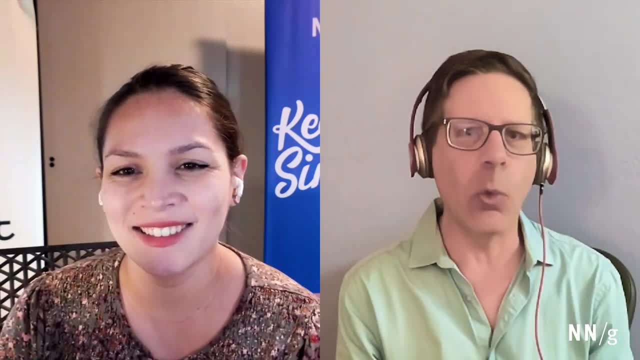 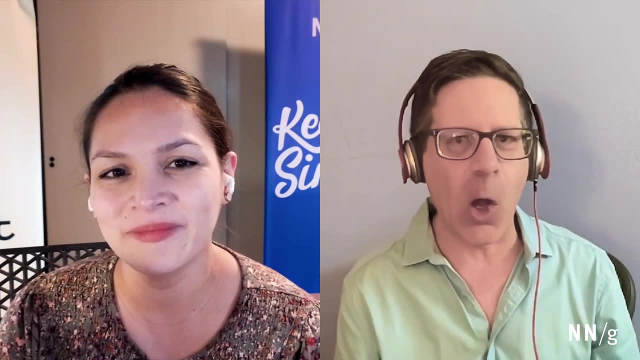 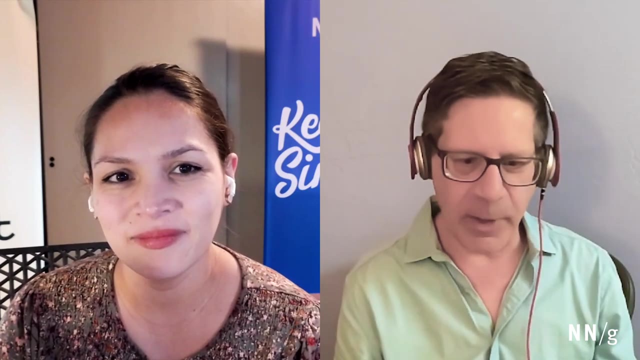 say. what a survey doesn't necessarily do is tell you why. Uh, but an interview can tell you why, because you have the opportunity to ask follow-up questions. So you might ask that same initial question: What's you know, what's the motivation? Well, I mean back up a little bit, even in a 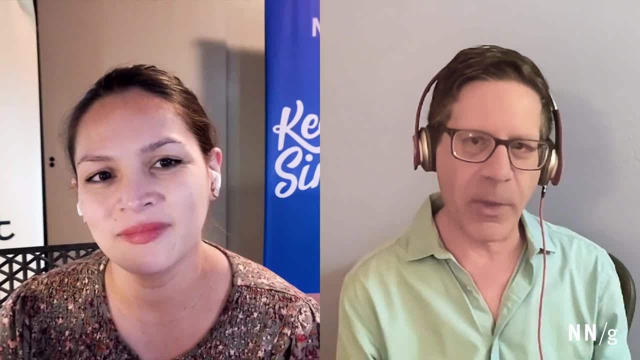 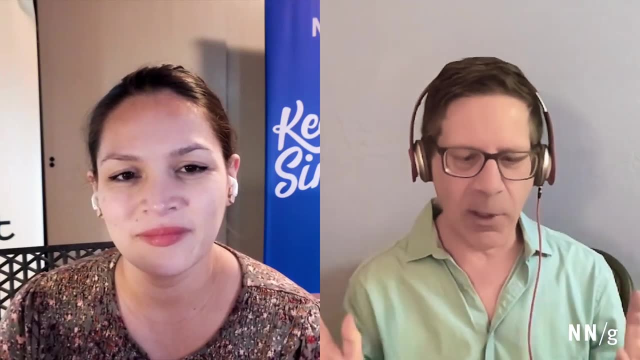 survey. um, you know, you might give people four choices of something or let them write in another example, but you might see some patterns or some groupings. but in an interview you might ask it in an open ended way, You might not say which of the four following is has kind of directed your 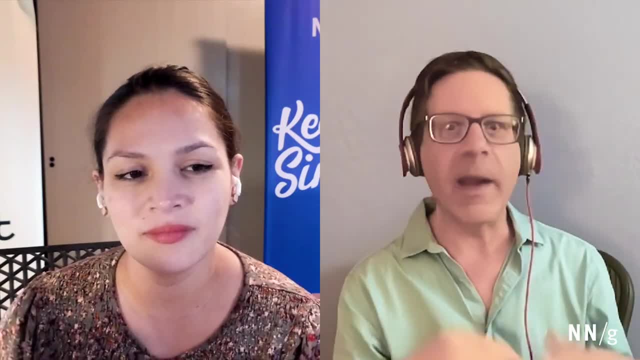 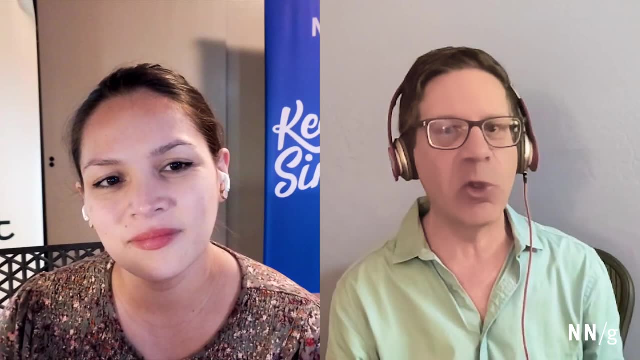 your reference or or your behavior, but what is it that kind of informs your choice? So you ask this open-ended question. Um, and so sometimes our questions have huge amounts of assumptions built into them about how people do things or how they think about. 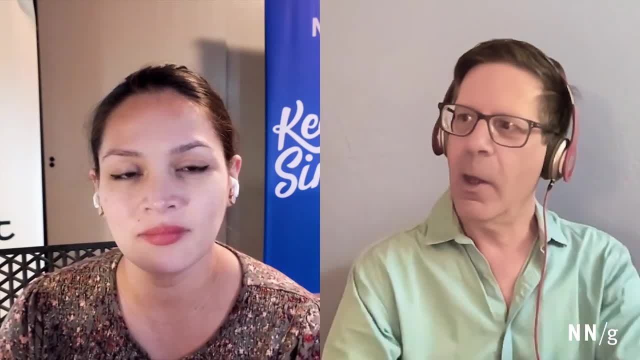 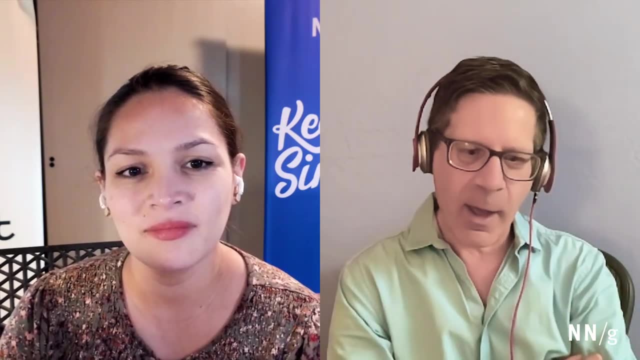 or what the choice is, or what actually comes before something else. So you can hear those moments in an interview. You can switch uh, switch direction and um, ask follow-ups, or let the person reframe the whole context of what we're even talking about And you can. 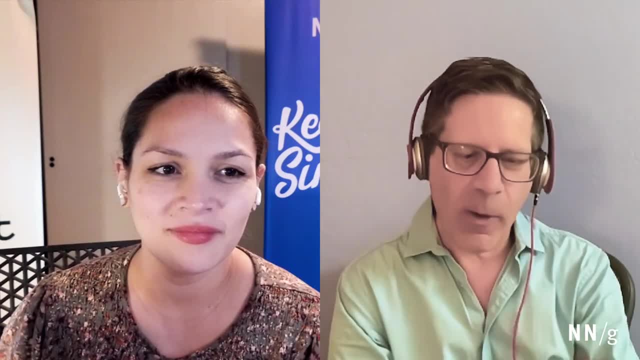 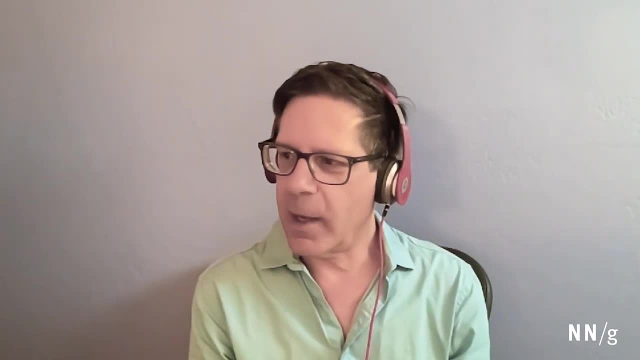 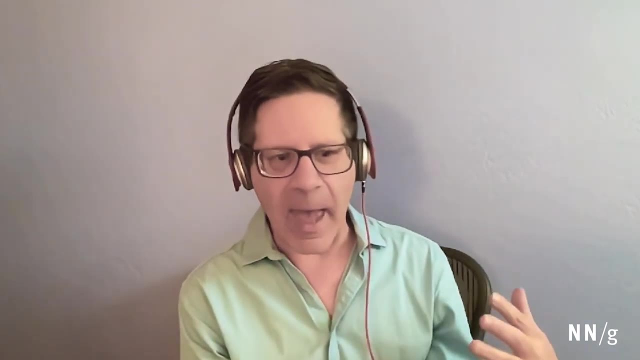 adapt on the fly, um, and ask more, and ask more, and ask more and kind of continue until you understand why. you know, one of the things I do like about interviews- and I kind of was getting at this a little bit- is that it's, it's a, it's a method that changes the researcher. 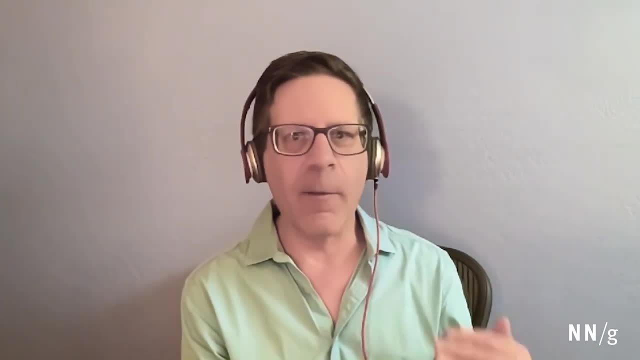 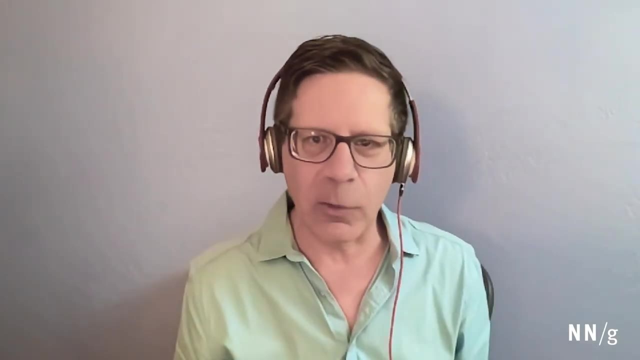 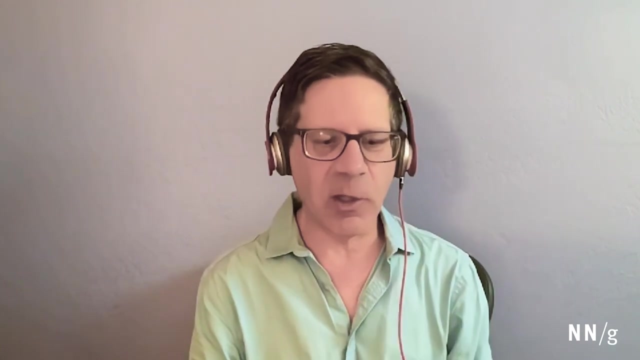 It changes their understanding of people, of the problem of the opportunity, And it does that in this experiential, kind of immersive way. If I'm going to talk to a number of people over the course of a week, um, you know, it's good, I'm going to be scratching my chin, uh, you know. 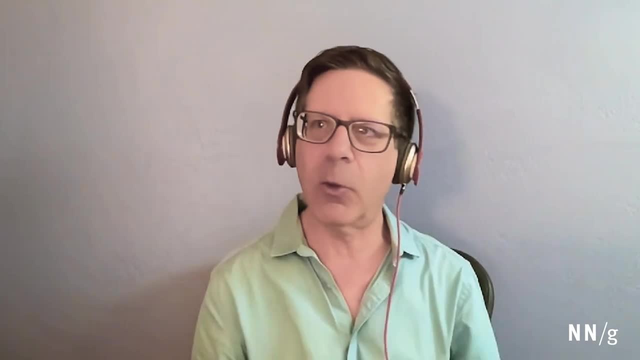 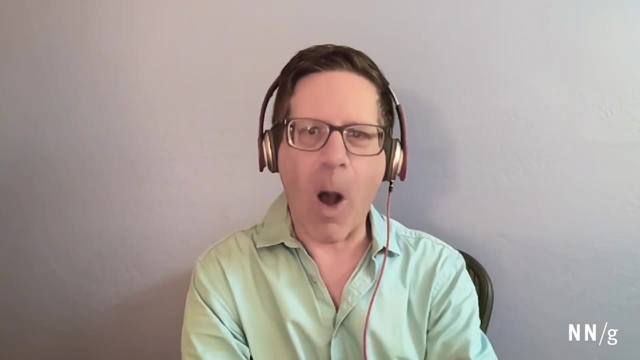 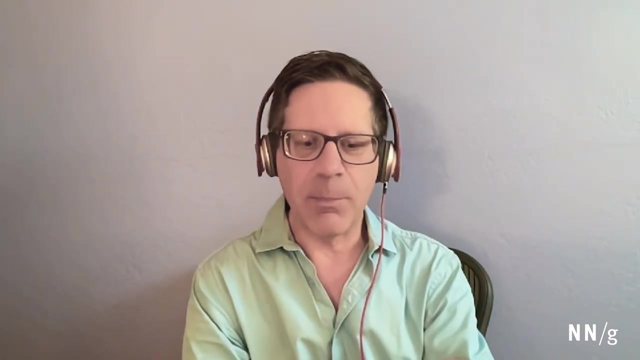 on the dog walk or thinking in the shower like it gives you a lot of experiential stuff, um to chew on, um the. the conclusions that you take are not obvious. They're not in the interview And it it it kind of. for me it's a very rewarding experience to kind of be pushed. 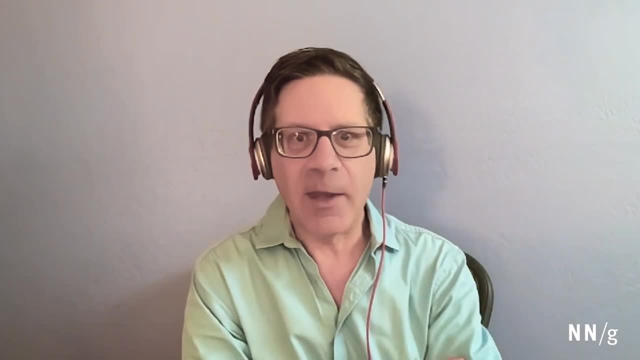 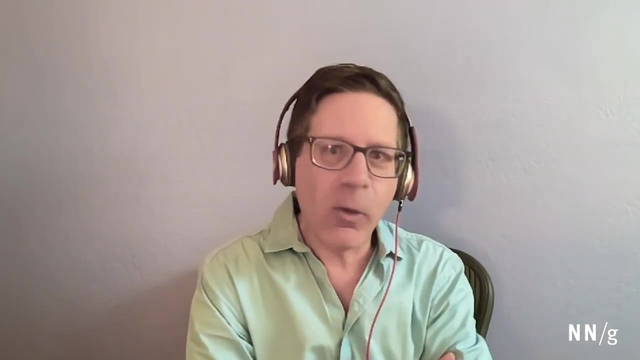 into this sort of sustained creative state, as you're thinking about. you know the people that you met and how they talked and how they, how they view their work and how they view their lives, because it it. even if it doesn't directly go there, it goes there indirectly. You. 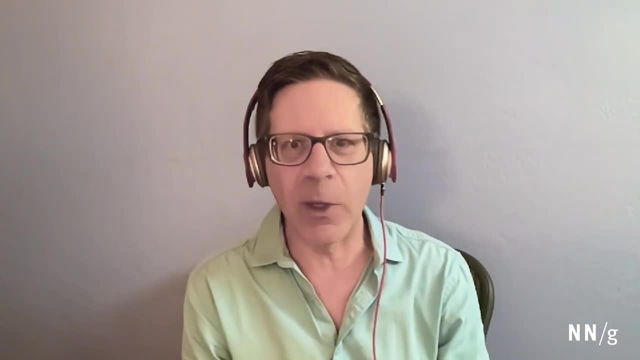 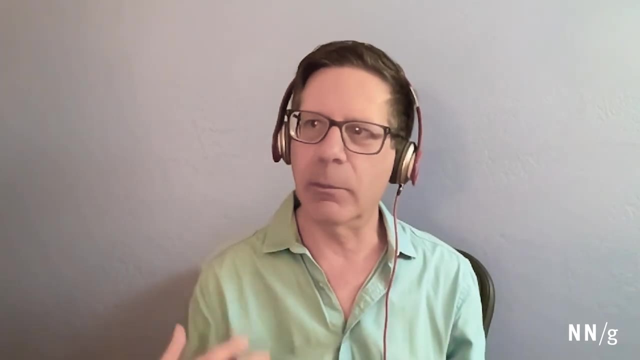 you start to see it, You start to understand something about other kinds of people. So it's really rich and rewarding, which you know is nice on its own, I guess, but it's um a really powerful way to stimulate. 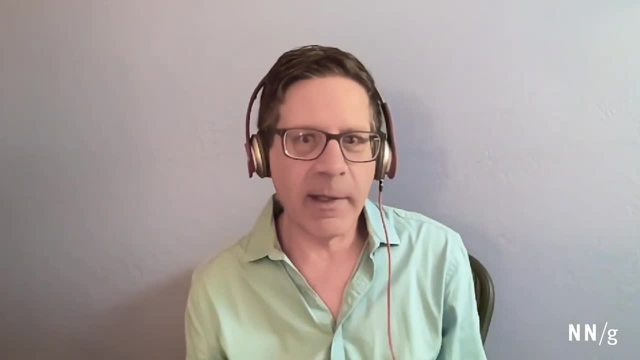 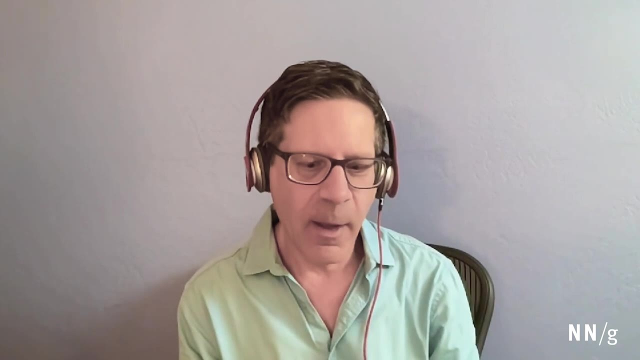 thinking about what it is that we're trying to answer. So I, you know, I get a lot out of it with the data and I get a lot out of it with the experience, And that um is different than other methods and, again, can compliment and be complimented by other methods because they 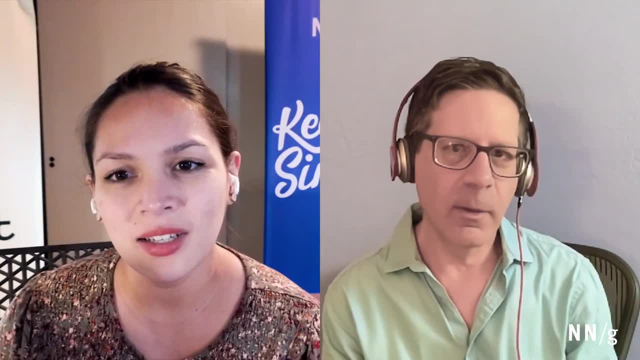 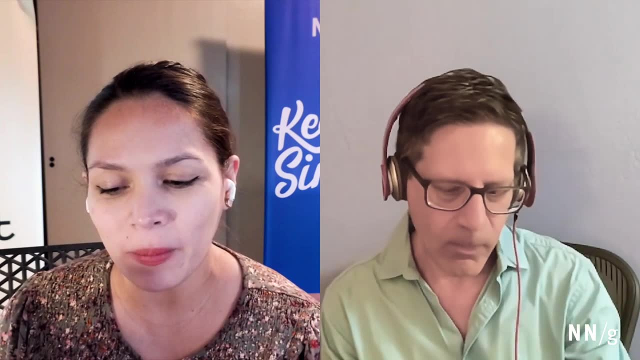 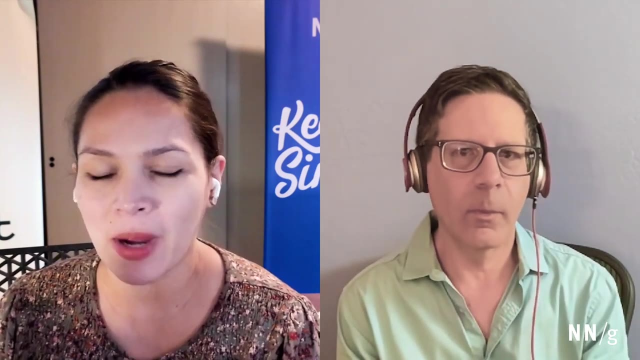 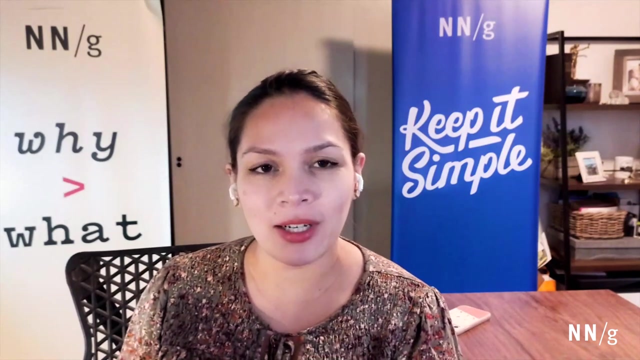 answer different kinds of questions. Absolutely, Um, I have to say, when I started running interviews, uh, the, the, the thought of experiential learning, like you're just saying is, was really powerful for me- And that sounds like a big word, like powerful, what? Uh, but it really was, because it was an opportunity to 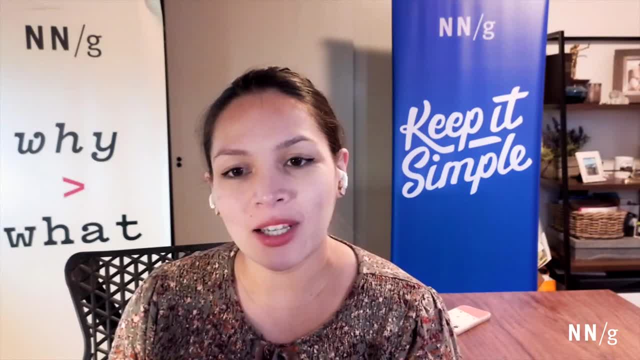 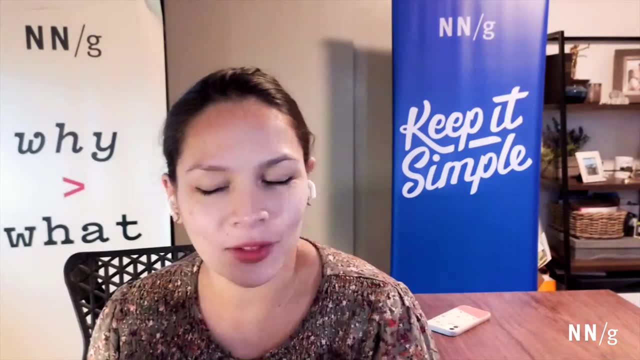 talk to another person and to connect with them in a very different way than you can in a survey. Uh, and part of that is, I mean, sure, In a survey I could certainly say why did you think that if someone choose, chooses some sort of satisfaction rating, fine, but the likelihood that I'm going to get 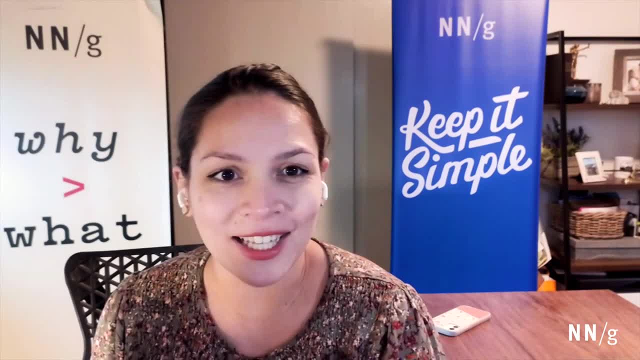 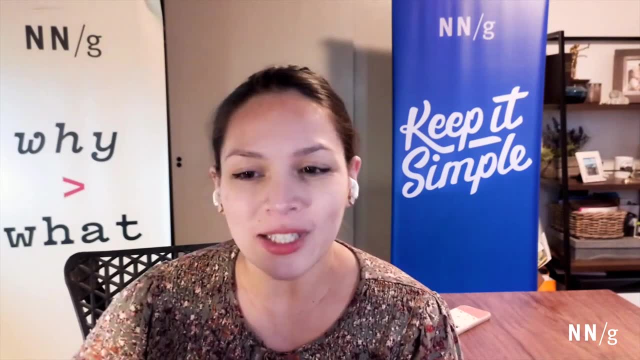 any more than maybe a sentence or a couple sentences. it's pretty low right. It's usually going to be some sort of short, stunted statement, And if someone's really angry maybe they'll write a little bit more, but I'm still not going to necessarily get the nuance. 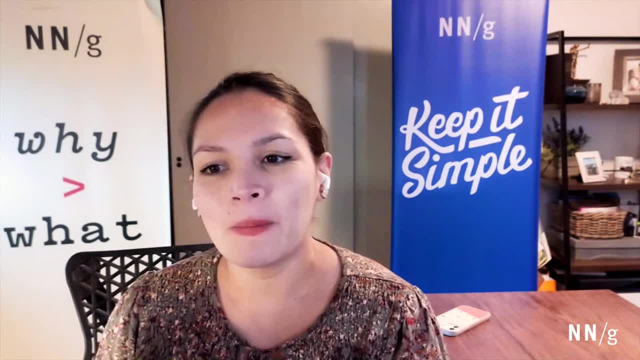 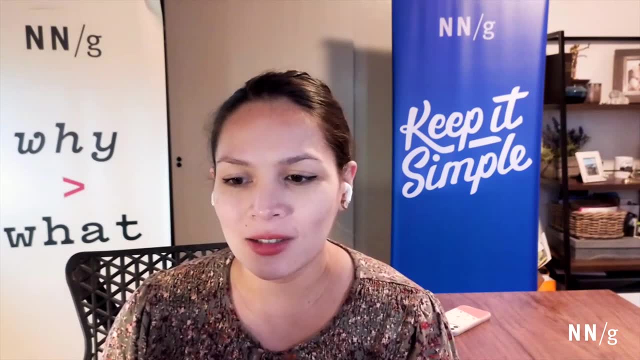 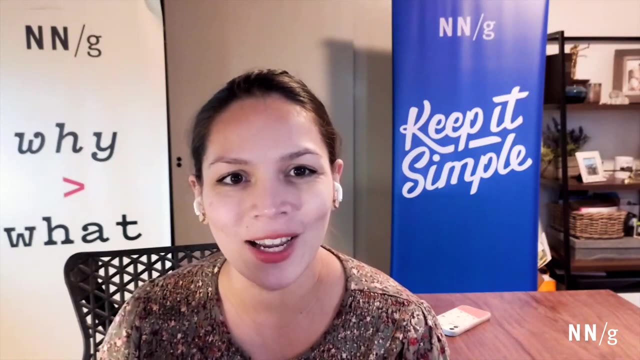 of what someone has really experienced And, um, I think that being able to talk to someone is going to give you so much richer data. Uh, you, you can connect emotional sentiment and even some of the more complicated emotional sentiments and maybe people won't be talking about or think is worth talking about in a survey. 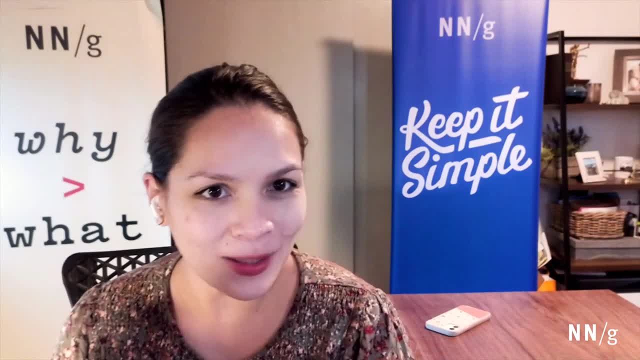 Um, and and to your point. you can also drill a little bit deeper, ask questions like: well, what, what about this particular topic? Let's, let's explore that a little bit more, like, like you were saying, the survey, when it goes out, it goes out. 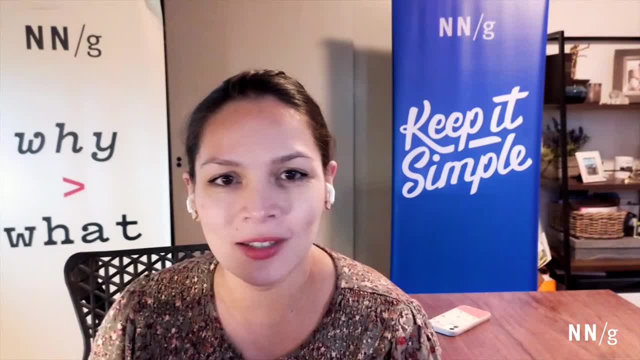 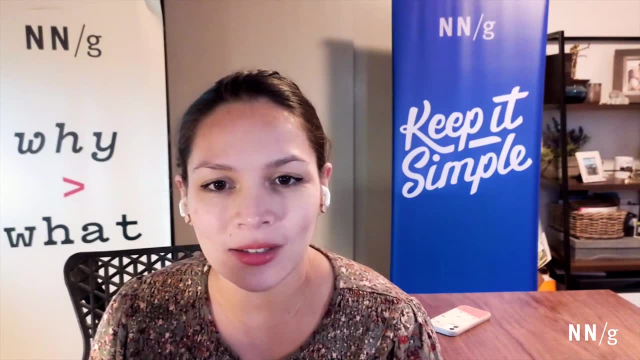 And there's no interesting comment from the other person. ask for it from this person here. let's follow up with them. I mean you might be able to try, but the likelihood that you'll have any sustained conversation after that is low, if not none. 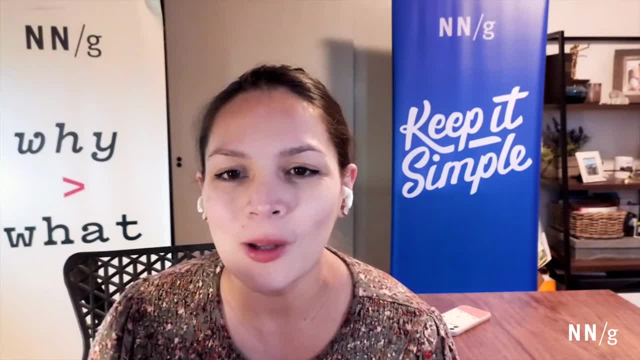 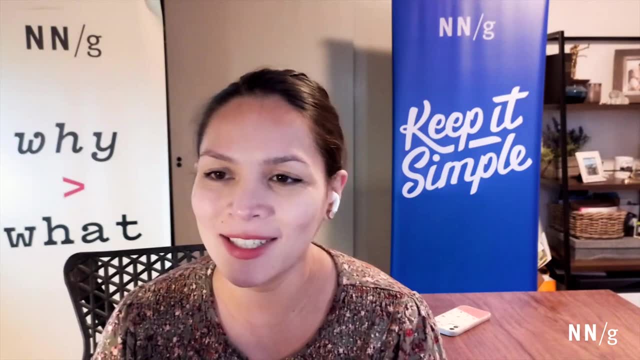 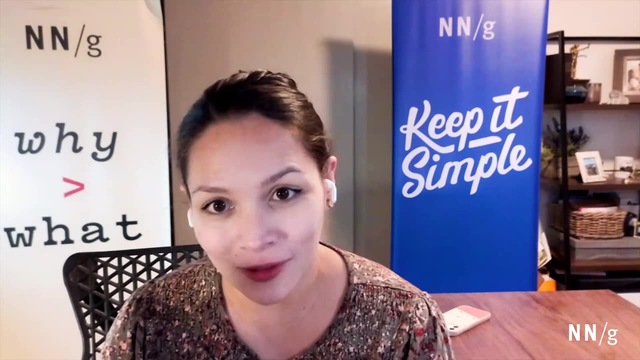 So I do think that interviews have this value that is sometimes undervalued, in the sense that surveys can sometimes be a bit overprioritized or seen as kind of the easy button solution to getting user feedback. So, yes, while I do still use surveys occasionally, I usually treat them a. 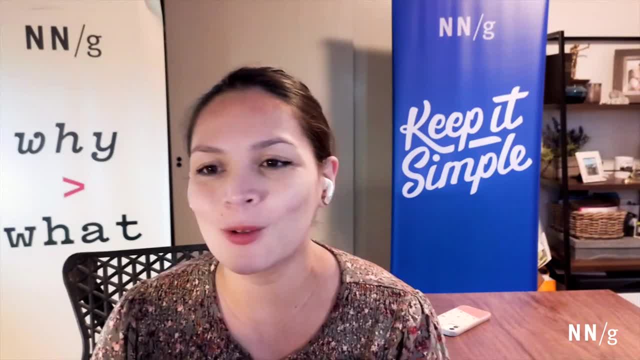 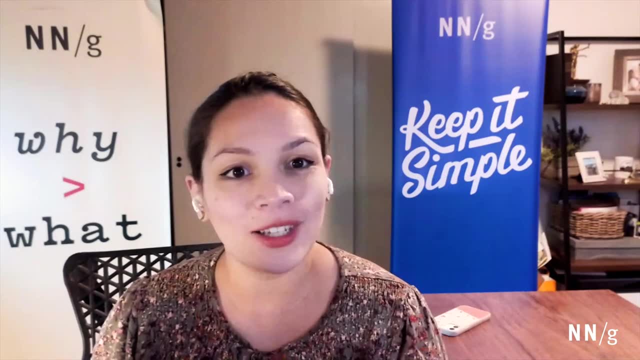 bit differently, or I don't rely on them purely as the main source of user feedback And I kind of acknowledge that, hey, there might be other methods that could be beneficial here, Like maybe an interview would help supplement and add a little bit more context than 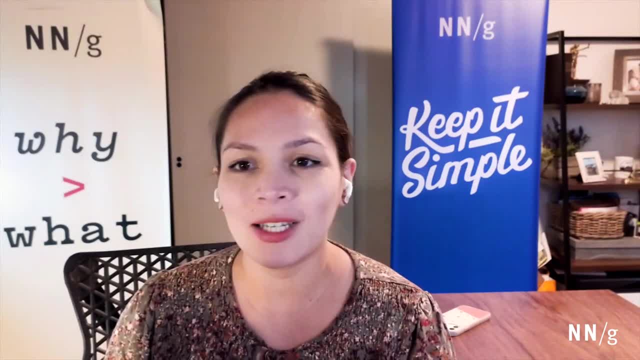 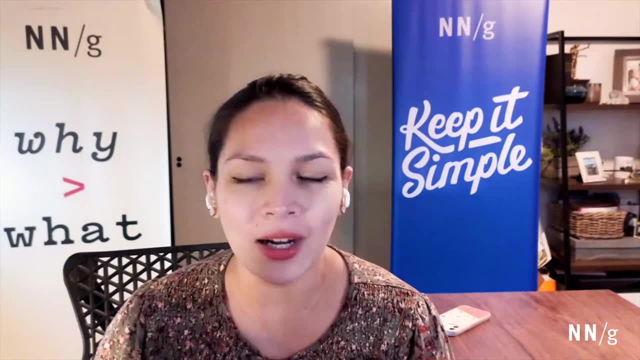 the survey is currently getting me, Or maybe the survey is going to be a good starting point, whereas the interview is where I focus on maybe some really specific questions that maybe I want to dig deeper on. So I totally agree with that. I guess to your point. you are kind of related to what you said earlier. 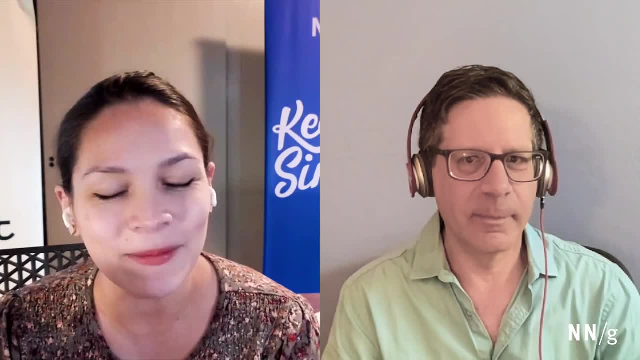 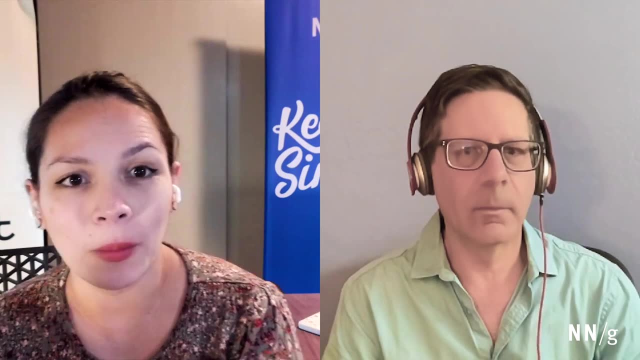 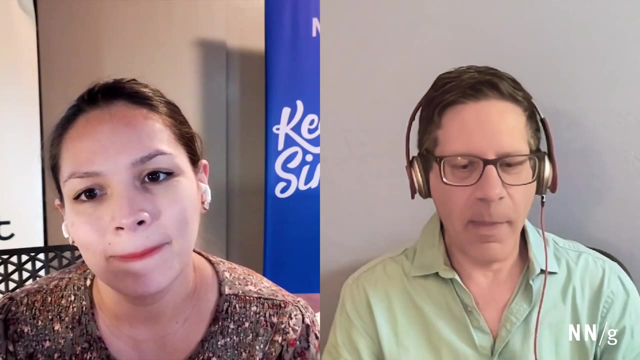 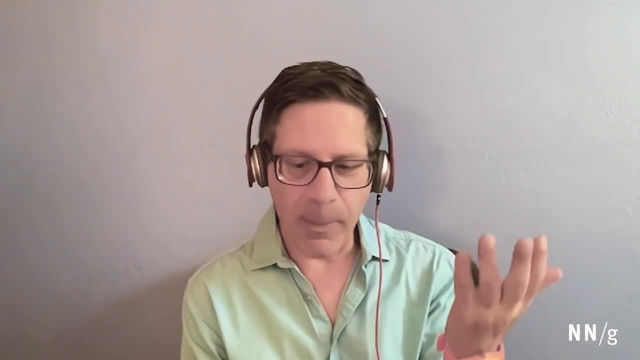 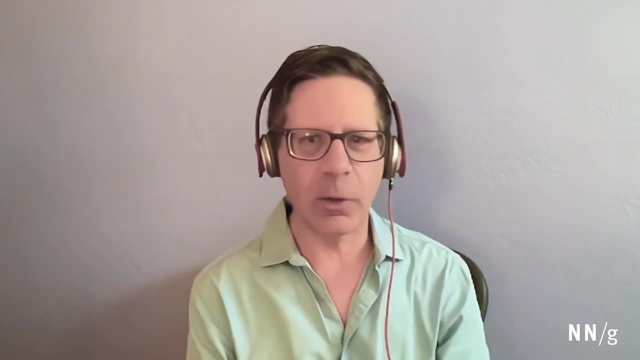 of methods that we can use, And I think there are a lot of methods that we can use And I think we make up new methods all the time. This is a great topic that you all have actually published, I think, the classic article on this by Christian Rohr. It's, I think, When to Choose Which User. 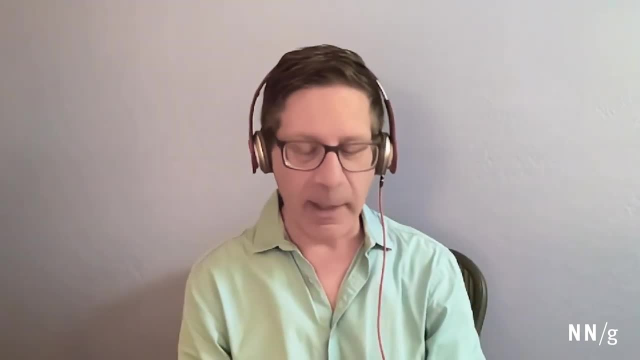 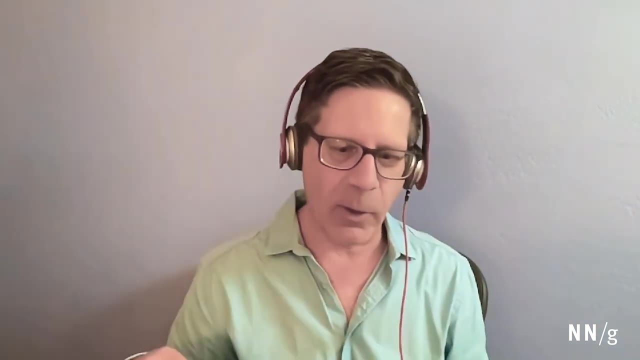 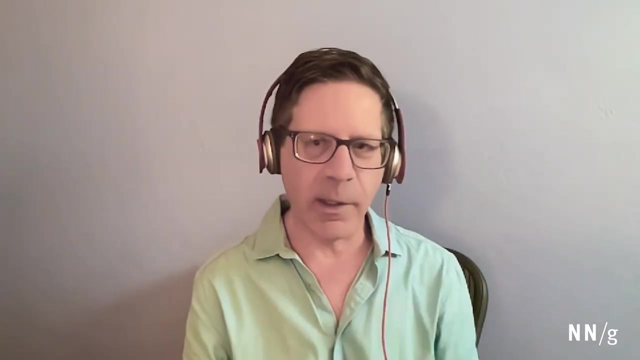 Experience Research Method. I might not have the title exactly right, but it's a classic. Everyone cites this all the time And he does a great job of kind of laying out different methods and what kinds of questions they answer. So one example is: let's say we wanted to understand 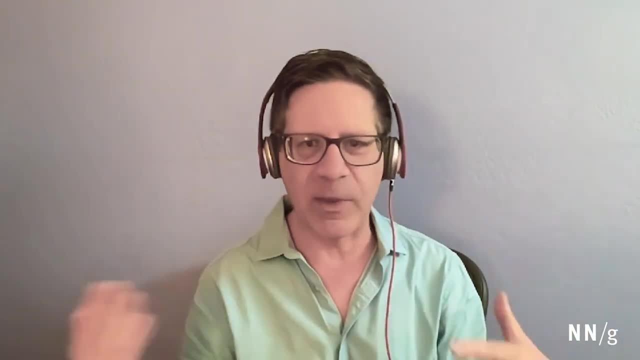 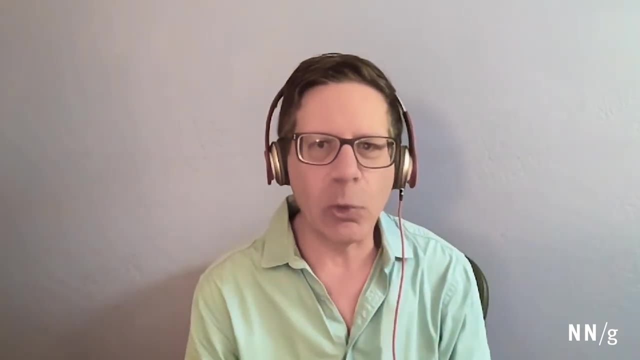 there's two different navigational paths on a website to kind of complete some task, And we want to understand, I don't know which one people would choose or which one if people go down those paths. which one do people get further down? Let's say we want them to. 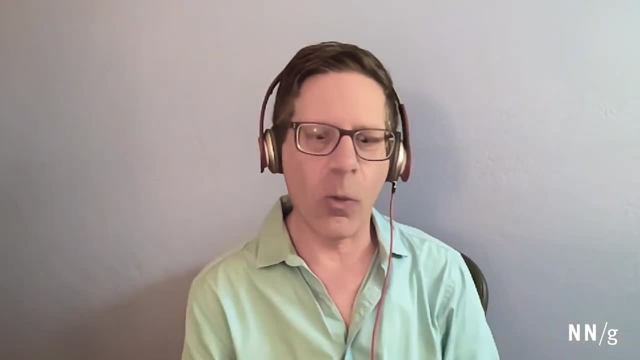 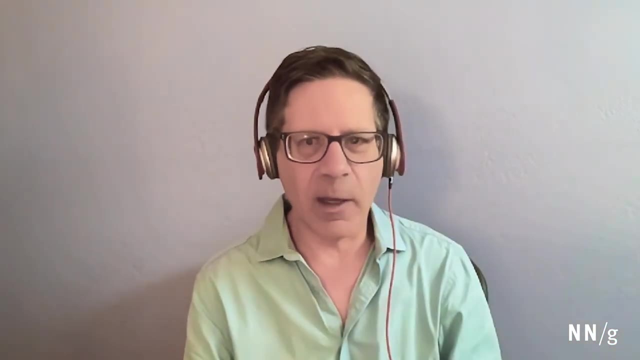 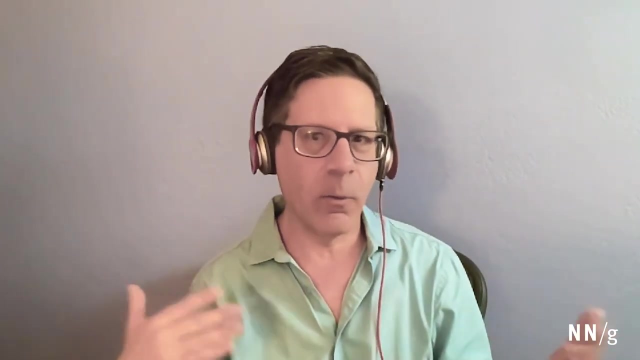 complete something like make a purchase or register, So you know path A versus path B, which leads to more success. Well, that's not something you can do in an interview, But it's something you can do like in an A-B test. So you put those up and people are randomly. 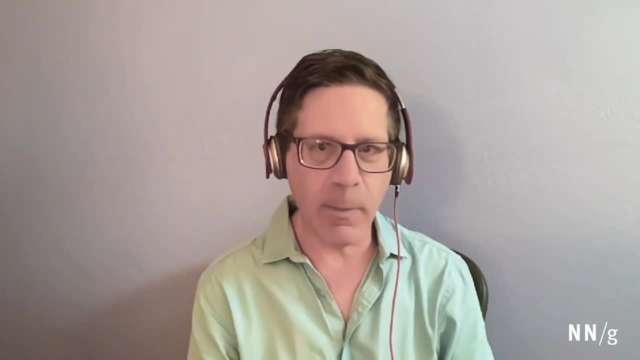 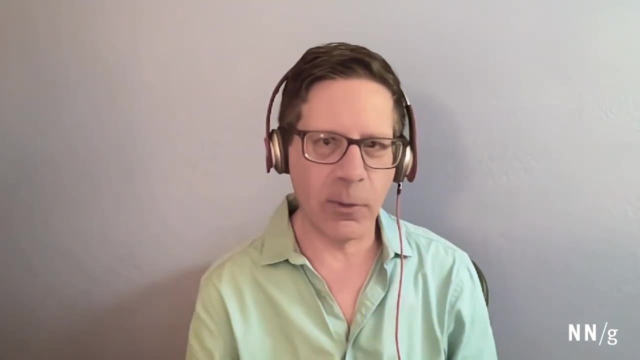 sampled on your site and they're directed towards something And you can. maybe, depending on your site and your traffic, you might be able to get a lot of data very quickly about two different design choices or two different kind of implementation choices. Again, you don't. 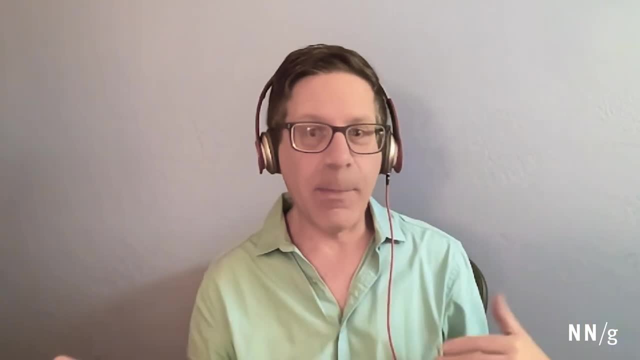 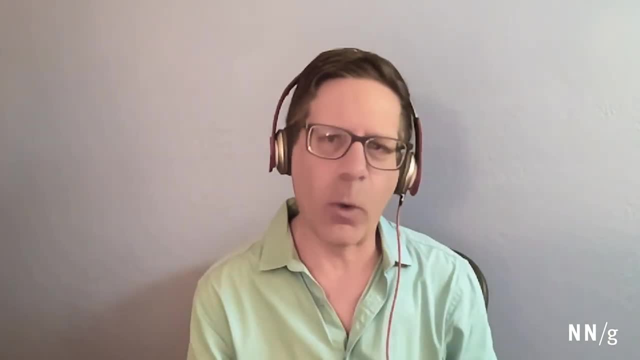 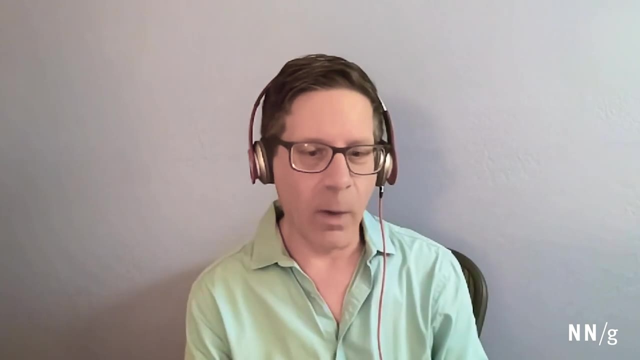 giant explorations and you have two different ideas and you just want to see which one works better. You know, I think you put it really well, right, We could combine different methods and we could if we needed to understand why. we wanted to dig deeper into, like what is, what's the? 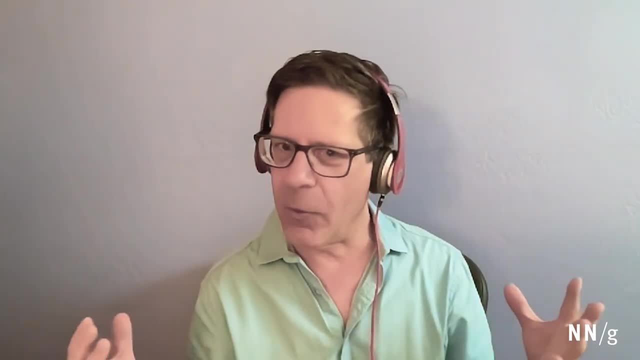 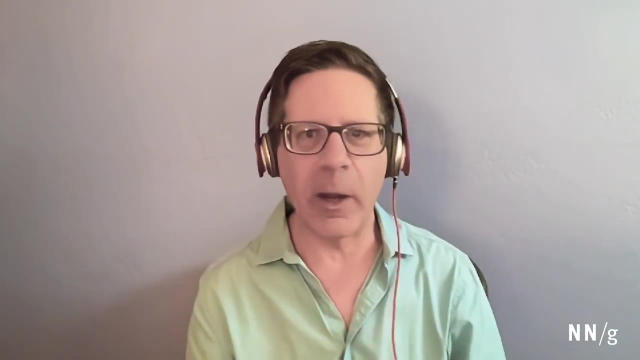 objective in going down this path, or what's the mental model about how this site is structured or what's the anticipated reward at the end of this path. we might want to do an interview. We might want to sit with someone and have them go through this path and choose A versus B or show. 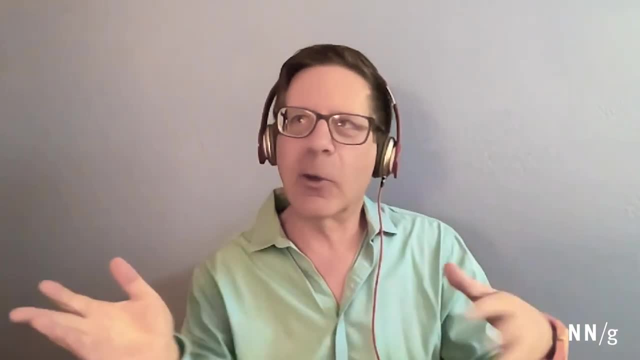 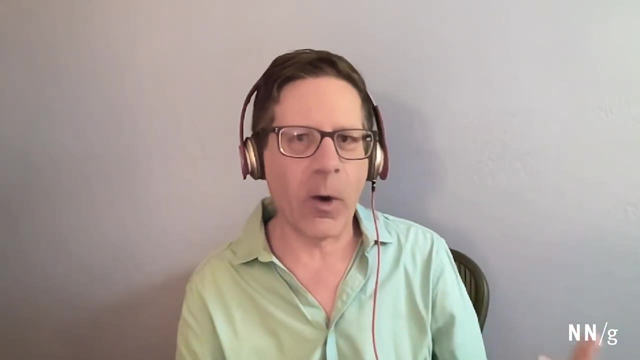 them A and show them B. Is that a usability test or interview? It goes back to your initial question. I don't know. It's sort of using interviewing to ask why. but if that's not our question, if our question is sort of which one or what, or sort of even how, then we would sort of run an. 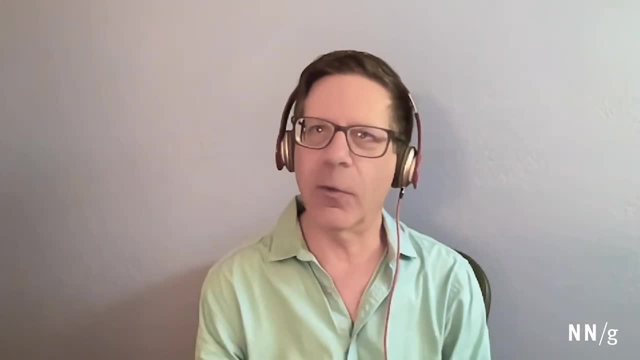 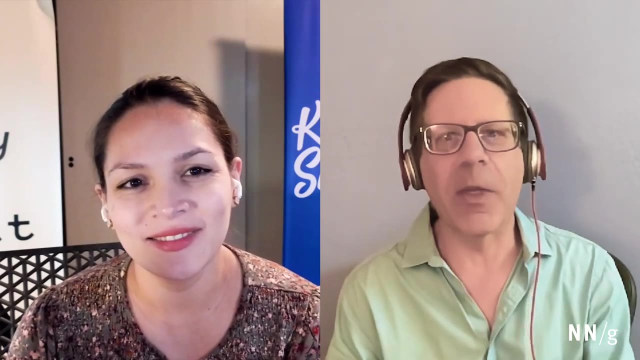 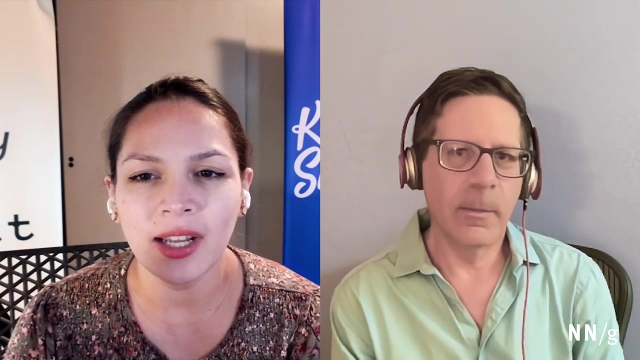 experiment or put these things in front of people and kind of track that. That's a very different kind of initial question than the one with an interview. But that's a scenario, I think, where you wouldn't use an interview initially, You would use an A-B test to get that answer Right. Right And I think, yeah, there's. 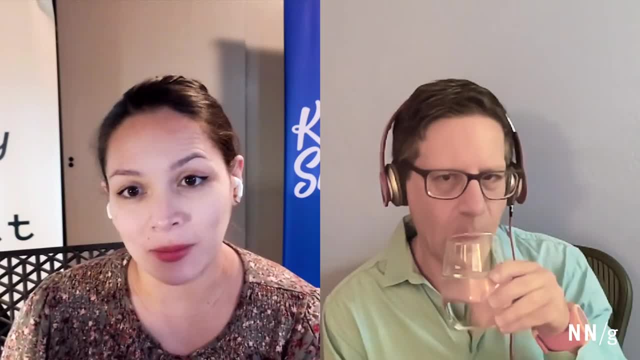 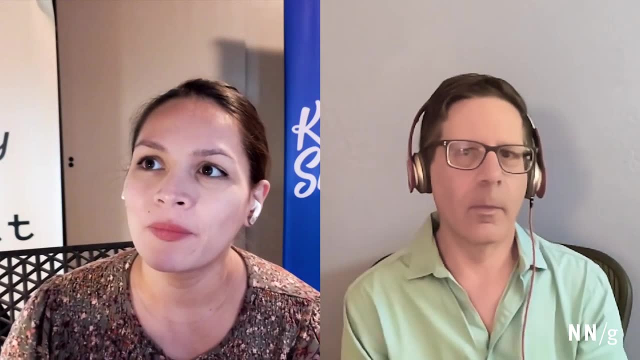 obviously going to be certain things that you might not be able to ask somebody because it just simply is too fraught with challenges. Like, what comes to mind is: maybe we ask someone what is the process you take when buying a house? And, like, certainly someone can. 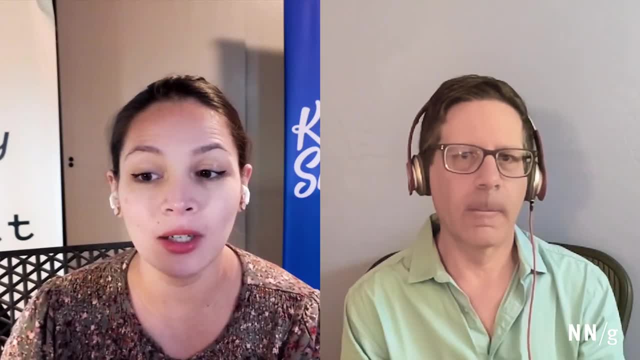 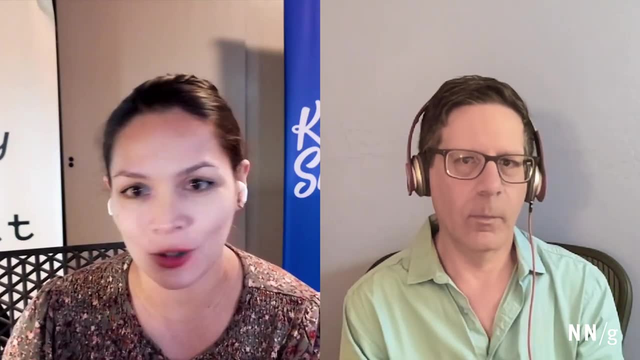 like talk From memory about the time they bought their house and maybe they give a lot of detail but there still might be missing pieces. that not because someone's being malicious or withholding information, but maybe they just didn't think it was worth talking about or forgot about it. 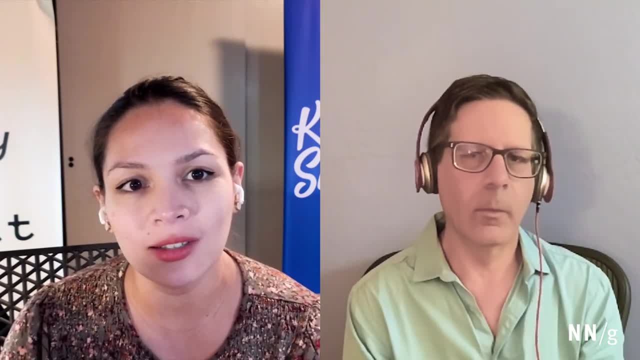 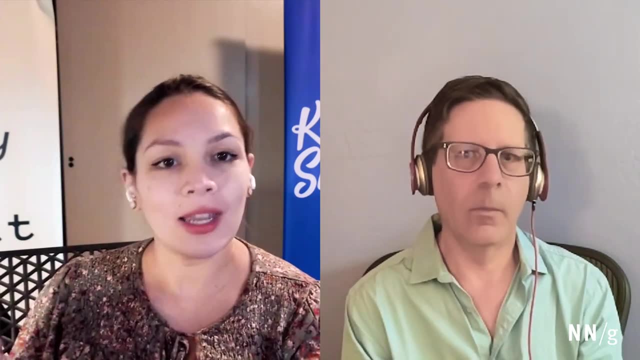 And- and I think that's one of the challenges with interviews as well as like, maybe, some form of observational data, or if we were to say combined with like a diary study, where someone is tracking what they're doing over a longer period of time, then then these methods might be. 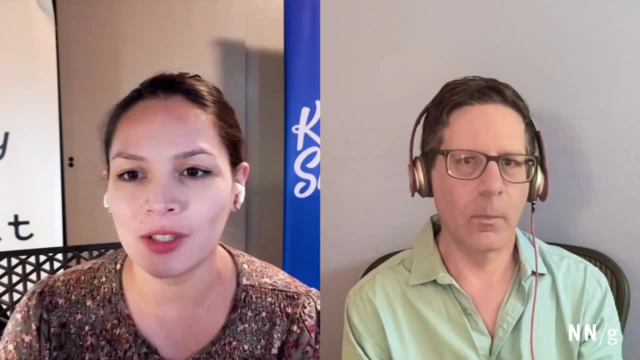 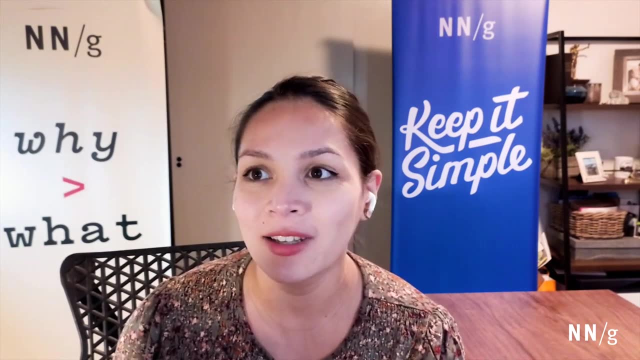 helpful to complement where an interview, which as much as I would love to talk to people all day long, there's kind of a time limit to it. Another thing that comes to mind is maybe an impractical scenario to observe Like um, they're probably going to be some parents on this listening to. 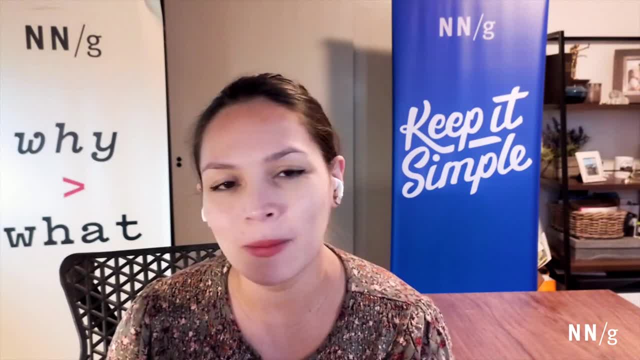 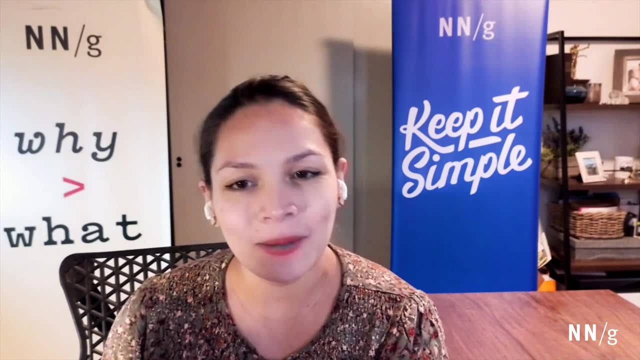 this podcast. who would say, yeah, if we were studying something? like a baby waking up at three in the morning, is it really practical for a researcher to be present and observing that? possibly, but maybe that's not something people have the budget for. 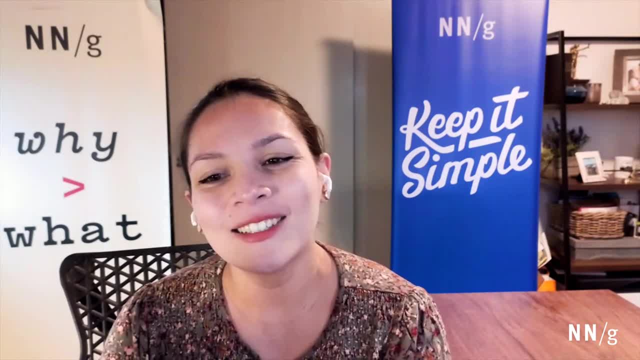 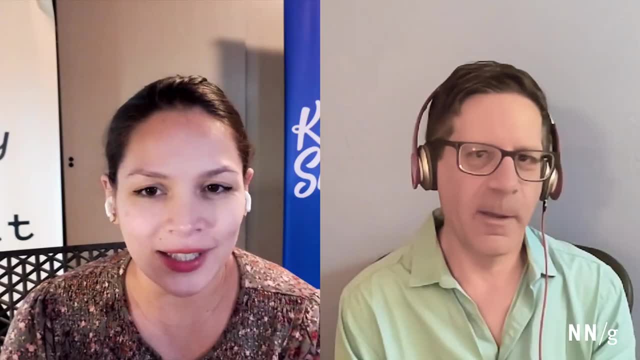 Invasion of privacy. you know, it might not be that interesting, So that's where that interview can obviously fill the gap of perhaps something that's really hard to observe as well. Obviously, this is a topic you're very passionate about and there's opportunities to interview users. 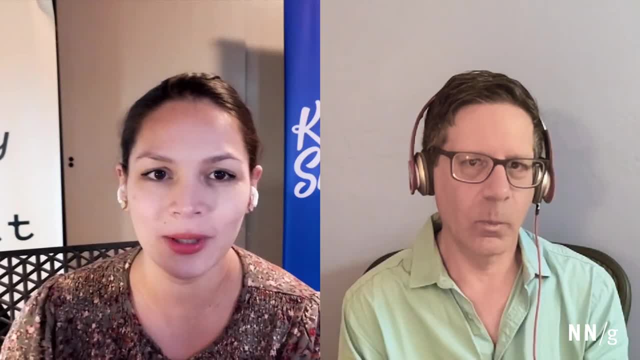 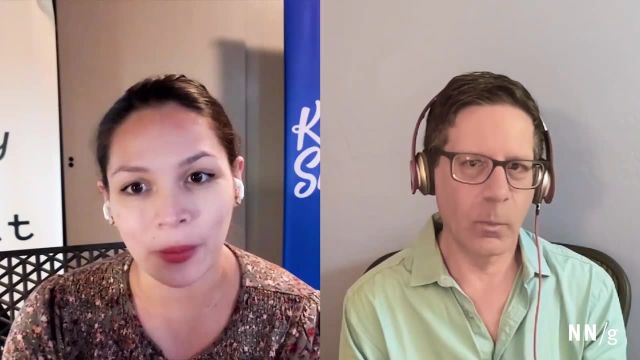 not just as its own standalone method, but even within other methods like usability tests or field studies, And it's a topic that you're passionate about so much that you not only wrote a book, but you've also- had you know- created this. 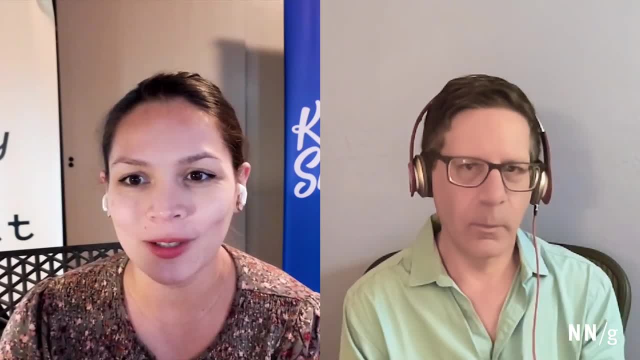 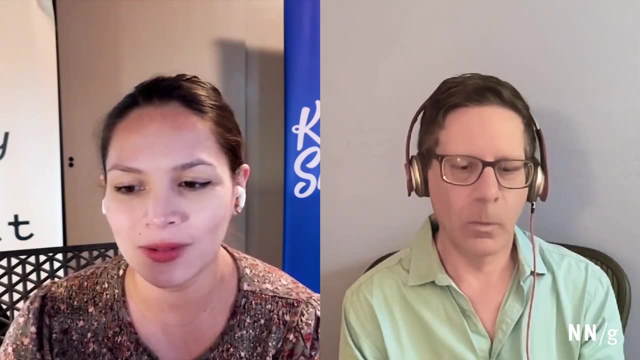 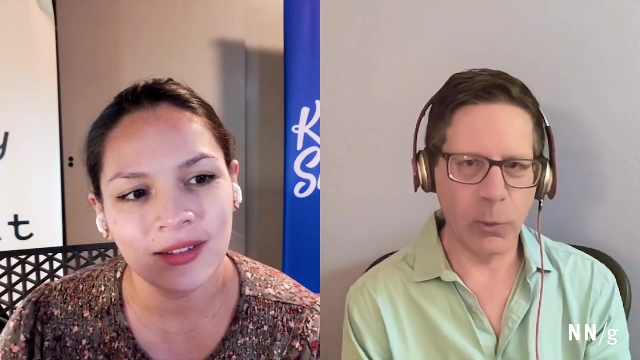 second edition, 10 years after the publishing of your first edition interviewing users. What would you say has changed over the past 10 years? when it comes to interviewing users- And I think the the context in which we do research- I mean of any method, but certainly 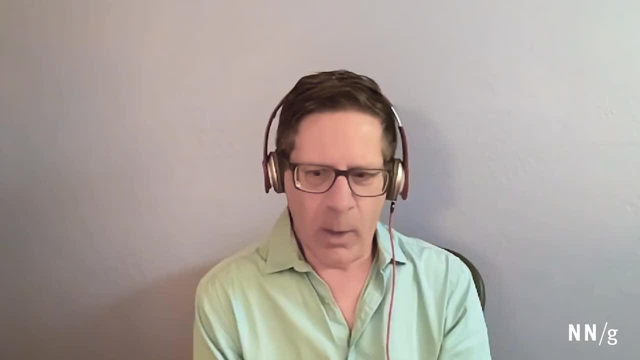 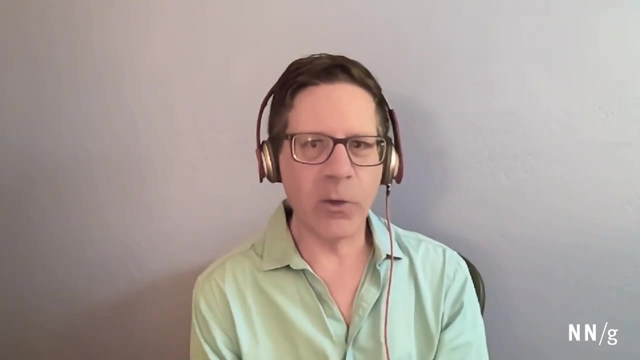 interviewing um has has changed in 10 years. You know we've seen a lot more organizations building up teams, but we've seen a lot more organizations building up teams. but we've seen a of user researchers that you know are doing interviews Um, we've seen a lot more people. 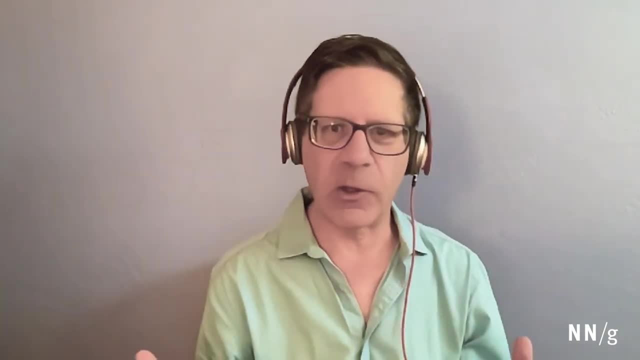 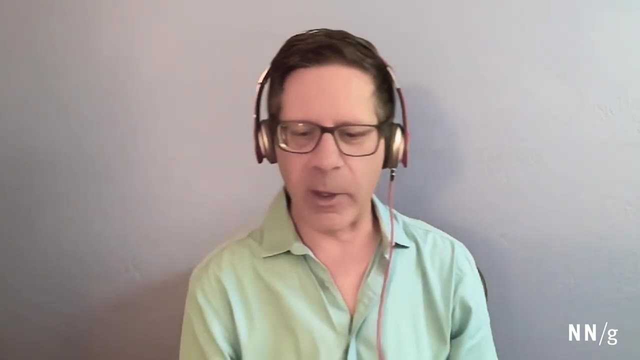 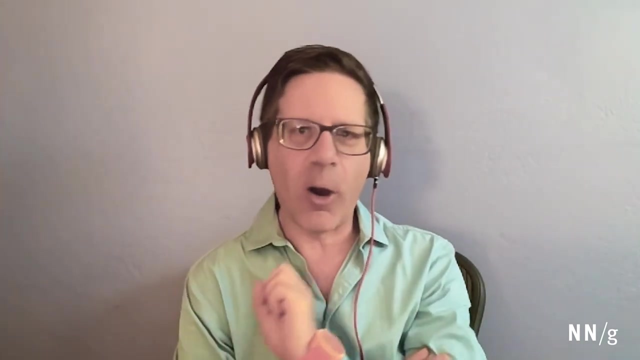 inside organizations and the the term. Kate Tousey has this great term. She calls them people who do research, PWDR, And so she, uh, is a writer about research operations and a leader and teacher in that field And she talks about: you've got researchers and you've got PWDR, And that. 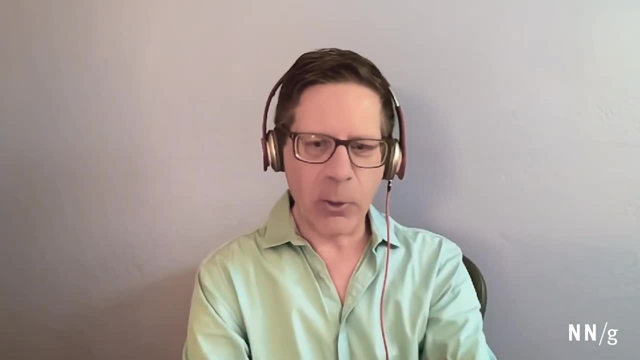 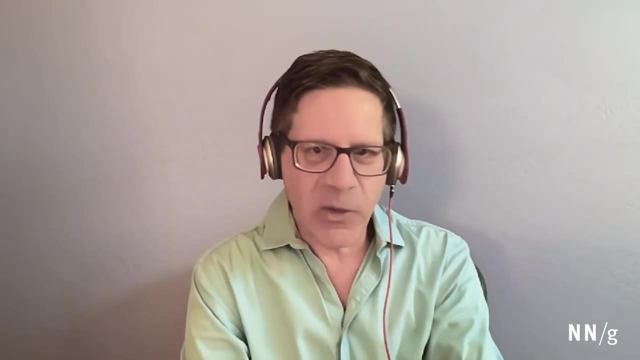 framework I think is really helpful because, you know, we've been sort of struggling- I think collectively, as a field over like to ask ourselves like well, who does this work? Is this people with titles? Is this consultants or vendors or partners? Is this- um, you know? 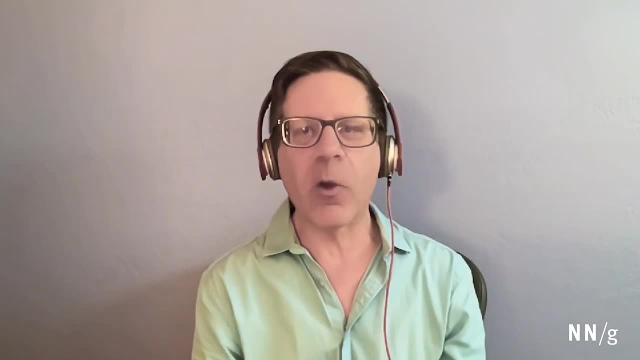 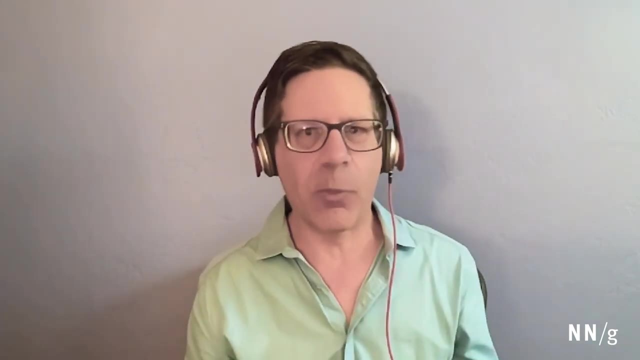 whatever you go across your organization- And I think it's it's still an open question, but it's it's shifted over 10 years- You have you have fewer consultants and external practitioners, you have more internal practitioners, Um, and so you have with that that we've also seen. 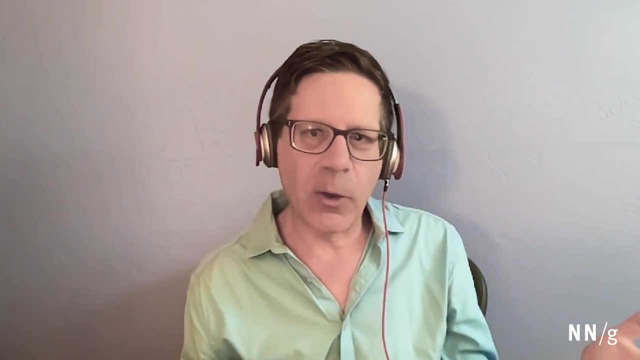 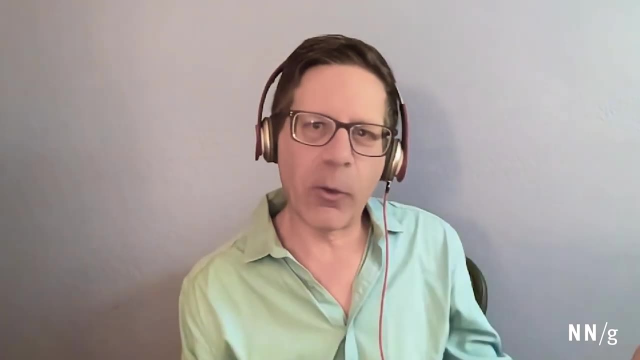 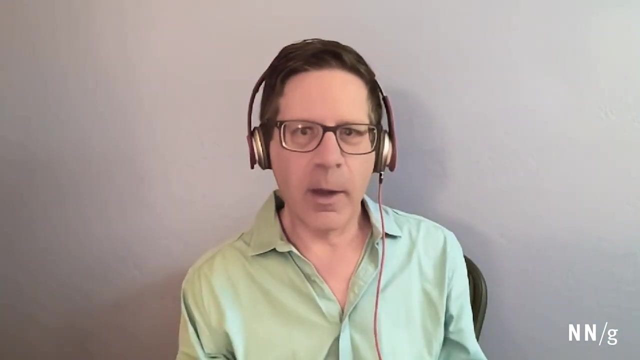 you have leadership. So I think you could go back a number of years and a company may have a researcher on staff, uh, but they maybe didn't, they reported into some other organizations, So kind of the maturity of research as an in-house function. So you have, you know, you have career ladders. 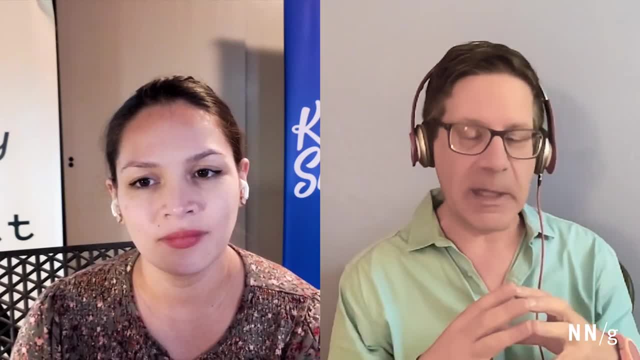 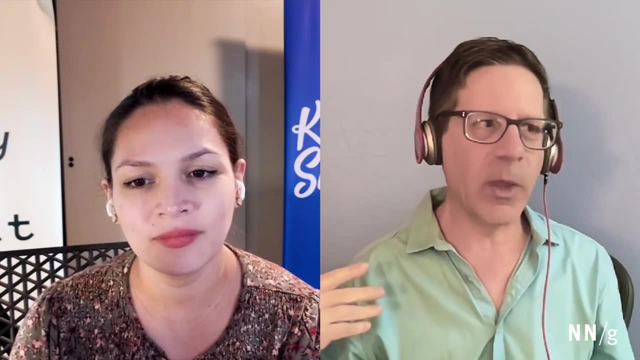 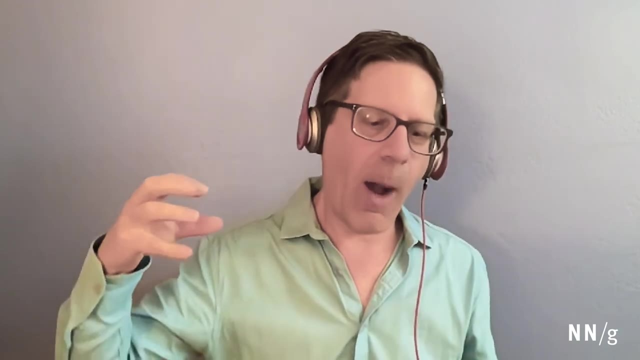 you have ways to progress and, um, you have teams with different methods kind of brought together. Um, and this I mentioned research operations. This was not really a term that got used very much. I don't think it was used at all 10 years ago. this idea that, um, you know the operational, 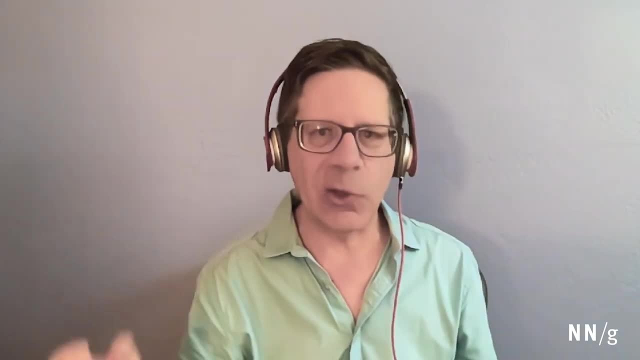 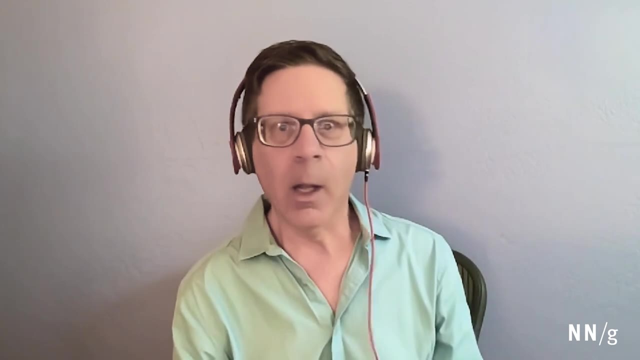 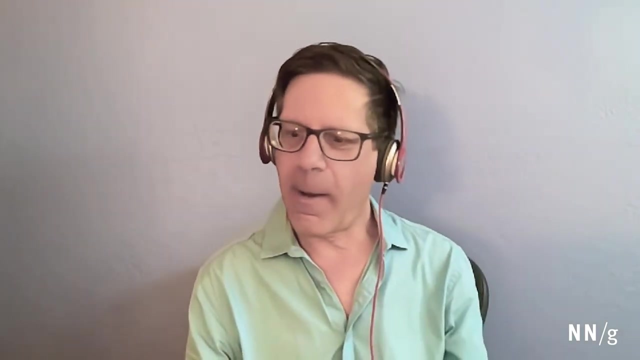 support to make an organization ready to effectively perform research. So there's lots of there's lots of tactical aspects, logistical aspects, legal compliance aspects, which we really didn't talk about. So we kind of tried to avoid maybe 10 years ago. um, that have you know, legislation has. 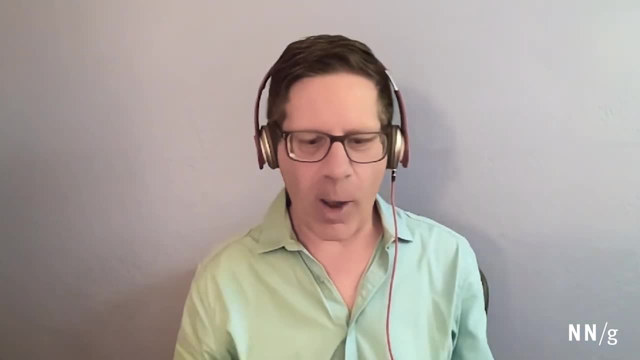 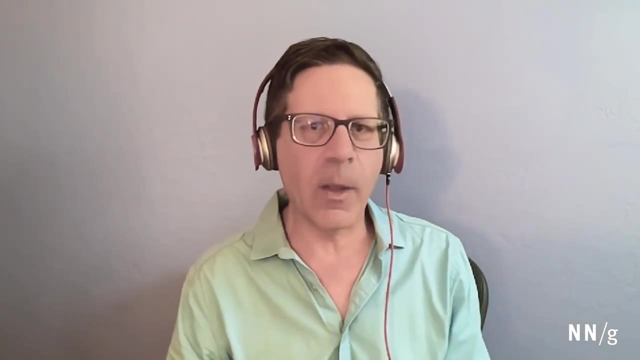 gotten more serious. the consequences there are. Um, you know there are. I know I have colleagues who have, uh, who are research leaders, and they have a partner in the legal department of their organization And that person is set up to. 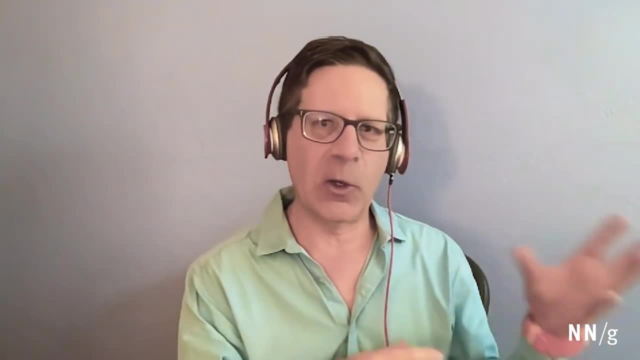 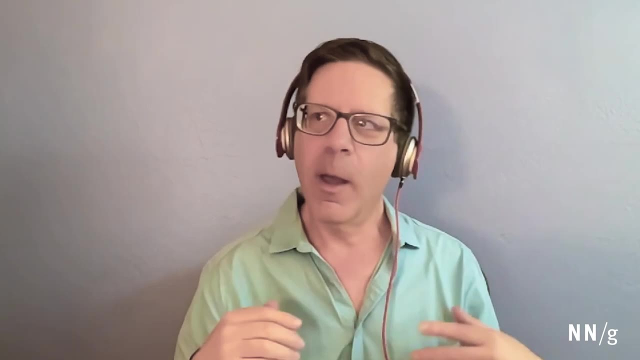 that legal person set up to empower a research person to do their work, as opposed to maybe in the past they maybe weren't told about it so that they didn't block it. So, um, you, and that's kind of an, that's some operational mindset that says, you know, what do we have to? 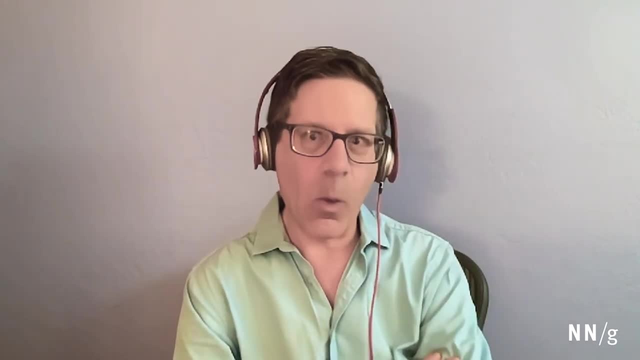 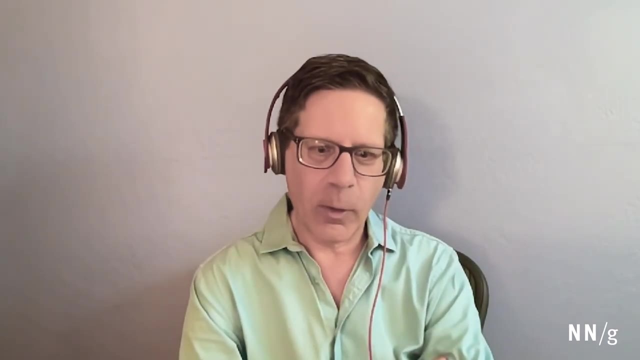 do as an organization to be effective This way? what tools, what practices, what skills do we need? Um, and so that I mean that's a very mature um kind of narrative about how research works inside the organization. 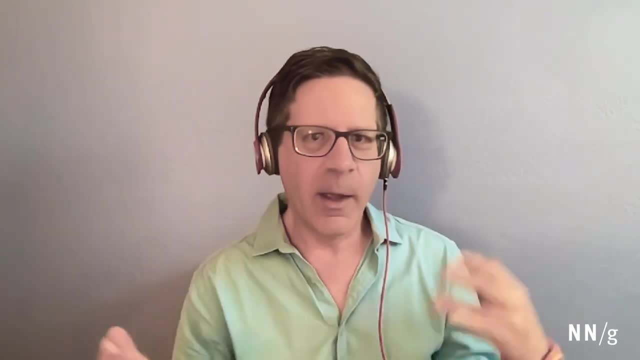 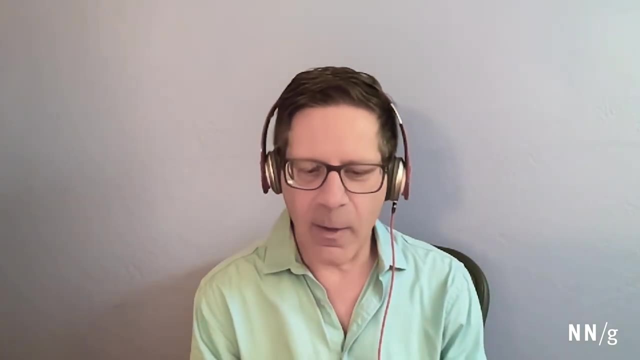 So it wasn't in the organization as much, And if it was, it was, you know, maybe opportunistic or kind of, you know, small and not sort of fully empowered. Um. so I think that that, and you know, if that's not you, and and you know you're. 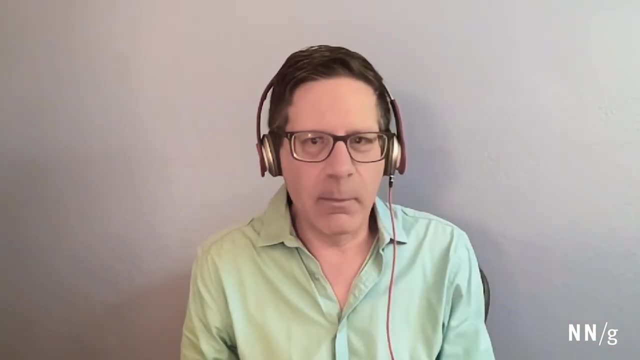 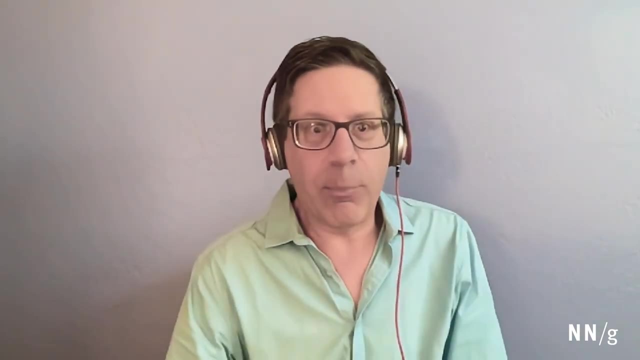 listening to this, you know, like that's not you. Um, you know, I would say like I don't want anyone to feel bad. I think you know you're now part of a more mature uh practice and there is sort of 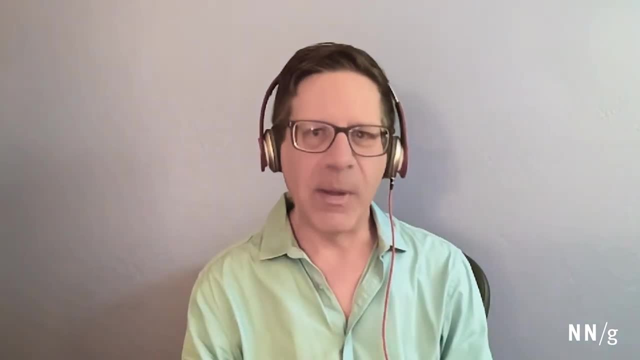 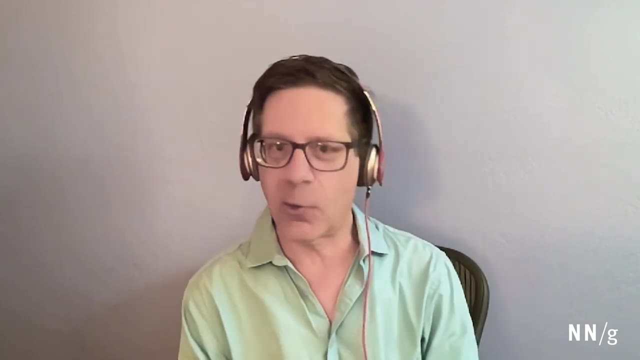 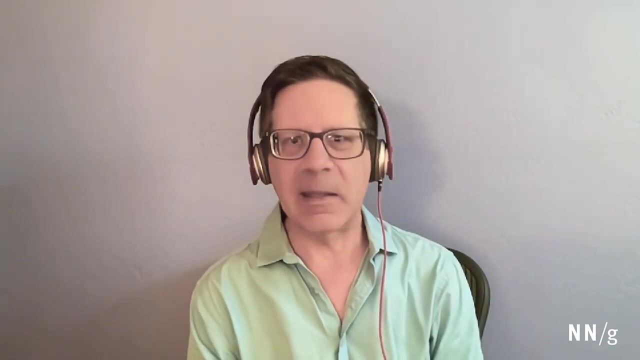 better examples about what this looks like when it's kind of built to scale, fully staffed, And you know, yeah, it's a big. I don't think everything is rosy for researchers in organizations or as partners at all. It's hard work, it's uphill work, but, um, you know the baseline or the examples that. 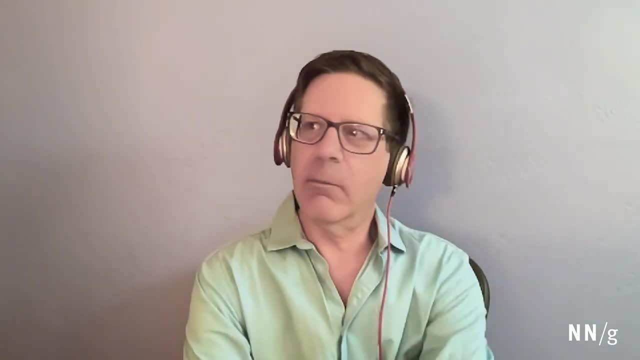 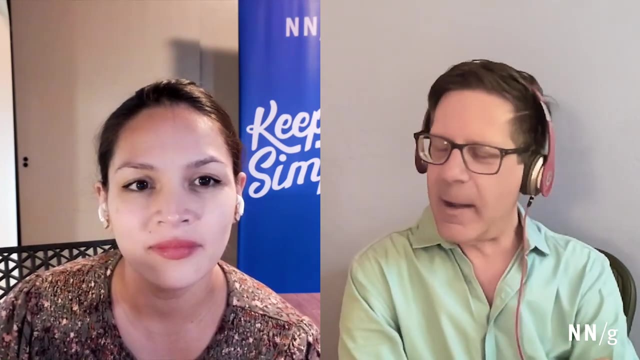 we can look left and right and kind of see Where there's a commitment and an investment, um, and what a difference that makes. we didn't, we didn't have that 10 years ago, So that that context has really, I think, changed. 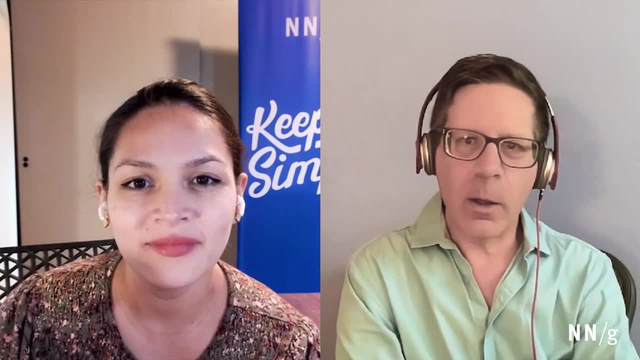 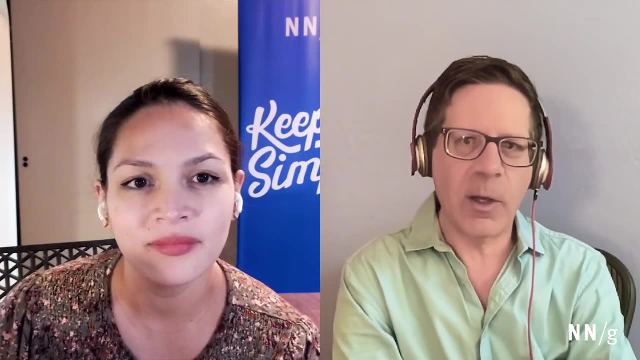 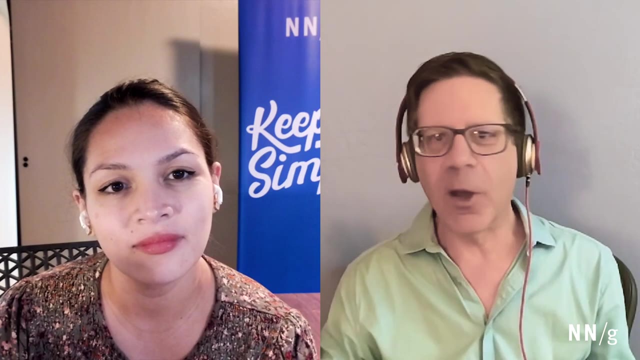 So you know who I'm writing to now and what I want to kind of arm them with. um, you know I have more, much more to pull from and I have a little more clarity and direction in trying to address the different participants in research: the researchers, the PWDR kind. 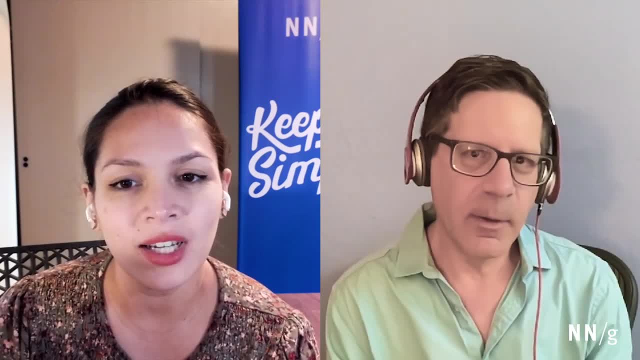 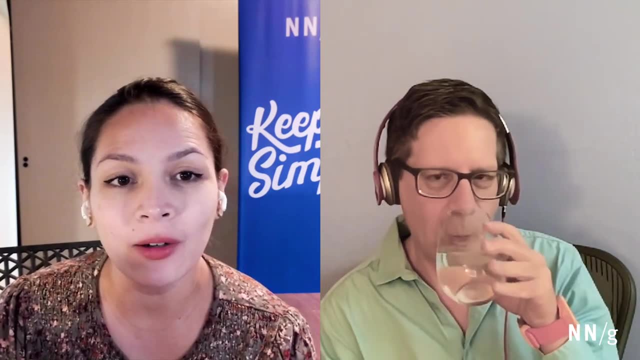 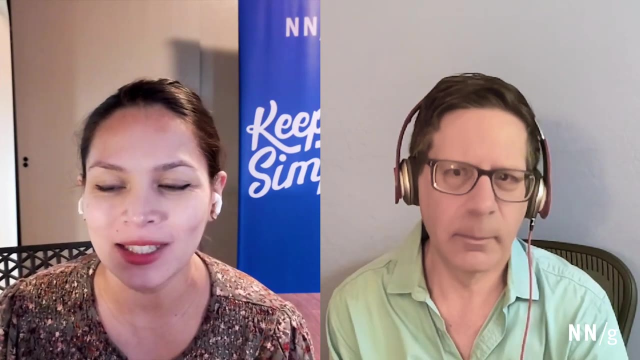 of you know that. Yeah, definitely, I think overall I totally agree. I think the field has really matured to the point that we're not only saying research is important, which I think was sort of the the chant you know that we often had to basically repeat over. 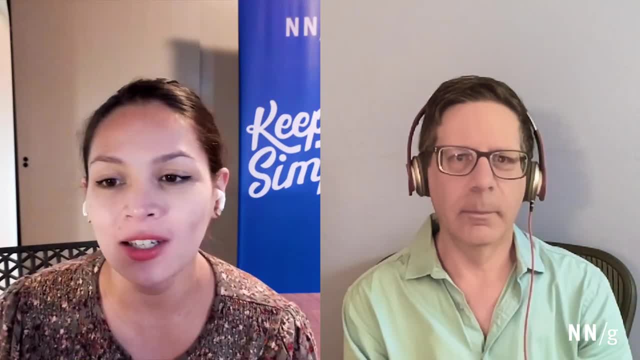 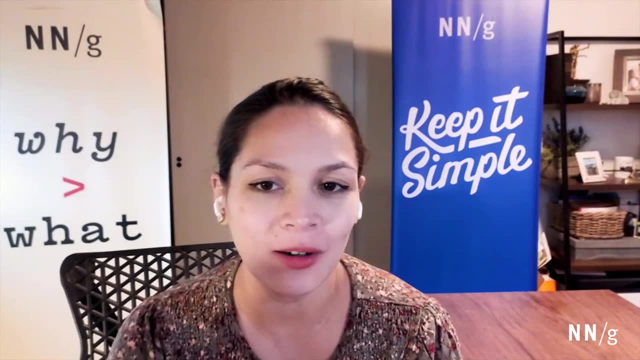 and over and over in order to get seen or even taken seriously. uh, in a lot of meetings we've kind of moved beyond that, where now there is- generally speaking again to what you said earlier- there are some organizations that are still 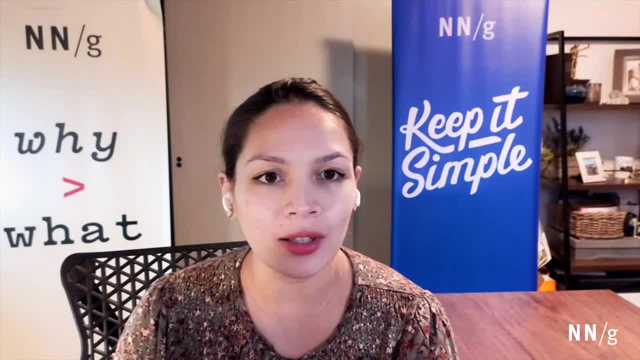 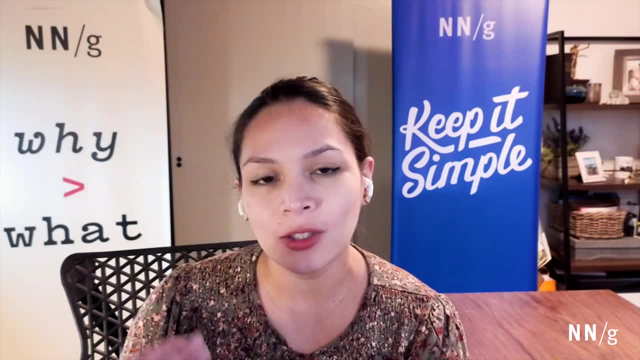 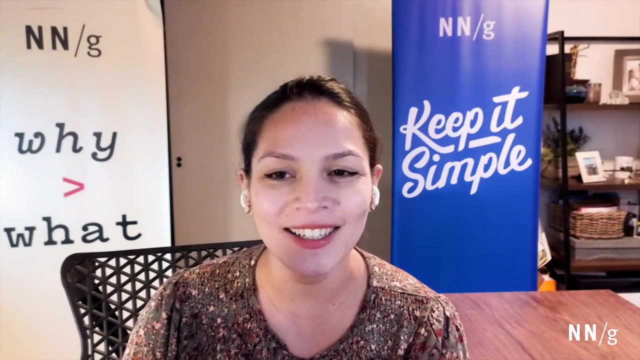 A little bit less mature, you know, as far as what they're currently incorporating in their research practice. but overall, the field knows the importance of research and has started doing it often. Um and so now the question is: well, if we do have people who are trained researchers? 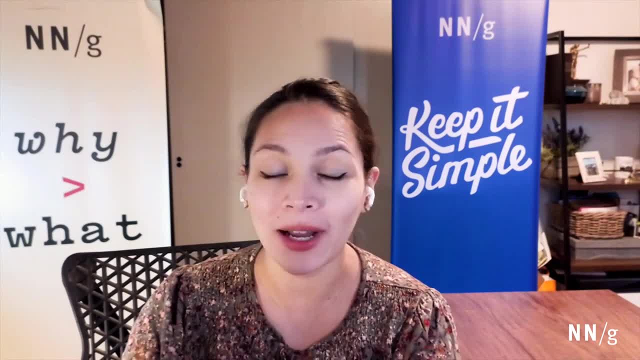 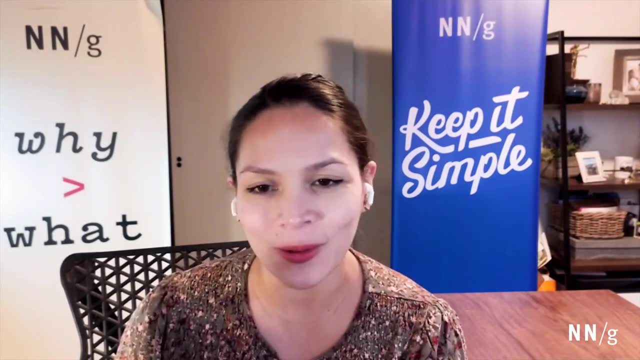 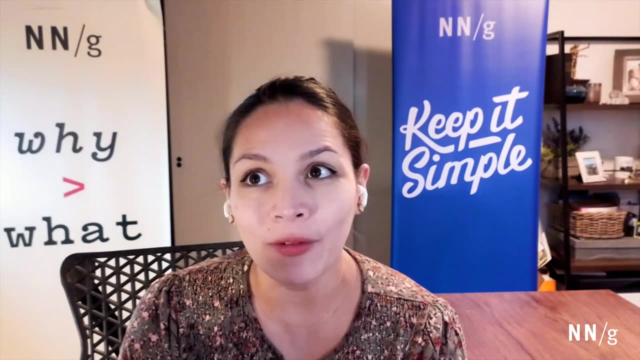 and if we have other people who are maybe not trained researchers but still see the value and maybe their organization doesn't happen to have that researcher role, can you still do these? And I think there still is room to do all of that. Uh, but I think there's also a challenge now where, if we have all these different people doing, 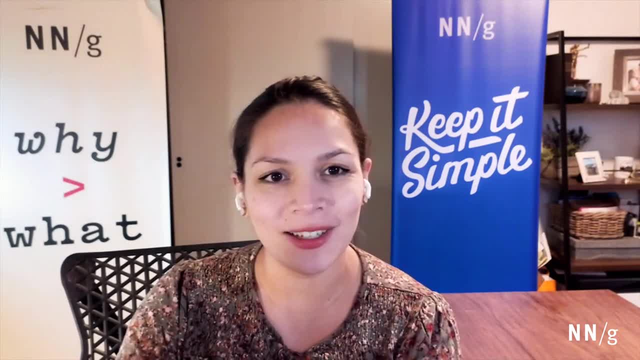 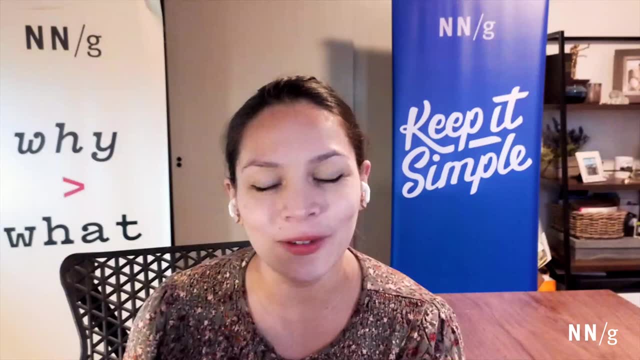 research and researchers doing research. how do we de-conflict, you know, perhaps overlap, And that's like a whole nother can of worms. Um, I know Kara Pernice has also done a lot of uh work in research ops has her own class on it. 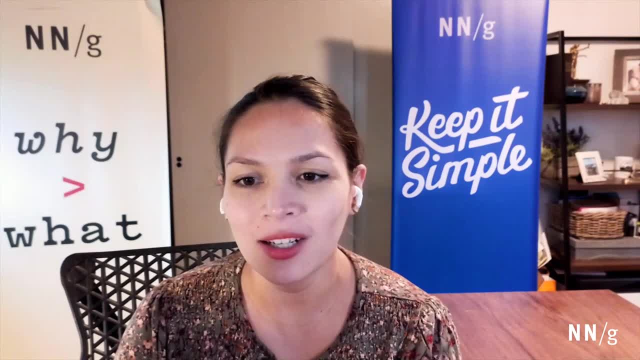 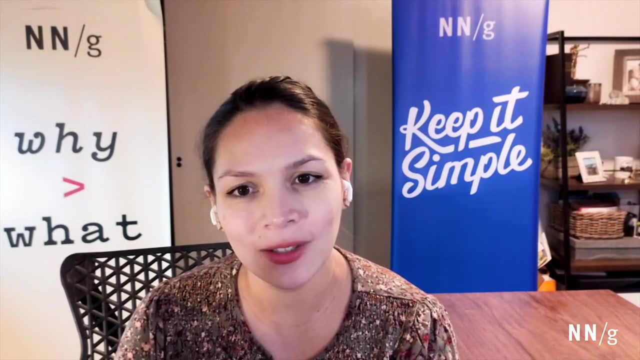 Kate Tauzy, like you were saying, is a great research ops, thought leader as well. Um, but yeah, that's, that's a huge change and a huge shift And I think it's a good shift overall, even though it is more complicated. I think that. 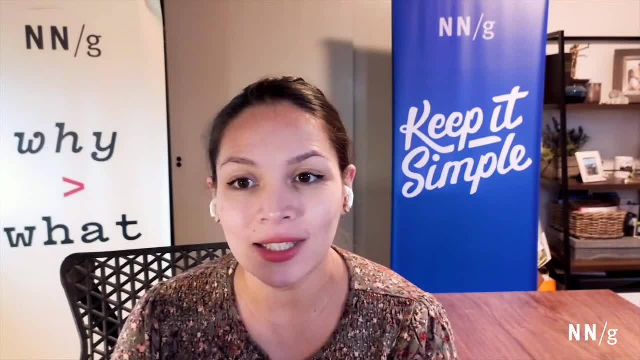 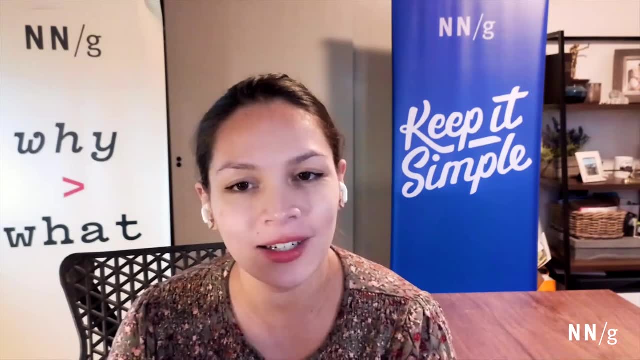 it bodes well as a whole for just the idea that interviews are something that people don't balk at as like an extra step, but as something that Hey, yeah, that's an excellent idea, Let's go. let's go and do that. 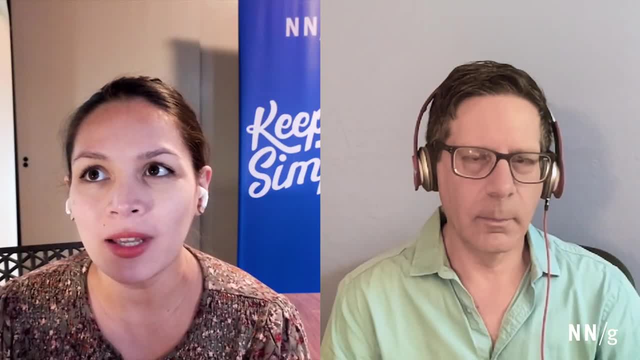 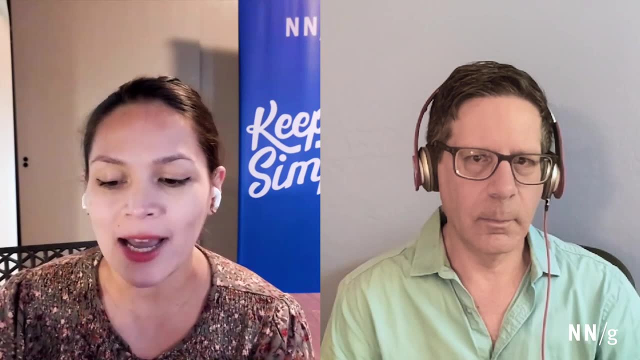 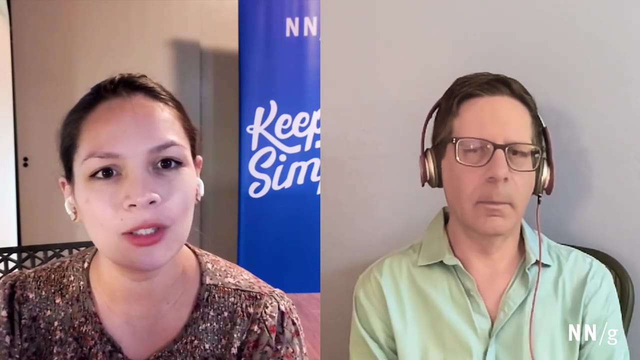 I guess a follow-up I have is actually about how maybe interviews are also more accepted or more readily accepted, in part by this kind of catalyst. That's in terms of the COVID 19 pandemic, which has now made remote research The norm right. 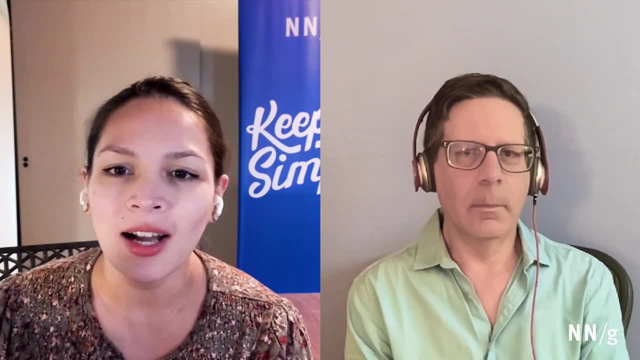 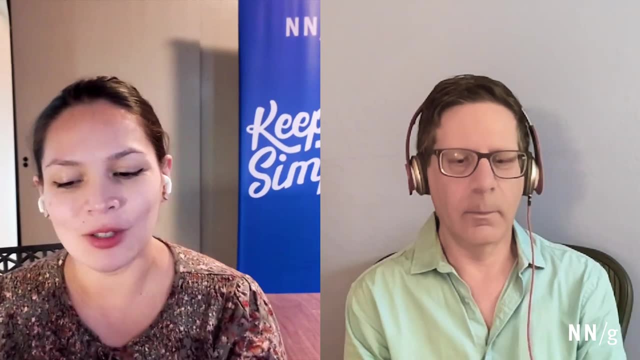 Which I think we were slowly moving toward that, but now it is very much the norm. So what are your thoughts on, like remote interviewing? Are these better or worse? I feel like there are some. there are different schools of thought on this and I would love 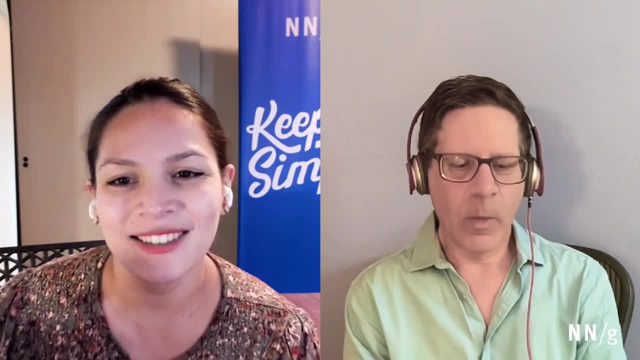 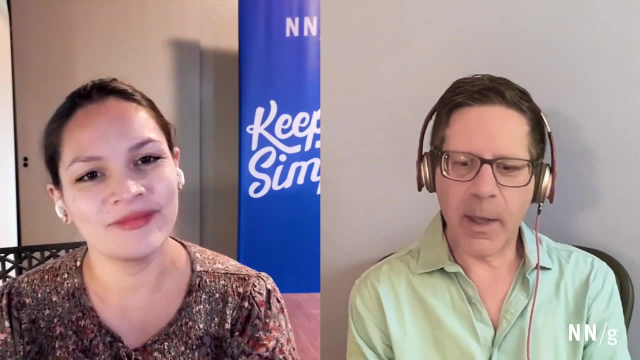 to know what you think. Hmm, Yeah, I mean, hopefully it doesn't have to be a binary, like we're only doing one or only doing the other. uh, you know, there's some, certainly some benefits to remote research. It's um, it takes. 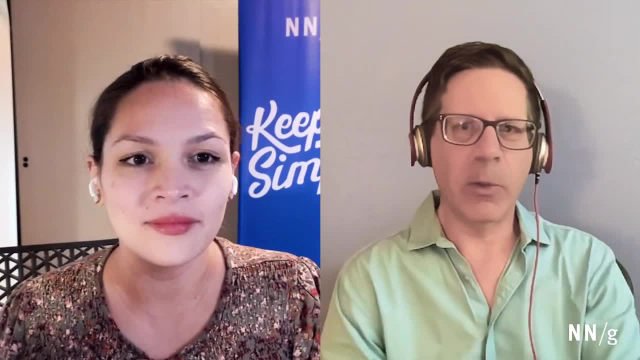 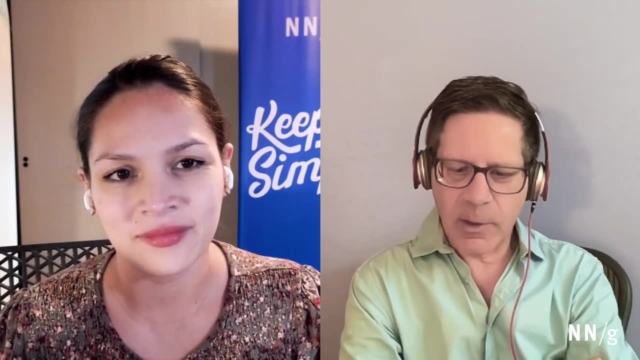 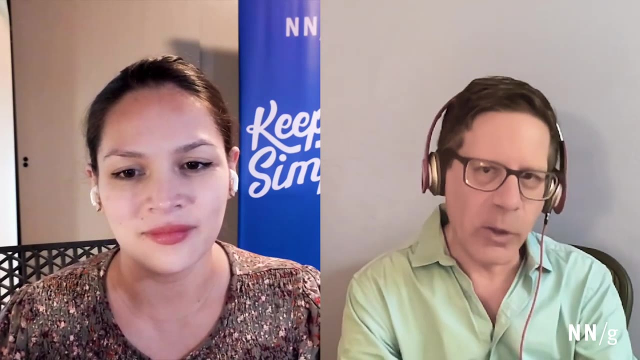 less time because you're just at your, at your computer, to do it. Um, I think- and I don't know if this is totally right, but I think it- it there is some, some narrative that it provides um, more, more opportunity for inclusion, um, that you might, if you're the researcher or 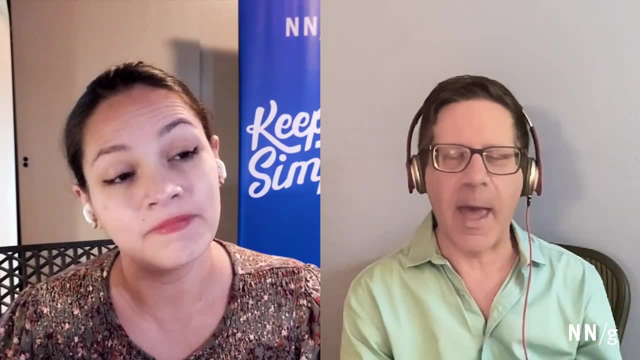 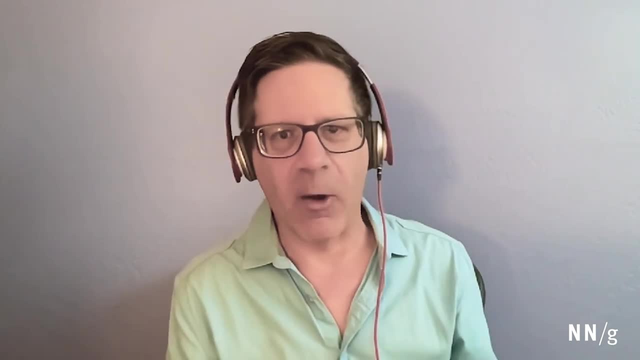 planning to research. you might be able to quote: get to places that not that you couldn't go, but maybe you wouldn't go. One example is, like people in rural environments know that, you know it's sort of if you're going to do in-person research, you might go to a city and like 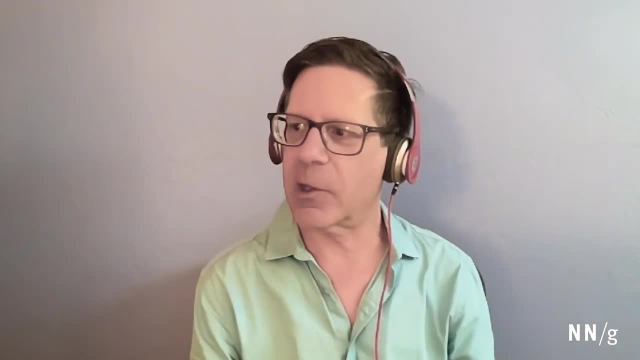 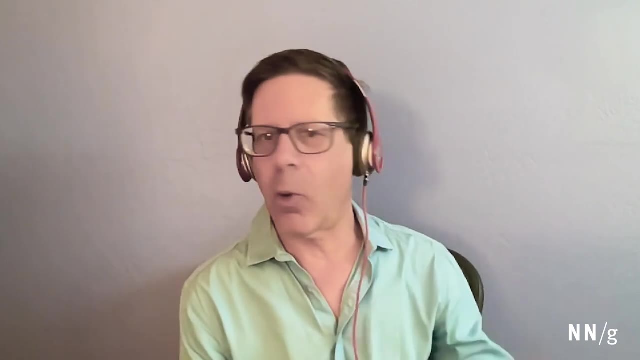 you know, very quickly you can get a bunch of different kinds of neighborhoods or different demographics spread, Um, but to go to, uh, you know, a low population area where you got to, you know, fly to a small airport and drive and and so on. that is. 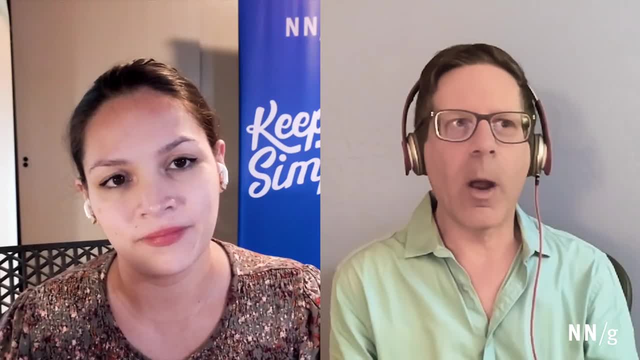 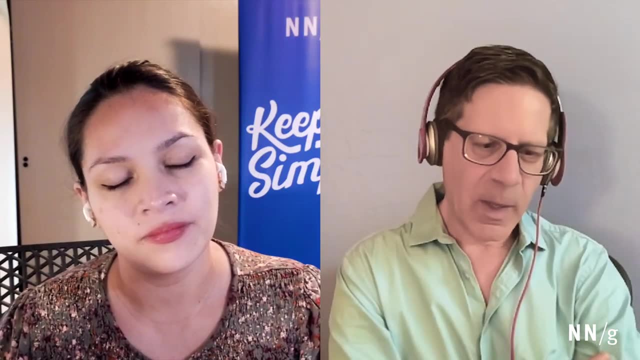 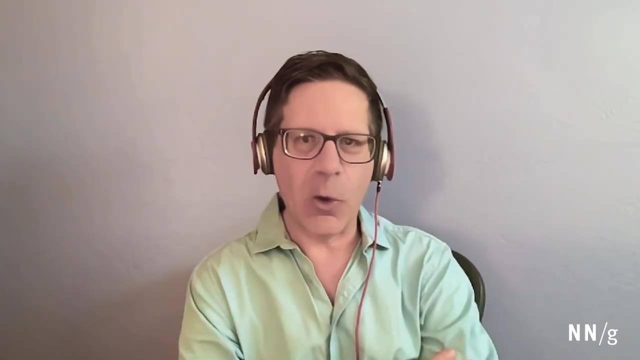 like. the cost for that is high. That's one area where um, uh, where you can bring in people that you might not be able to access as easily or you would have chosen not to Um. I think there's um- you know, more complex issues around um. this is very technology based, So 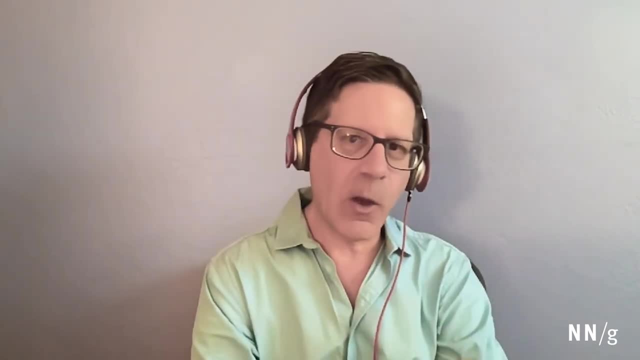 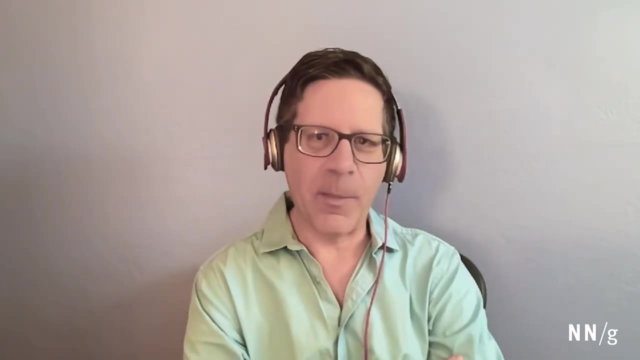 are we including people? Are we excluding people that don't have access to this technology? Um, you know, I suspect we're just replicating the biases that were in place, but maybe we're introducing new ones. Um, and maybe there are, you know, people that are. 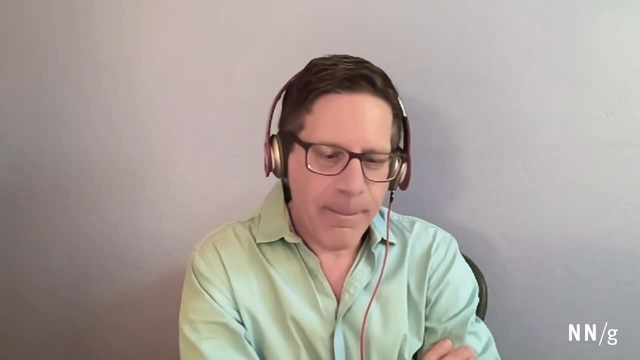 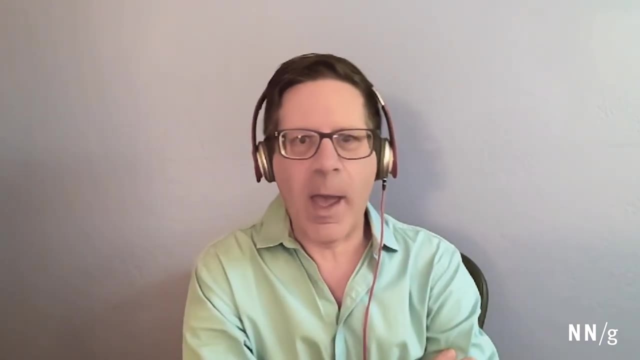 uh, you know that can. we can find people that, um, you know, maybe aren't office based, that aren't laptop based, but that are carrying around a phone and using a phone and, um, uh, where we can involve them. So I guess I think there's an inclusion question and I don't really 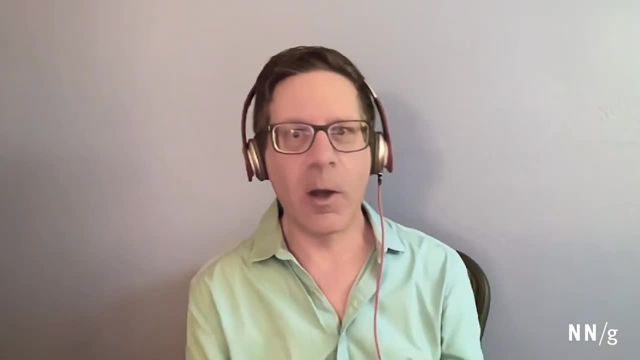 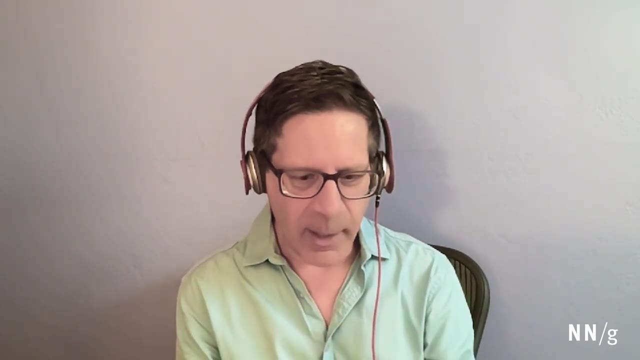 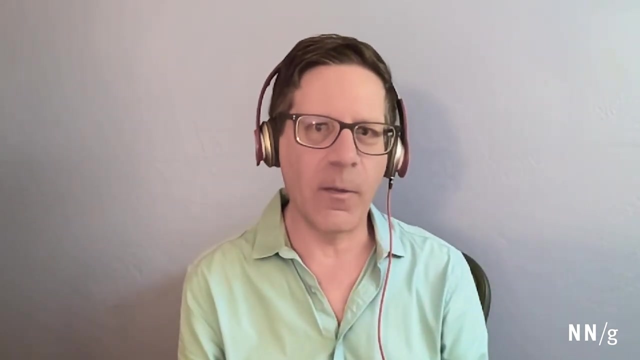 want to come down hard on, like this is what's happening, because there's, you know it is still a shift and I think it's, but it's an opportunity for people to consider Those things. Um, I, I grieve- and I'm using that word pretty strongly, Like I grieve the loss of 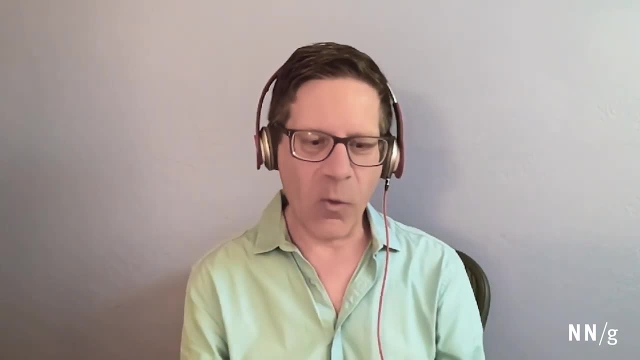 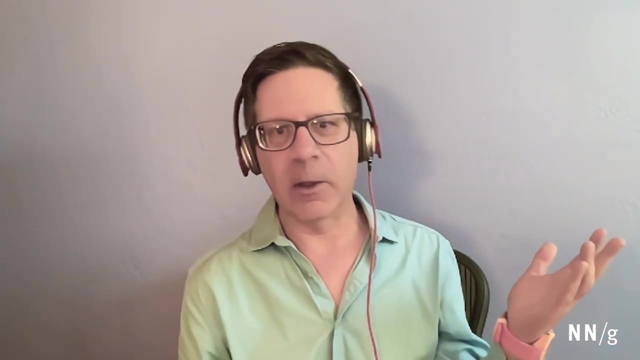 in-person interviews because, um, you know for all- and you were saying this really well- about the connection we have with people, it's different over a computer. Um, it, it creates challenges And this is I mean we know this because all of our meetings and keeping in touch with our 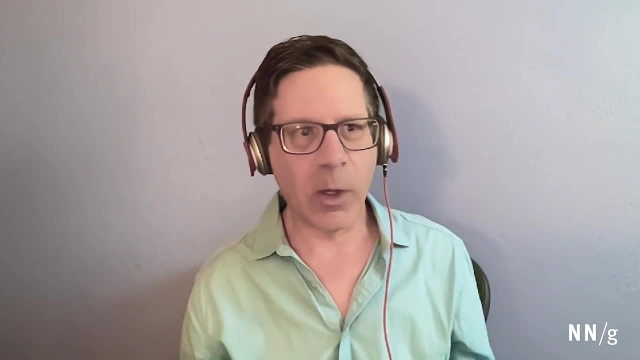 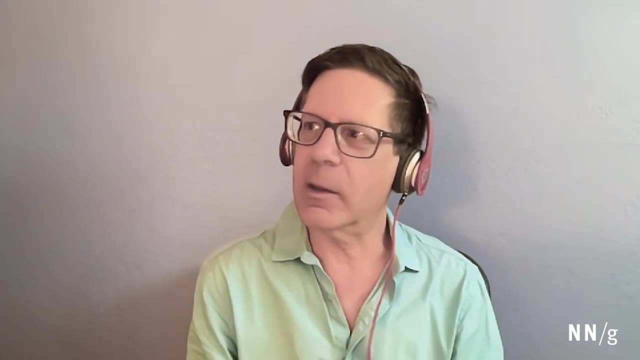 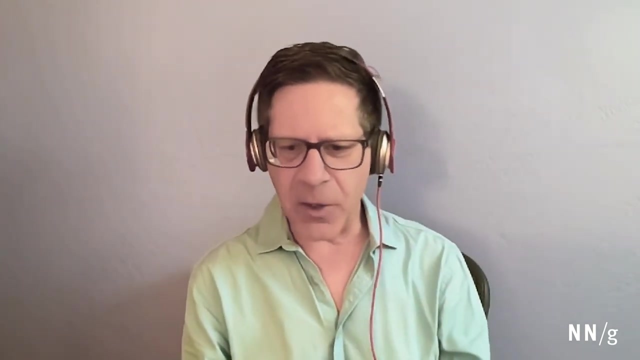 extended family, like we've lived our lives, you know, to a greater or lesser extent, for several years this way And it's it's created new opportunities and it's limited other kinds of things. Um, and I really miss um. there's just an excitement and a fear and a 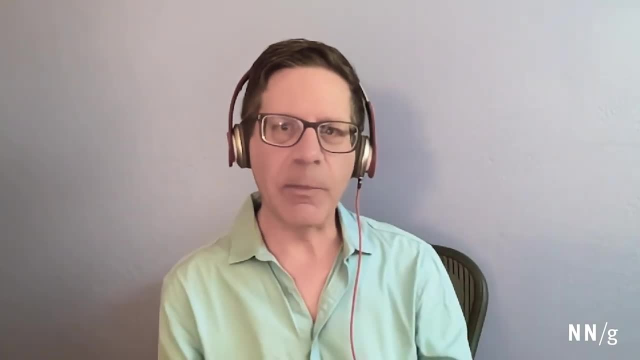 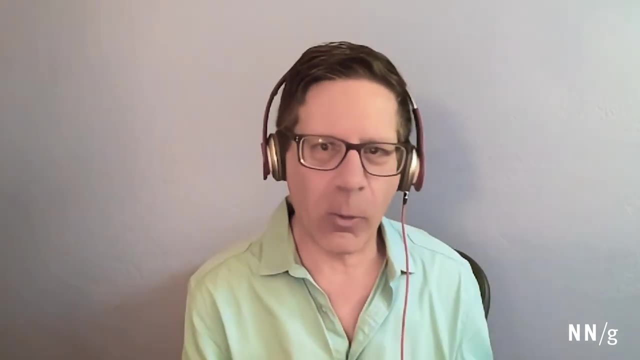 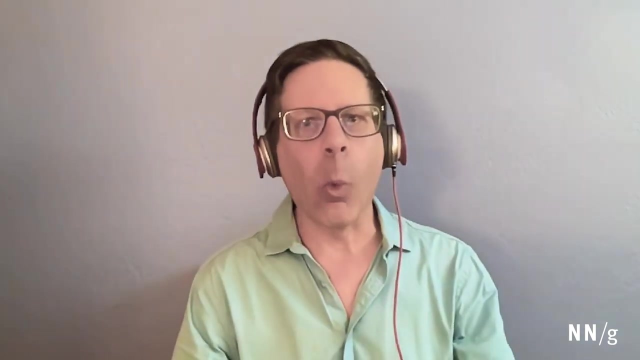 challenge and an inspiration that comes to me from being in the same room with somebody and seeing what their environment looks like and being shown around their workspace or getting a little tour of their house or peeking in their fridge or whatever that is. And you know, yes, there are workarounds to kind of how, how do we get that data? I guess I'm 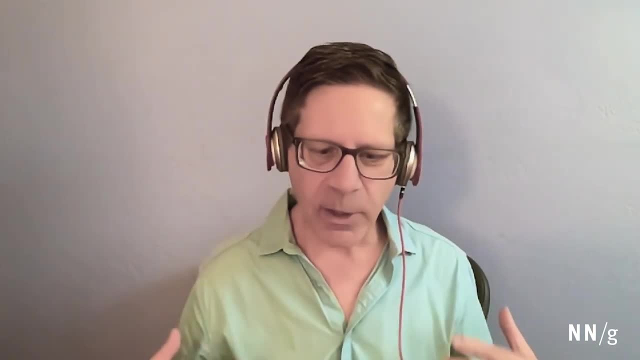 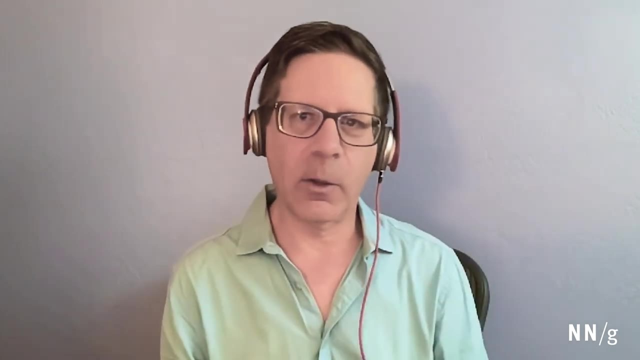 talking more from, like you know that, that human, experiential aspect of research. I enjoy talking to people and I get something out of it when I can go meet them. Um, and I'm an introvert, I don't want to do that all the time. It takes energy, et cetera, et cetera. 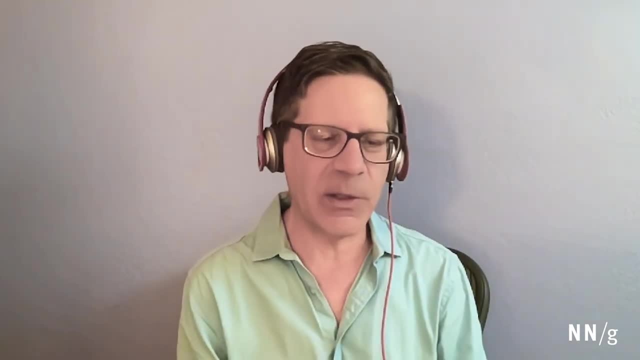 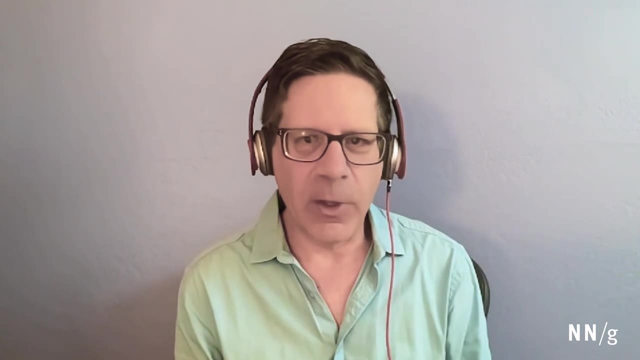 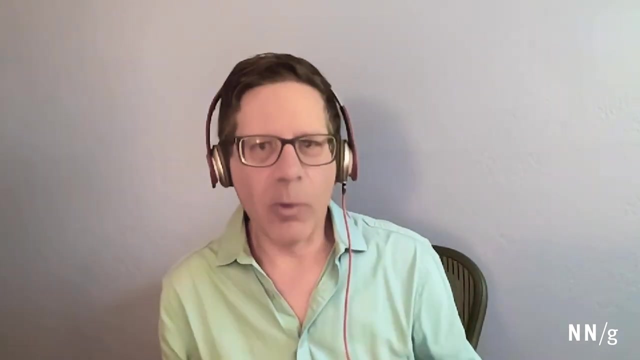 but something really amazing happened. So I would love to see us, you know, move to sort of using when and where and how we we still do this and that. um, you know, we've we've been talking all along about how do we kind of combine different methods- I think some remote, some in. 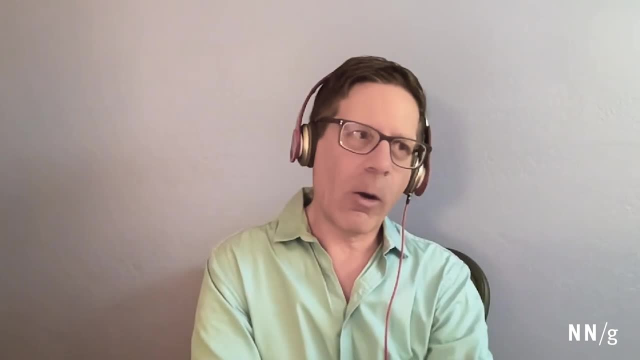 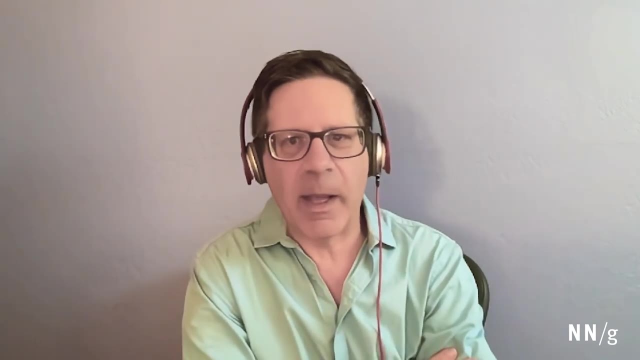 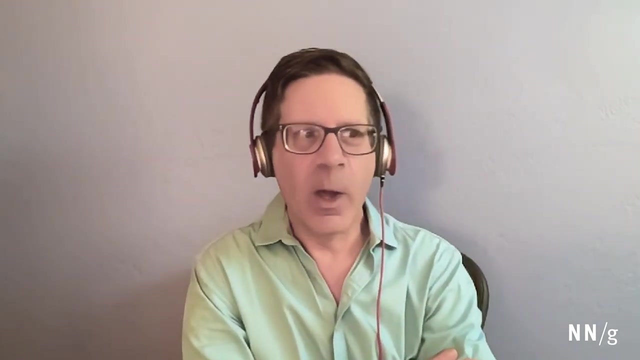 person. um, you know, so that we are are sampling broadly and, you know, being as inclusive as possible, but giving us- and Hey, it's not just me, Like when I take my clients out to do research- um, right To see what happens with their eyes, to see, you know, to drive back from the interview. 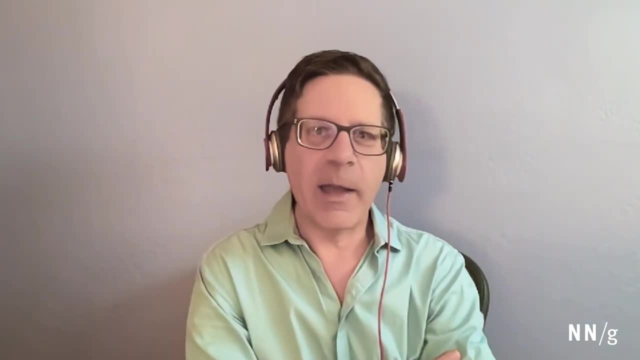 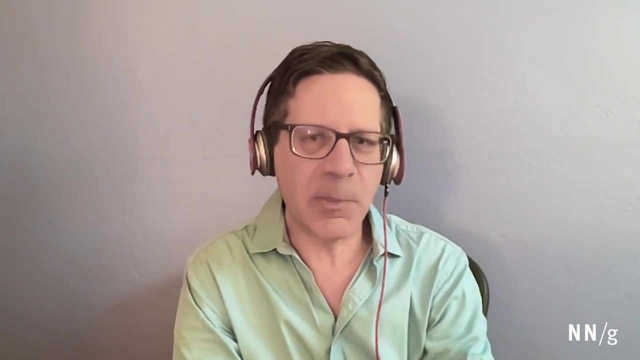 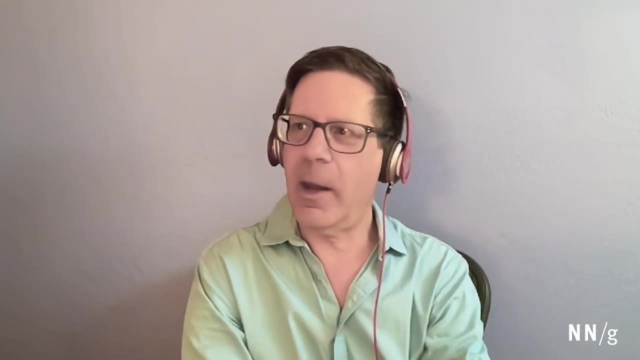 discussions we have. from these I mean fairly profound experiences, even about very ordinary topics like stuff happens. stuff happens to us And we talk about it and I learn about them. I learn about how they think about their customers. I learn about problem space. I learn about their. 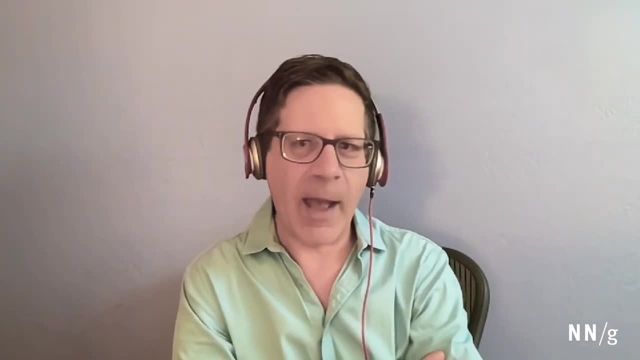 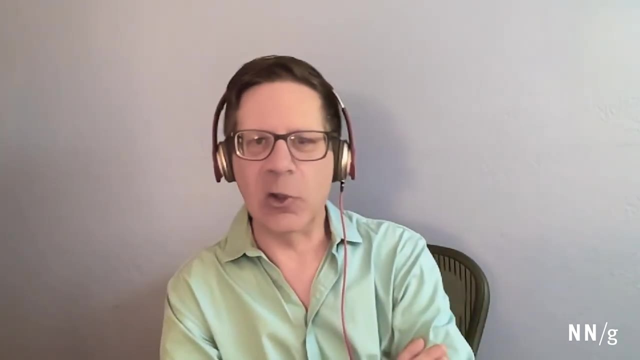 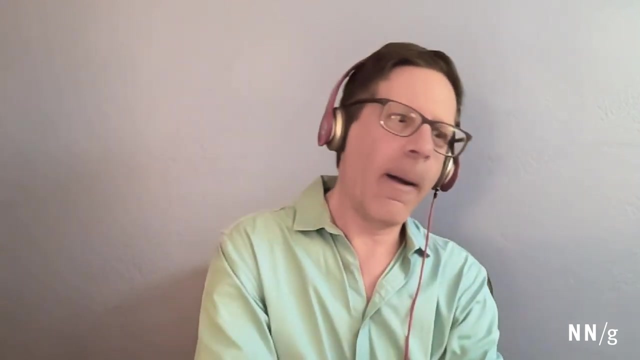 decision-making culture. Um, I get this interesting kind of access and we don't get that when we run a 15 minute debrief in the, you know, in the zoom, after we hang up the zoom with the person- And I'm not deriding those things- Those are like there's a lot of really good um. 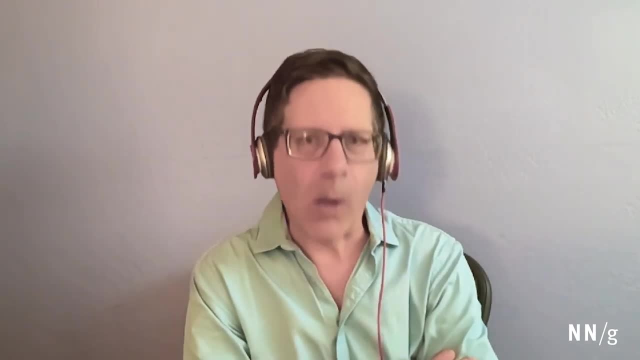 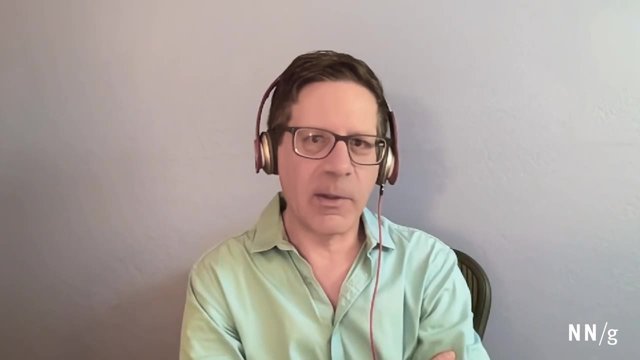 optimizing. that's happened in remote research, Like it's really grown up a lot over a few years. but I like the, the messier interpersonal aspects, uh as well, and kind of what I can get out of them. And yeah, I haven't done an in-person interview in. 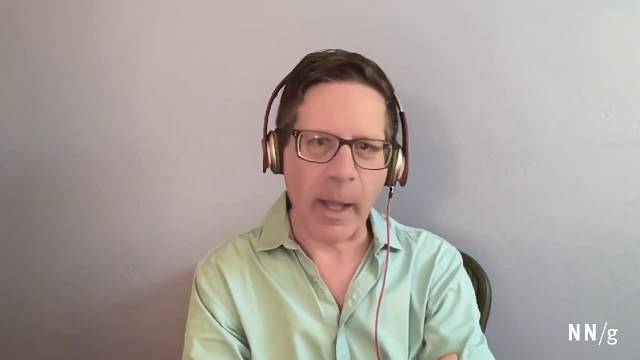 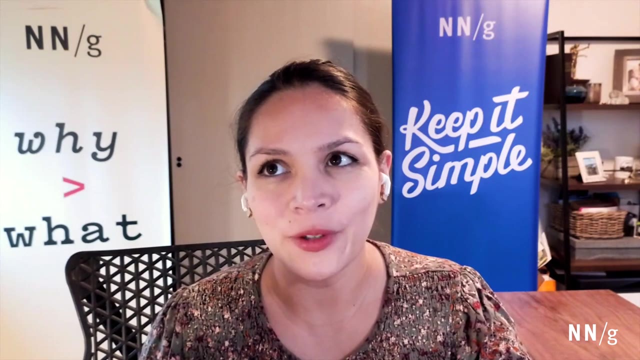 several years And I would, I would really really like to get that back into my life, because I just find it really joyful. ultimately, Yeah, It has been a few years for me as well And and, like you're saying, part of it is because it is cheaper. You don't have to travel. It's. 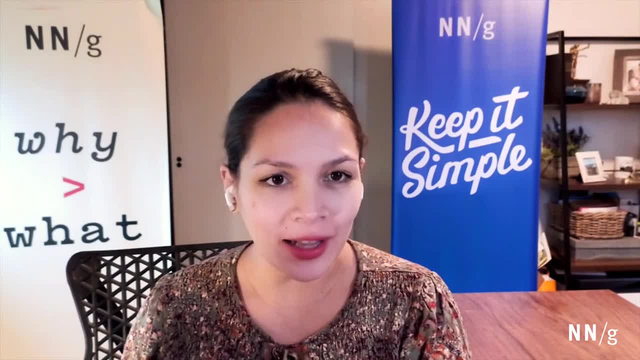 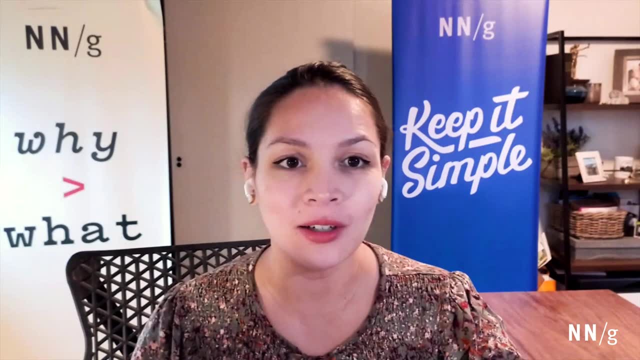 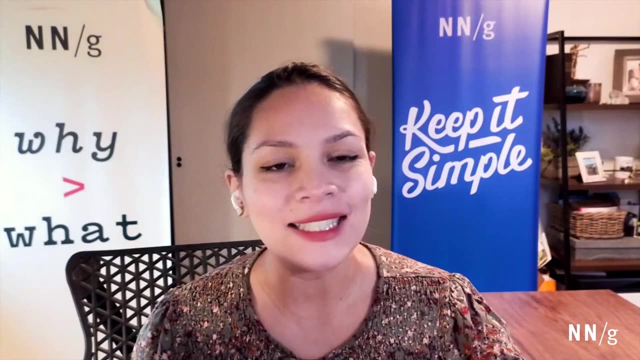 you can get easy access to people and- and yeah, regarding that inclusivity question- like there are lots of people who suddenly can do interviews that maybe in the past couldn't, because they couldn't leave wherever they're working to get to where the interview is, or we we couldn't talk to them as easily outside of these office. 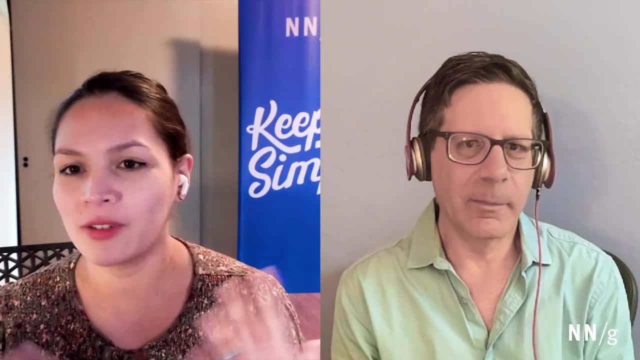 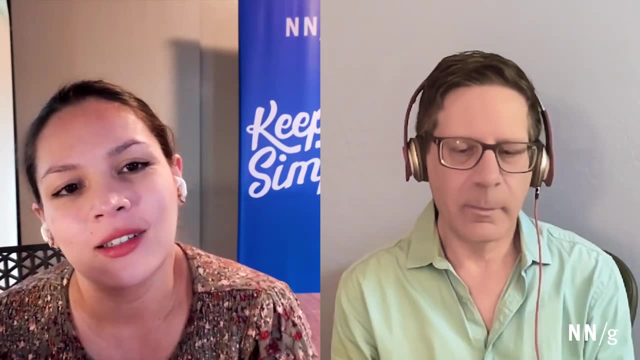 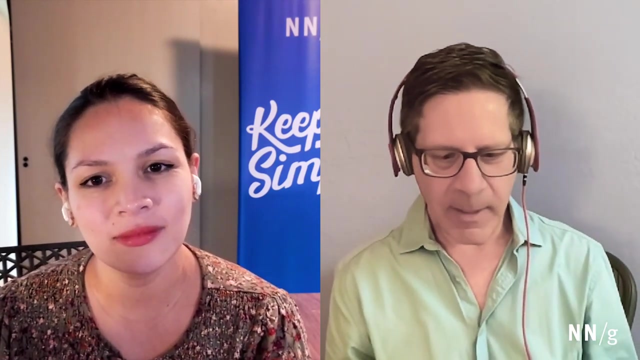 hours When thinking about the past 10 years. obviously, this is one big shift. There are many other big shifts. What hasn't changed in the past 10 years, Do you think? I mean this is still like a- uh, you know, uh- an enterprise of connecting with people, and 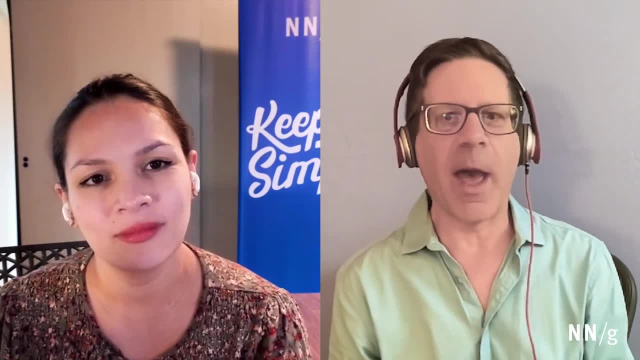 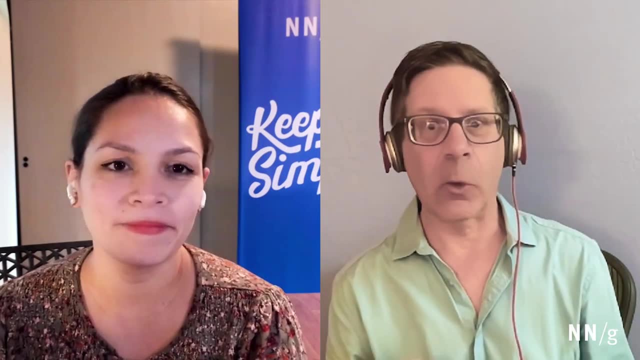 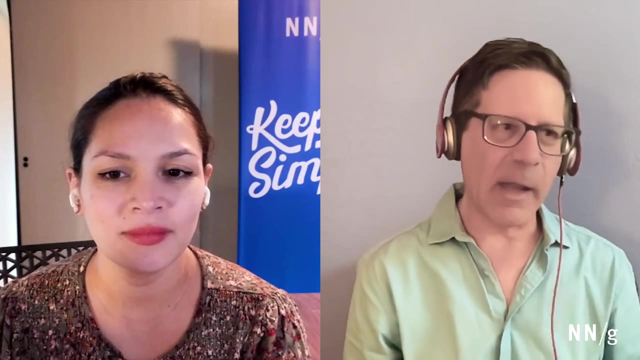 listening to them deeply and learning ourselves how to be good at listening deeply and, um, understanding what's not being said as much as what is being said, and learning where to follow up and, um, you know, doing the hard, the hard, heads down and collaborative work. 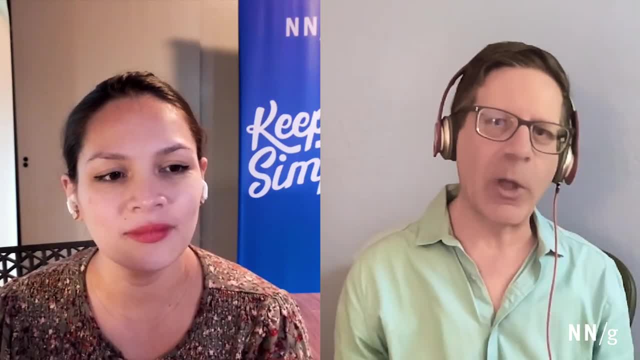 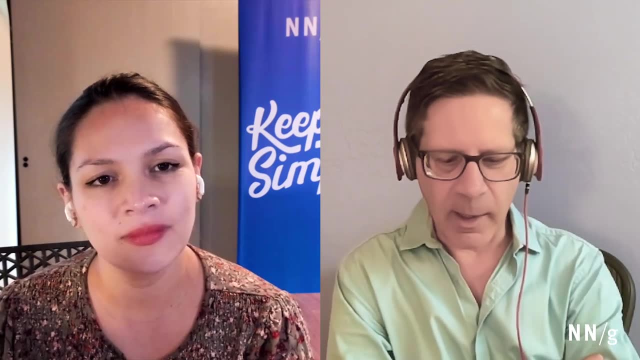 to, to connect these disparate dots into something new that we can bring together and recommend as a you know, as an implication or as a action that we can take. Um, I mean, that's, that's the work, Um, and so the tools that we 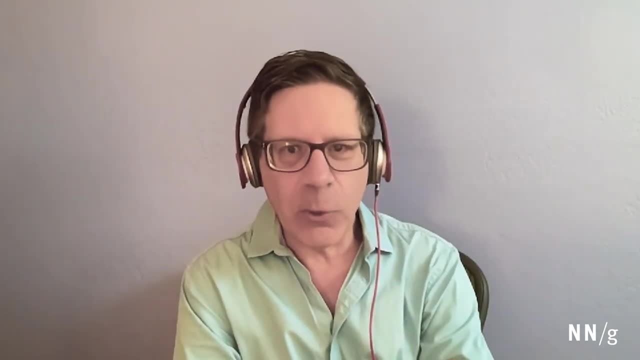 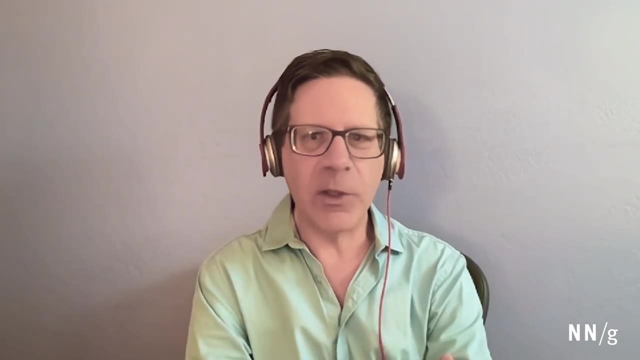 we use to do, it will change, uh, who's involved in doing it will change? Um, but that I mean at a, at a fundamental level. it is this sort of human to human and kind of creative, you know. 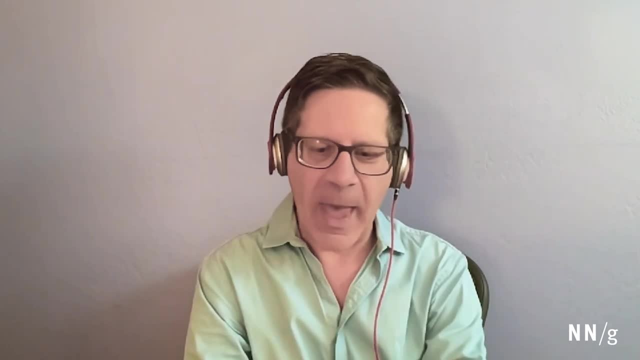 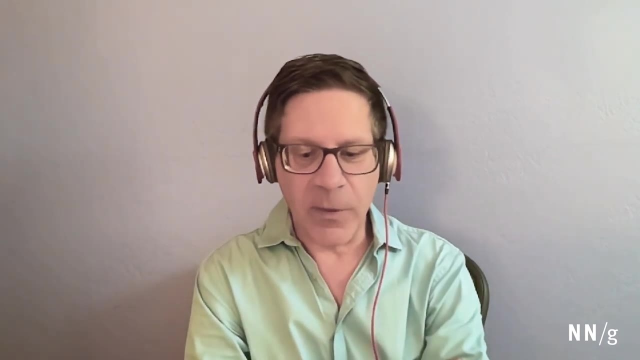 connecting disparate dots, sort of work, Um and that, and I can't imagine that changing. That is that is what we do, Um, so yeah, it's fun to revisit, like you know, in in re, in rewriting or writing an iteration like um. 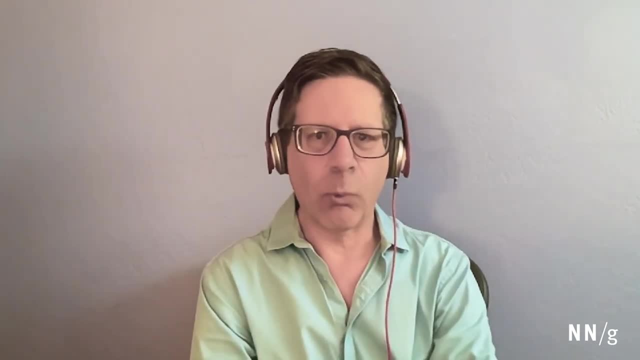 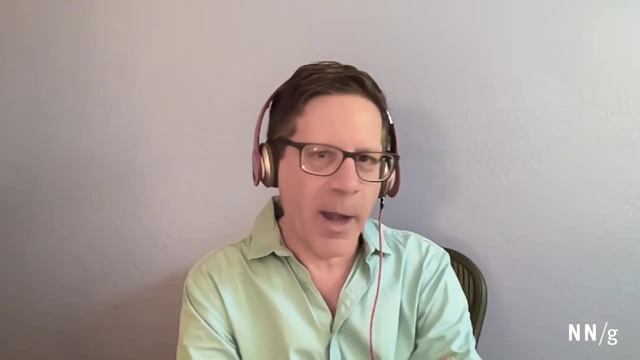 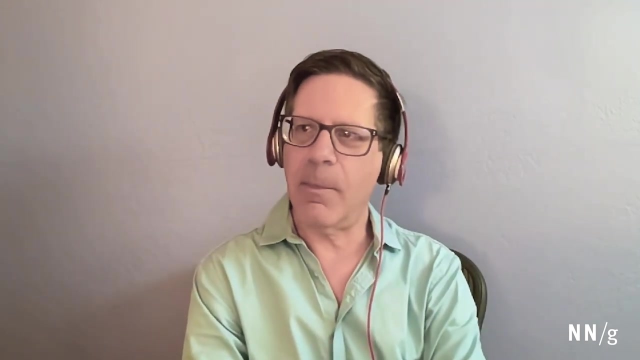 I don't think any of my advice from the past was wrong, but I have lots of my own experiences to kind of update or better ways of explaining things or things that I've tried and messed up, that that I feel like the context has changed. the fundamental sort of the backbone of this is the same. 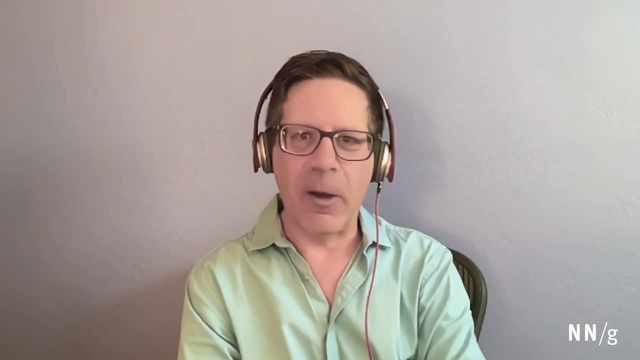 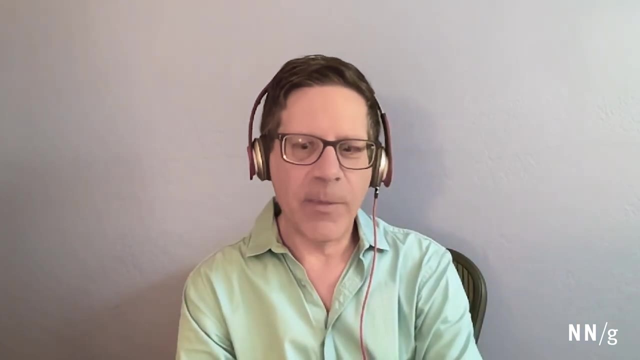 But, uh, I have 10 more years of thinking about it. that, you know, has helped me feel like, oh, I can explain it better or explain it in a fresh way. Um, so that that's kind of fun to do. 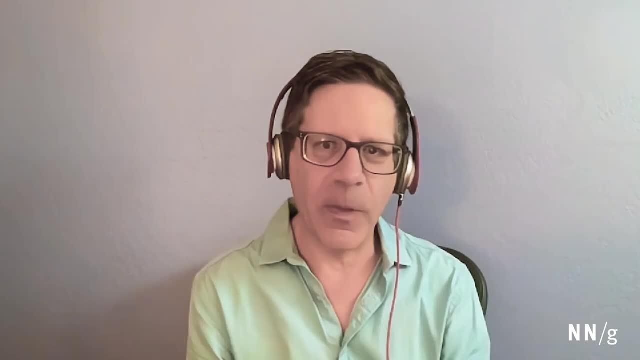 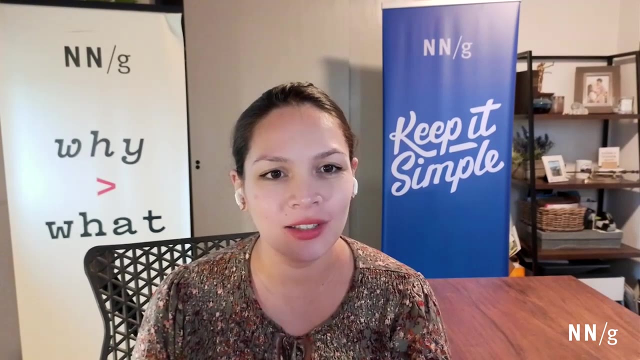 I think you know, as a, as a, as a writer or a thought leader on this stuff, that you know it was part of my, my thought process and my practice. I agree, I think over the last 10 years, that there have been a lot of changes. 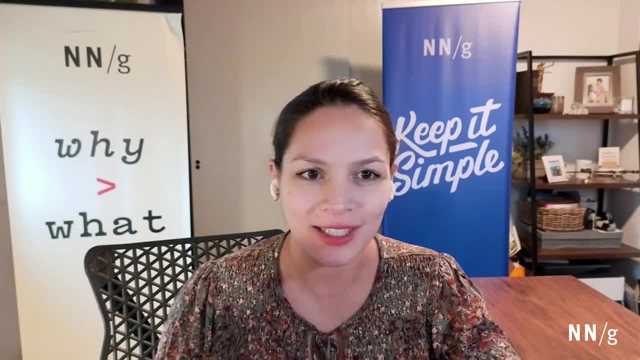 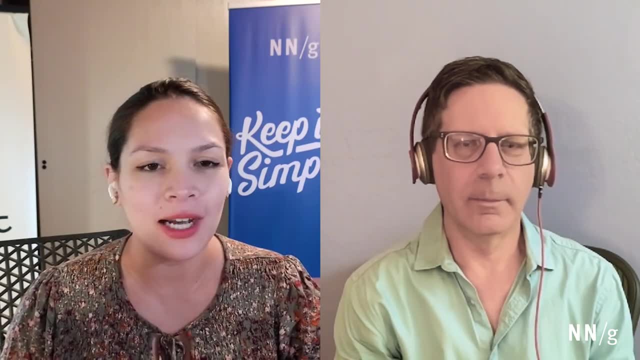 but human beings, like human to human conversation. conversation hasn't changed in eons right For for many, many decades, And I think there's always going to be this fundamental aspect of how do we converse with one another, How do we connect with one another. 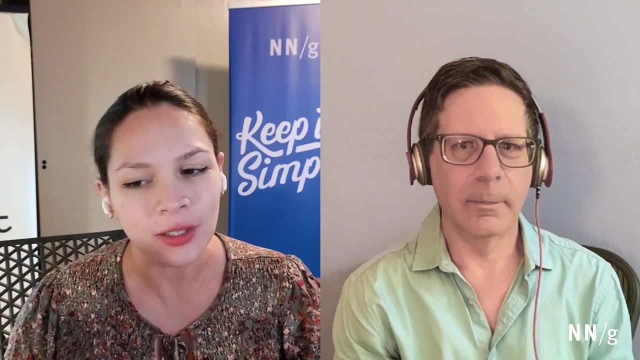 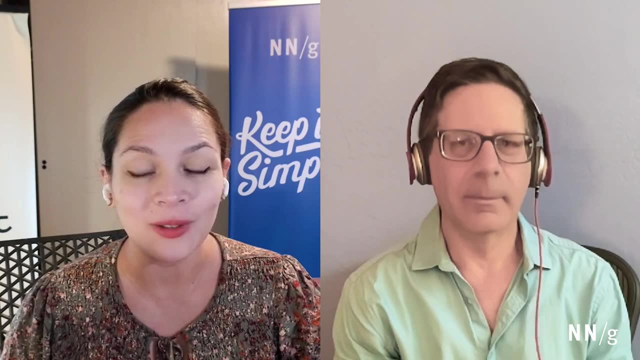 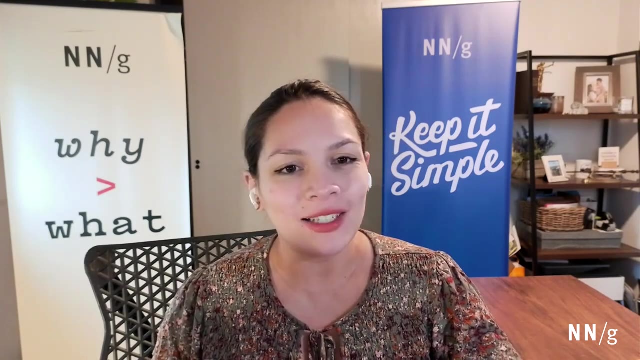 That that largely won't change. but but I also agree to with you in the sense that it's taken me many years to get better at interviews. Um, I do teach a class about it and I do know what some of my kryptonite sort of moments are. 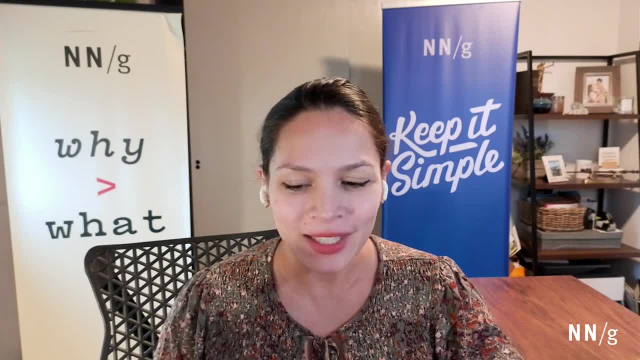 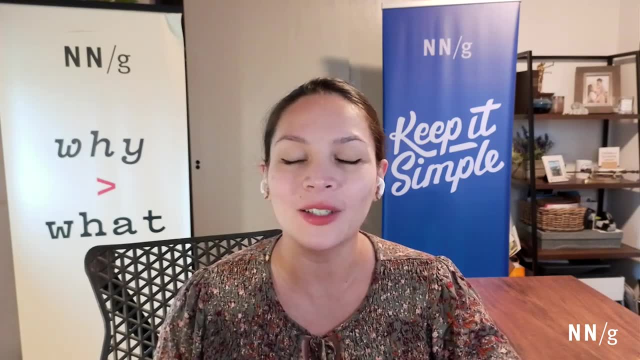 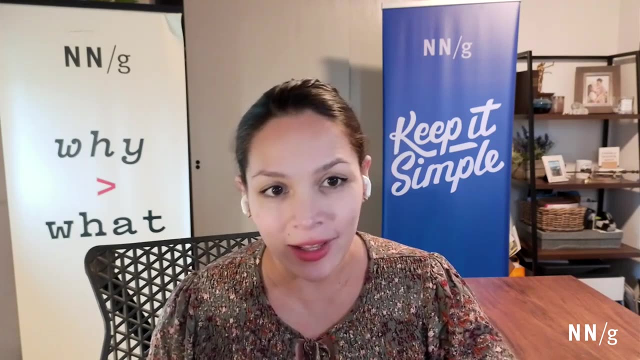 or some of my uh weak spots are, and I continue to work on them, but it's it often does take quite a bit of time to build awareness around some of these more logistical challenges, like how do I ask these questions or how do I convey that I'm listening. 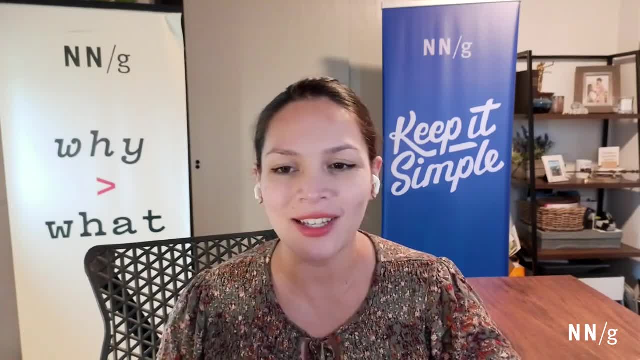 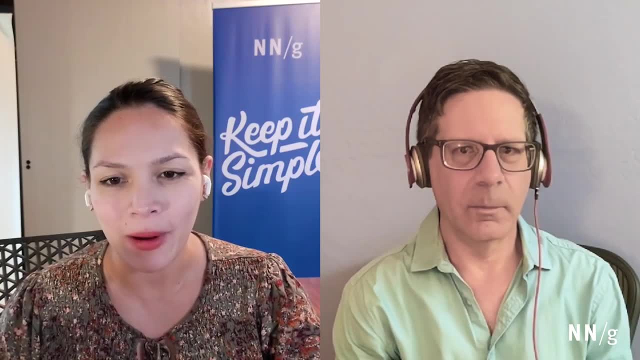 How can I be an active listener? How do I analyze the data Like? there's so many more things that I know I'm continuing to explore as well in our own research here at NNG. So, Steve, to wrap up, I did have one final question for you. 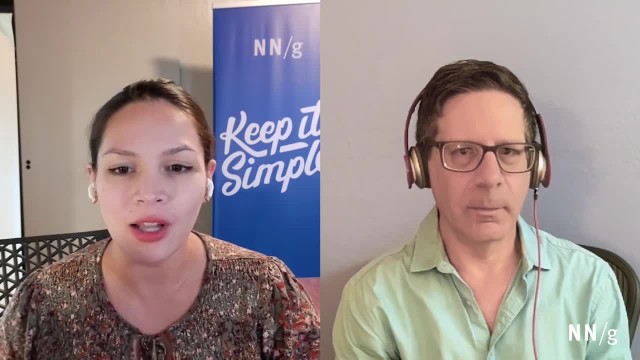 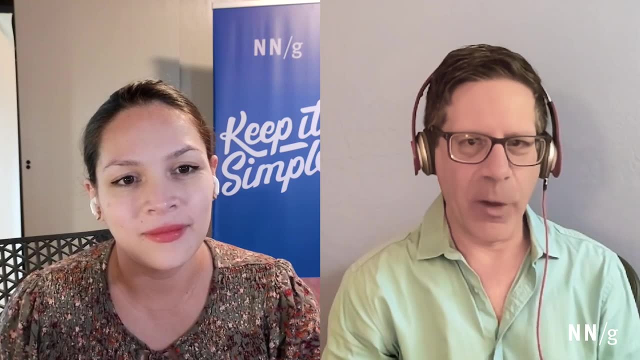 which was: what advice would you give to people who are looking to level up their interviewing skills? Uh, I liked your description of kryptonite. I think that we all have those And you know, one of the things that we get from. 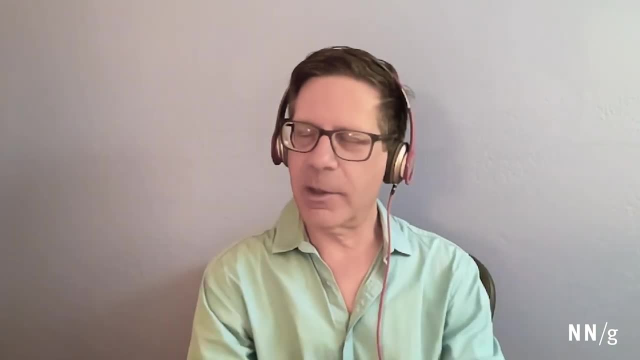 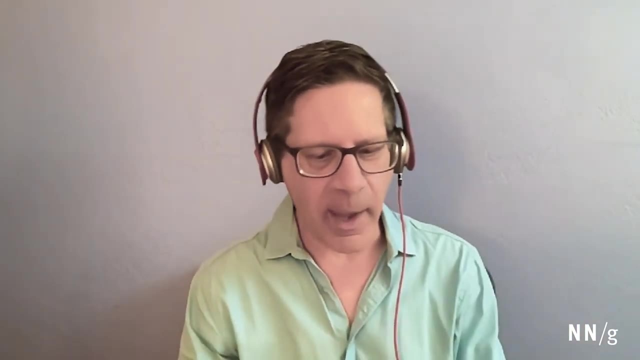 I don't know. listen to podcasts or reading books or just any kind of practice and reflect is is a chance to see what those are and, um, you know and reflect on them and and you know, and and try to work on them. 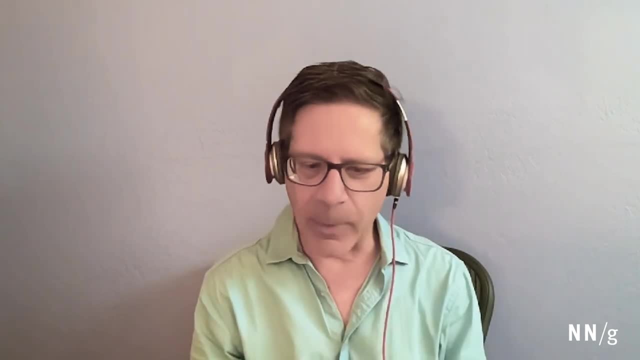 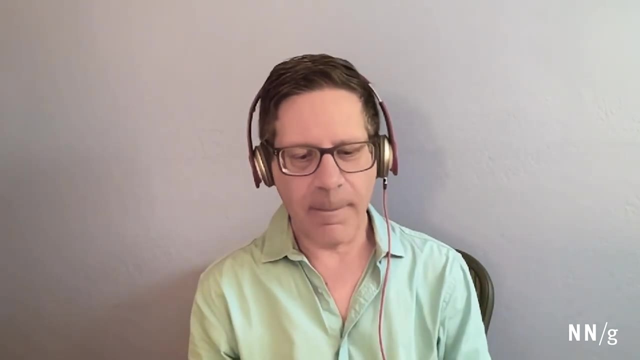 I think everybody is like that and you really put it so well, Um, so I'm going to highlight one that I think is fairly common and kind of challenging. Uh, and that is, um, it's about putting the question, putting the answers in the question. 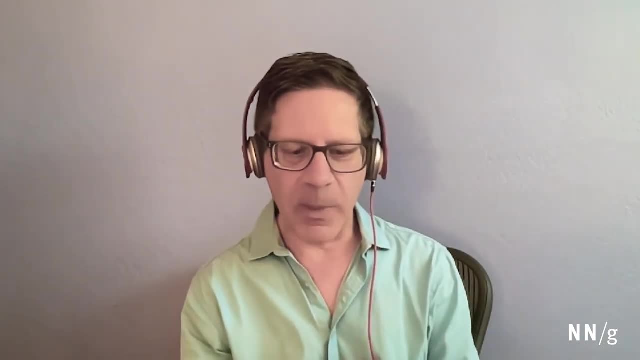 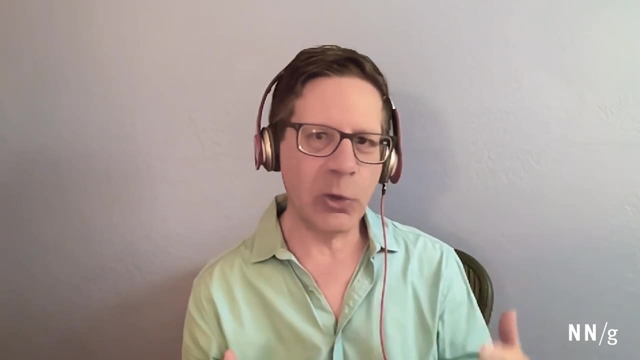 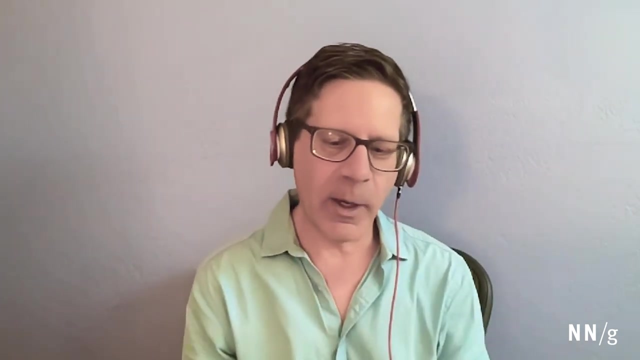 Uh. so I'll give a good and bad example. So what people might often do is say, um, uh, what did you have for breakfast today? Did you have toast or juice or cereal? and even kind of trail off. Sometimes they just kind of end with an error, with, like the voices kind of holding onto it. 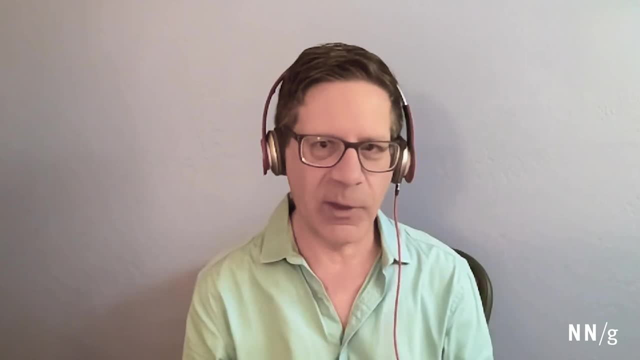 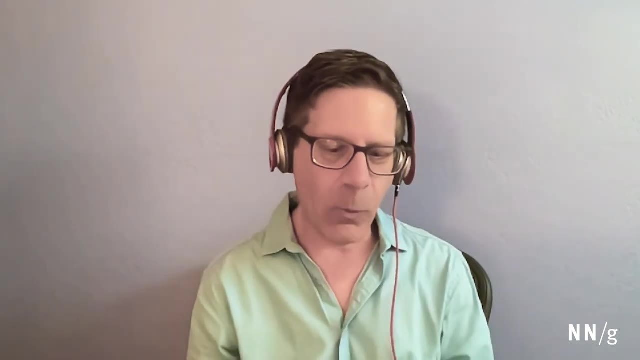 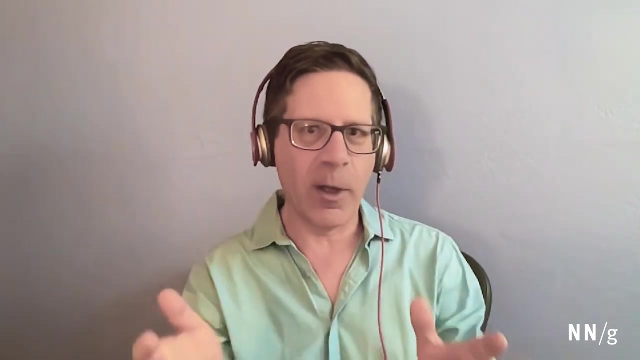 And the question, the expert question, is: what did you have for breakfast today? And I think, like I want to unpack a little bit about why we do that and why it's why it's bad. Um, we do that because, like, it's that moment at which you stop asking your question and kind of hand it. 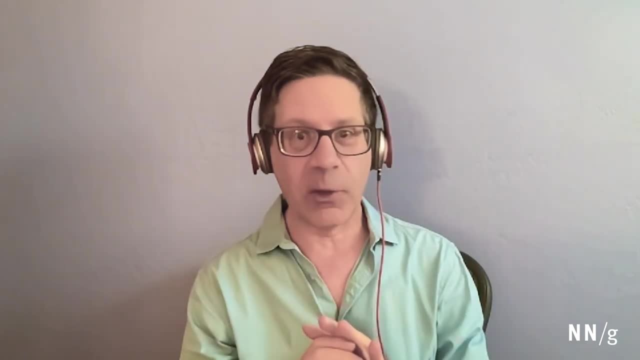 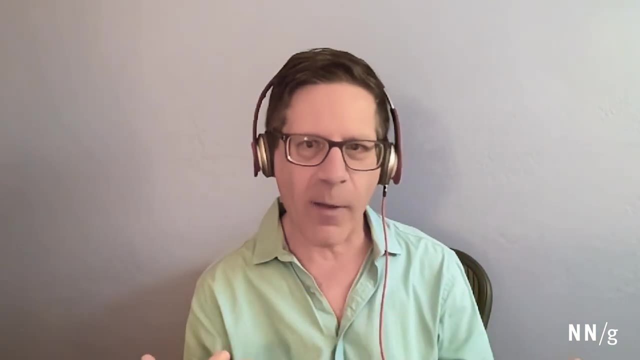 over to the other person is fraught. It's actually much worse in remote um because, like turn taking isn't well supported by the microphones, They cut each other off. a lag- a little bit of lag- in audio or video makes that very. 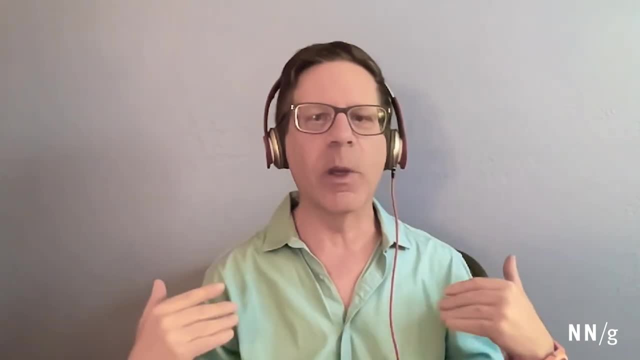 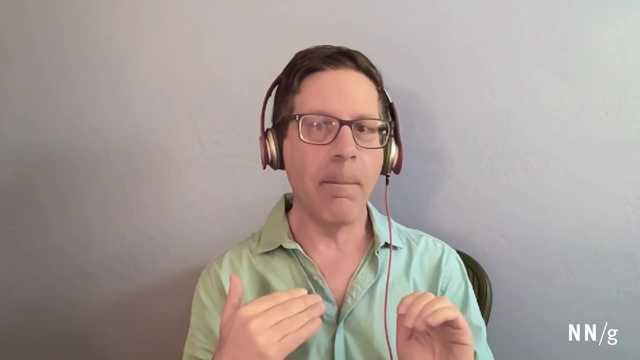 there's a very sort of automatic human We know about intake of breath and body language, Like we pick all that up when we're facing a壓. I love it like profits. you know to face with somebody and that's makes us better at turn-taking and that's really what that is. 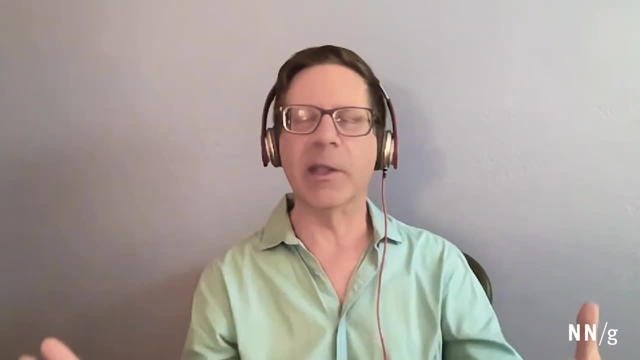 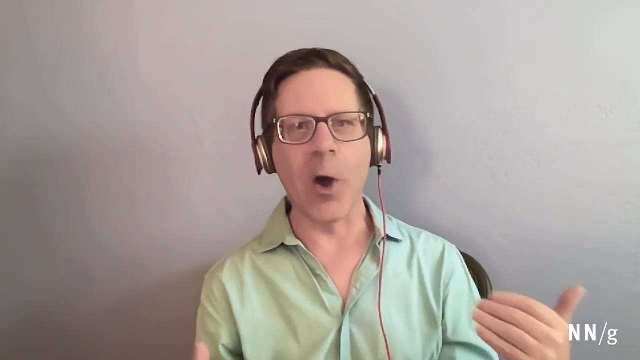 right, i'm done talking. now i want you to talk. so in remote it's even worse, but in general it's still uncertain. you don't know this person. some people, um you know, nod while the other is talking, which you and i are doing this whole, this whole uh interview um other people just keep their bodies. 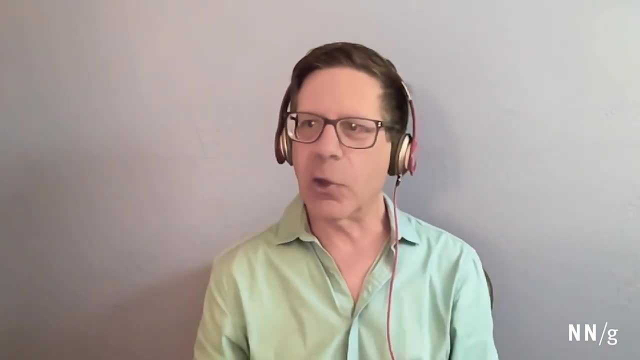 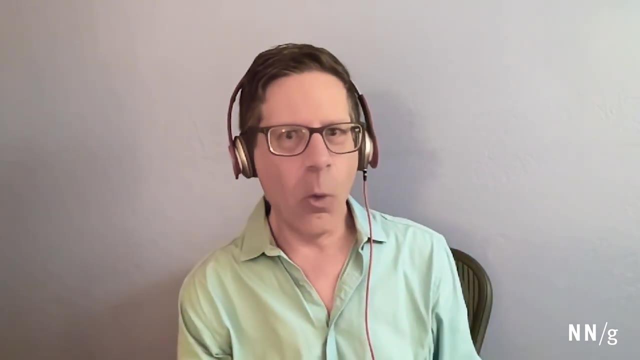 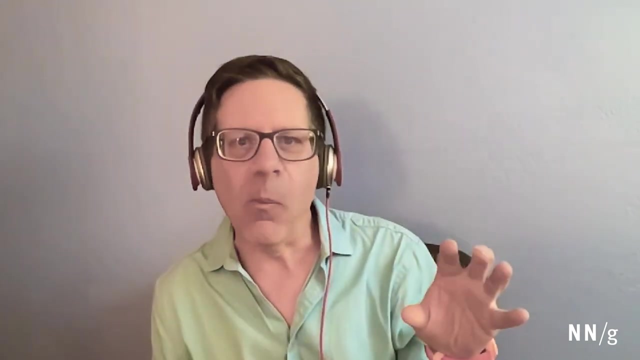 entirely stock and they still, and they just stare at you and so you don't know. uh, you know, at a sort of a gut level, it's uncertain. is it okay to ask this question? what's the person going to do? and so i think our naive self tries to be quote: helpful. let me be helpful to the person and sort: 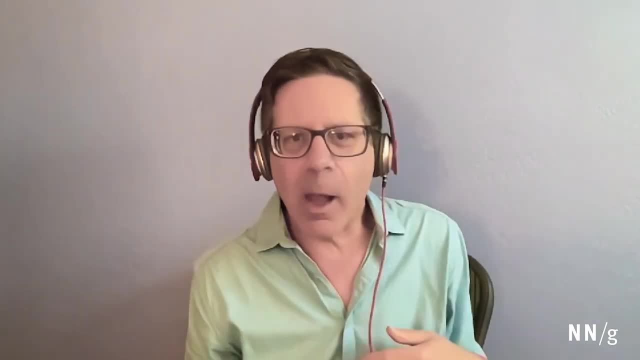 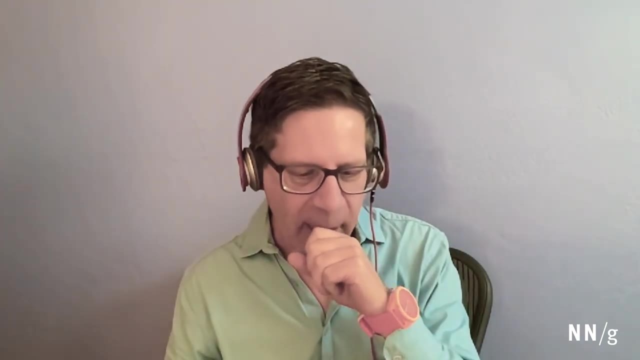 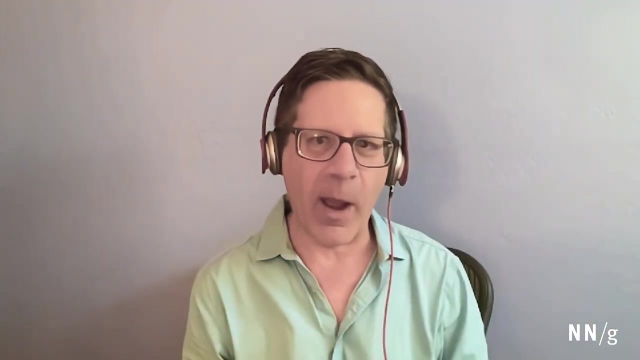 of lower the lower the intimidation factor, and so i'm gonna like help you with the question by making some suggestions as to what i might mean: um and uh, so. so that's that's why we're doing it. it's anxiety provoking to ask the question: what did you have for? 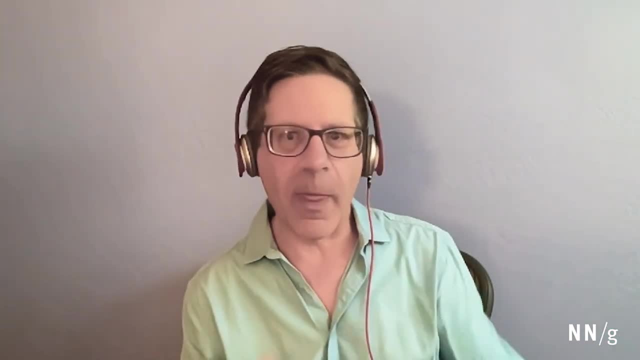 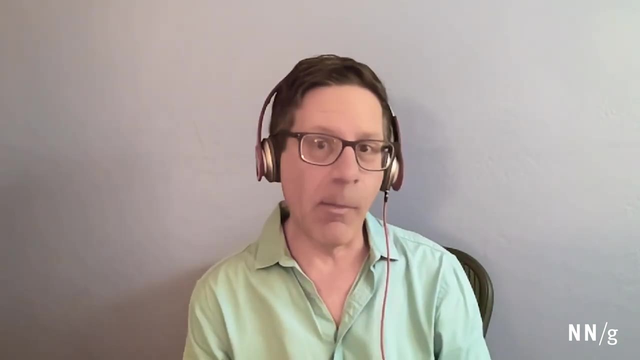 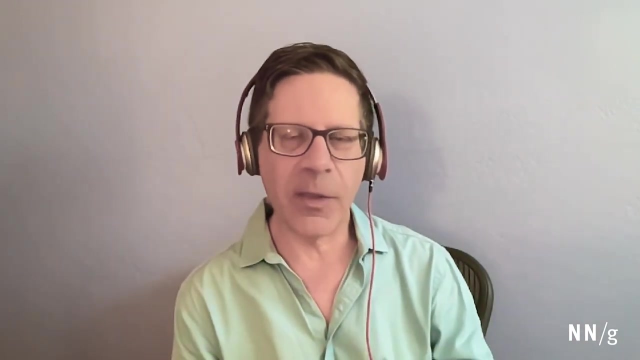 breakfast stop. that is tougher than the, the, the drawn out question. but the problem with that is um it it turns it into like a multiple choice question and it it starts to position you as the keeper of the right answers. and i think what we don't realize as interviewers. 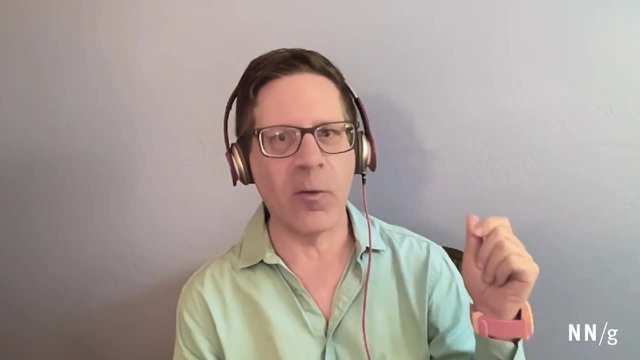 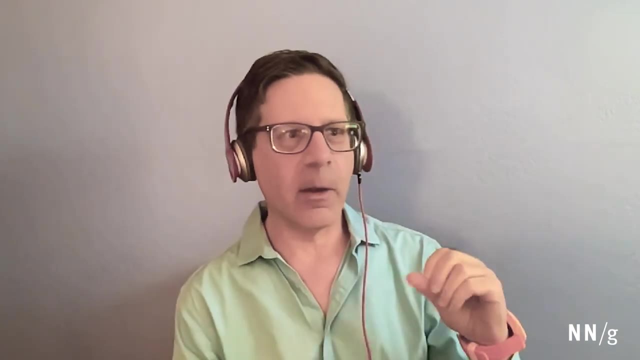 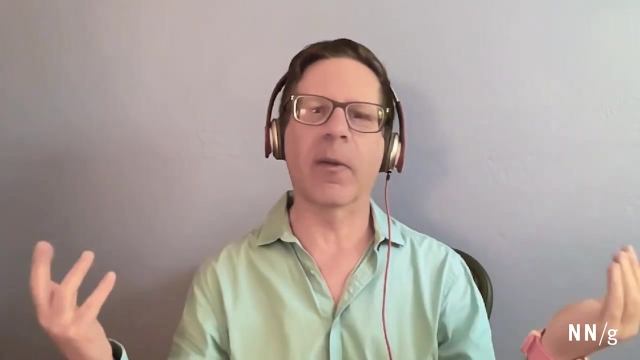 unless we've been on the other side- is how much power that interview has uh to the participant and how much that participant wants to do a good job, and that goes against what you're trying to accomplish. you do don't want that power. you don't want them to be pleasing you to be reflecting your mental model, your list of options. 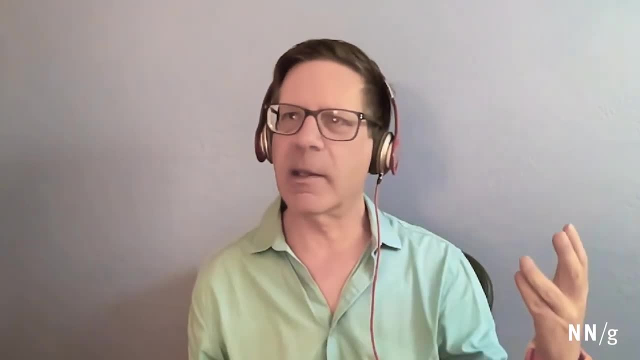 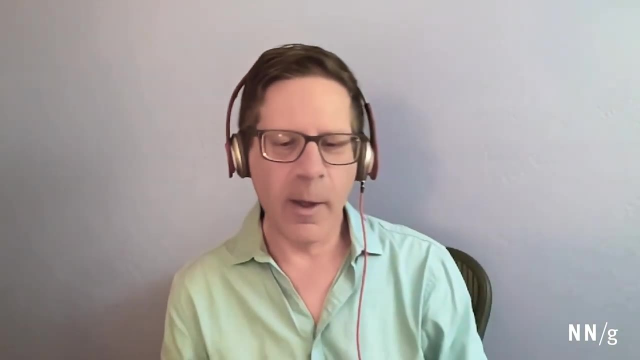 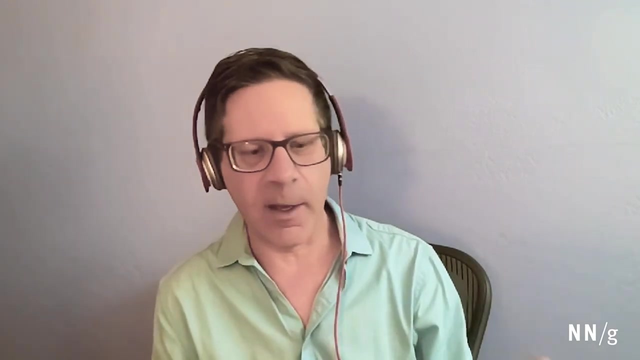 um, and so you know. i think if you're new to this, you might hear my example and say, like you know. so, yes, you said um, you know, juice, toast, uh, cereal, and if the person had pizza for breakfast, they can just say, no, no, i didn't have any of those things. what i had was pizza and 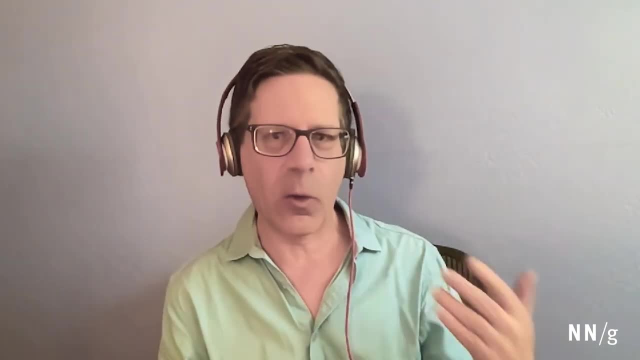 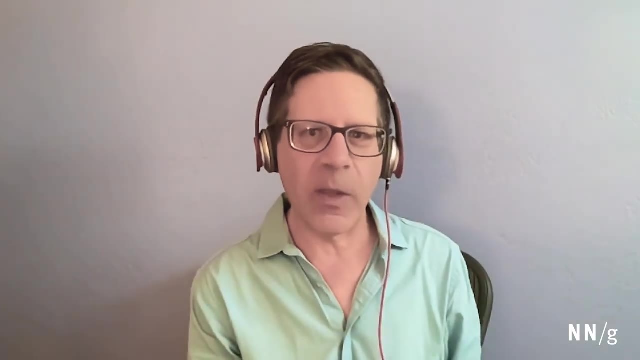 And maybe the first time they'll kind of push back. but eventually, over the course of this interview, the more you tell them what a good answer looks like, the more they are going to, without really thinking about it, you know, adapt to the rules that you're training them on. 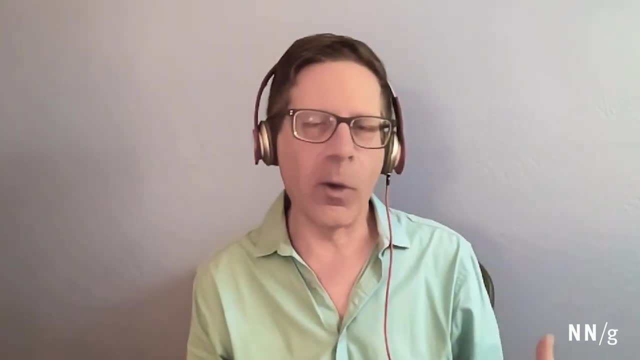 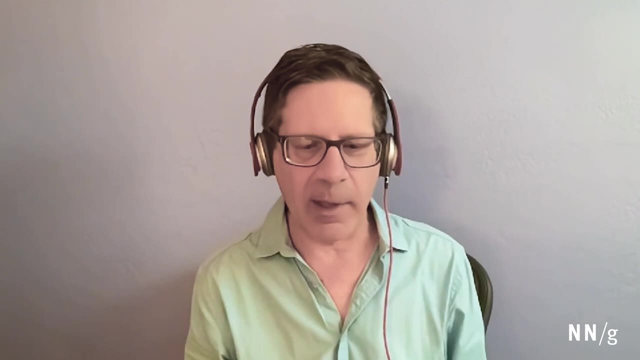 And so you'll get them. you're reinforcing your power and you're going to get answers that reflect back what's in your question, Um, and so you miss the chance to get an answer that falls outside of that, that list, And you're not trying to give them a complete list. 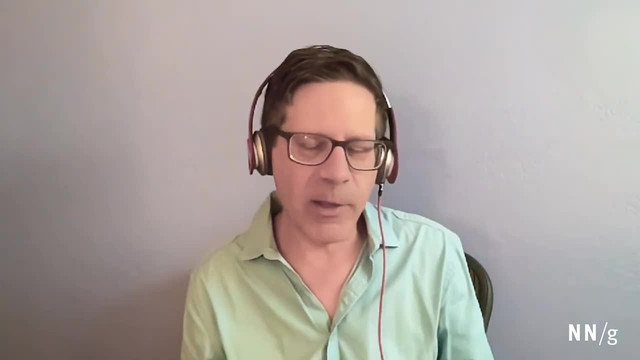 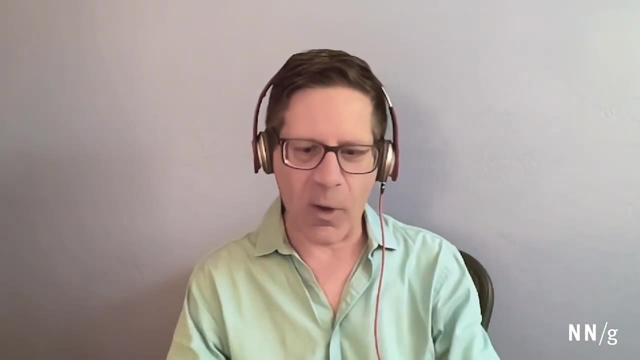 You're trying to give them for examples, but it doesn't come across that way. So, um, again, this is very, very hard, uh, which is why I'm like unpacking it so far, Like, and I think people will find: oh yeah, I do that. 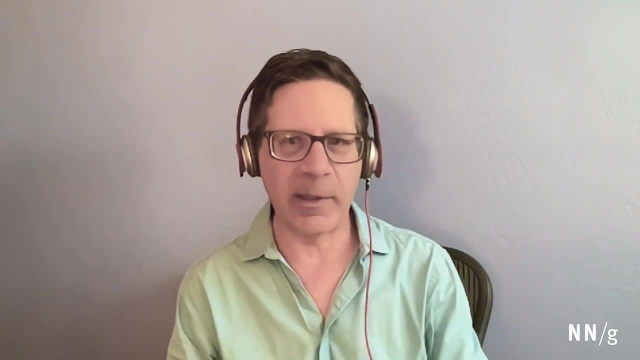 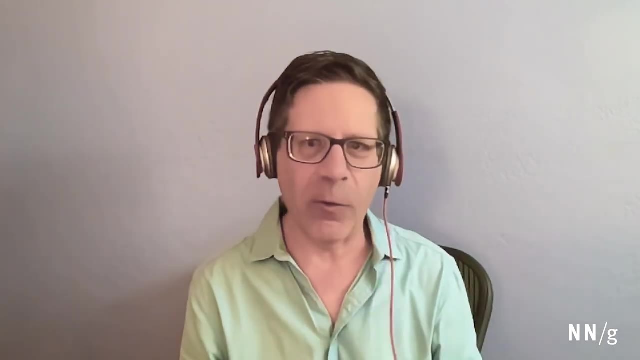 I mean, I hope people recognize it either now or the next time they do it, not because I want anyone to feel bad, but because I want someone to do Exactly what you're talking about, which is like be aware of your kryptonite moments and like just try once not to do that and feel that discomfort. 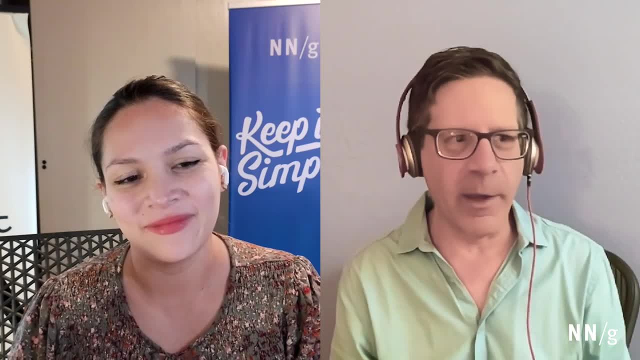 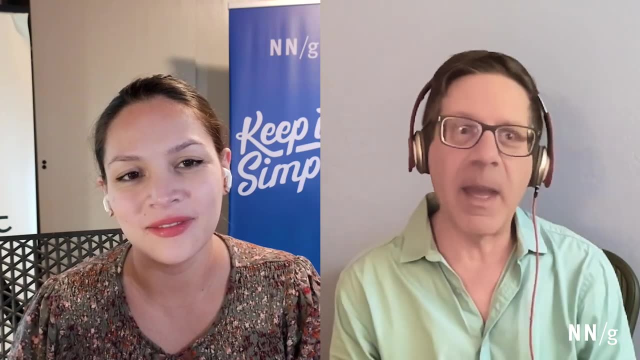 Like that's, that's the thing to kind of work on. So, anyway, that's one sort of simplistic and yet, I think, deceptively challenging piece that I think can make a big difference in the quality of the interview and what you're learning from that. 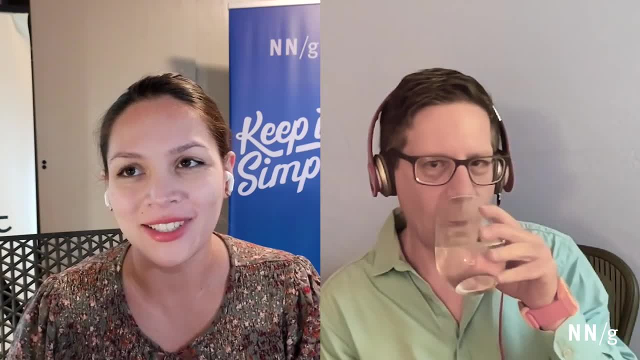 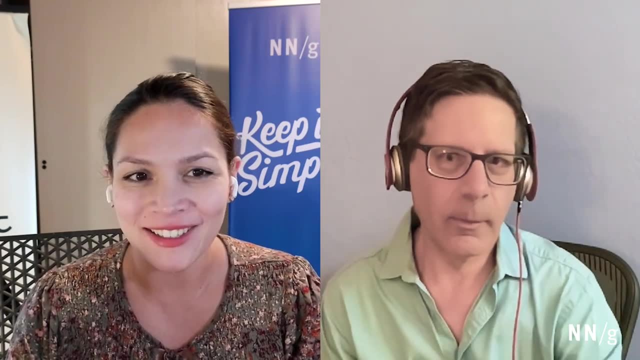 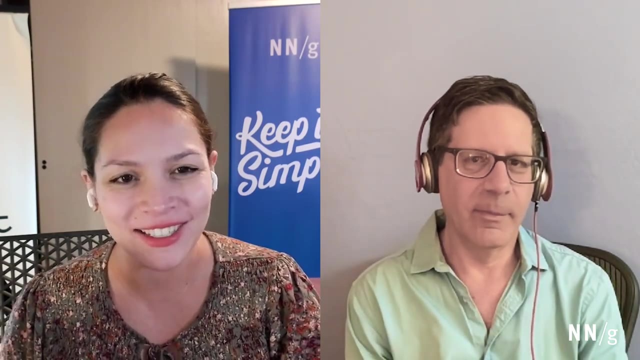 I absolutely agree. And For those who aren't listening to or aren't watching the video version of this podcast: uh, the entire time Steve was just mentioning this, this particular quirk, I was smiling and laughing because I do this precise thing all the time. 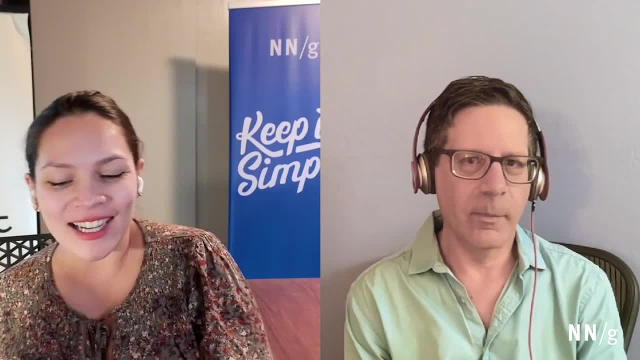 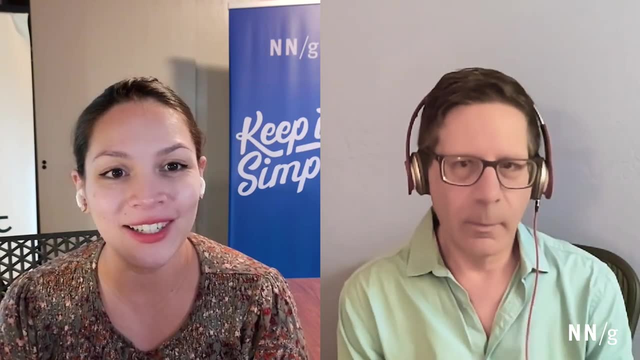 Not all the well. I've been more aware of it more lately, but uh, but it is one of those things that when I was especially a less experienced researcher, I did way more often, And it's something I've been trying to do a lot less. 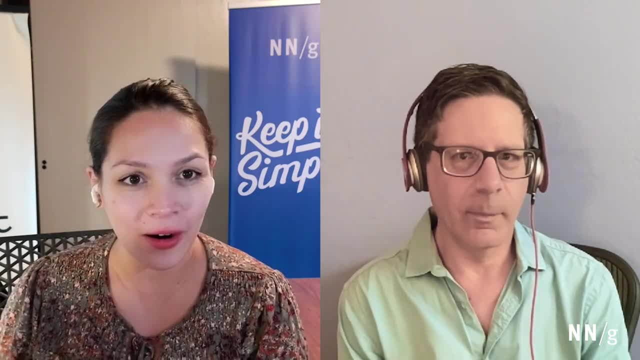 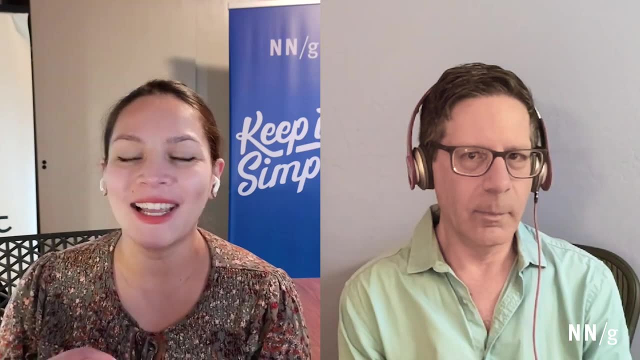 It's Hard because, like you're saying, turn-taking is hard. but when you're also hyper aware of that turn-taking, even if it's in person but especially remote, it is hard to stop And um, and it's also hard to not help. 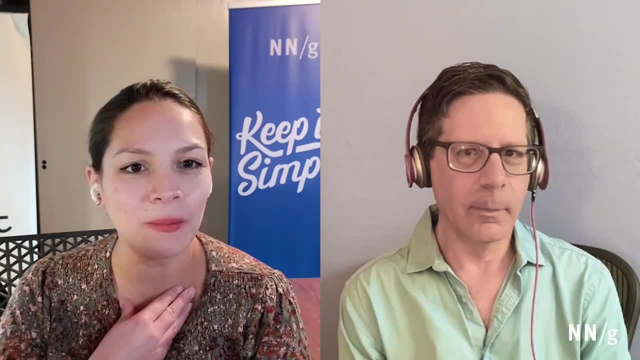 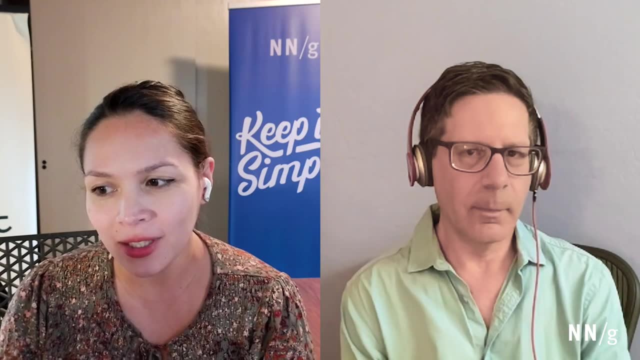 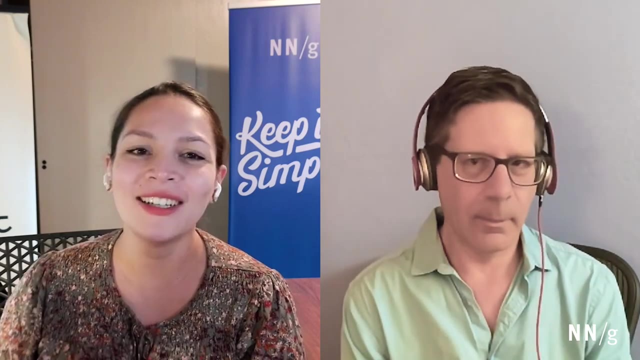 And one of the things that I noticed about my interviewing is not just helping by offering examples, but sometimes helping also would look like: oh, I want to be A relatable person, I want to connect with this person even more. So I'm going to share a little bit about my life experiences, which, for a podcast, that's fine. 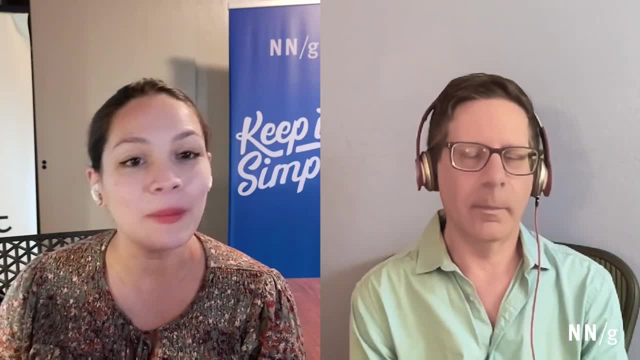 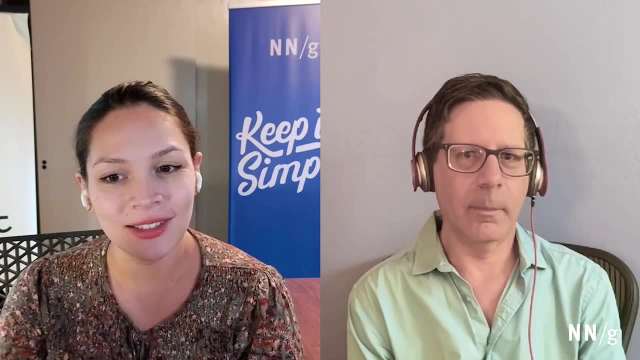 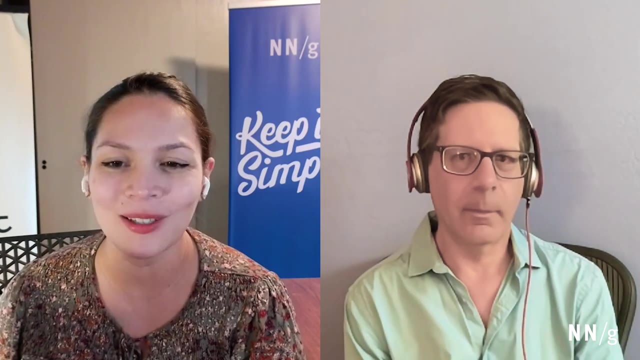 But for a research interview. that might not be fine, because then I'm starting to offer examples from my life that might Taint this person's actual accounts of what they do in their life, or maybe they'll realize that they don't relate with me after all, because they had a totally different experience. 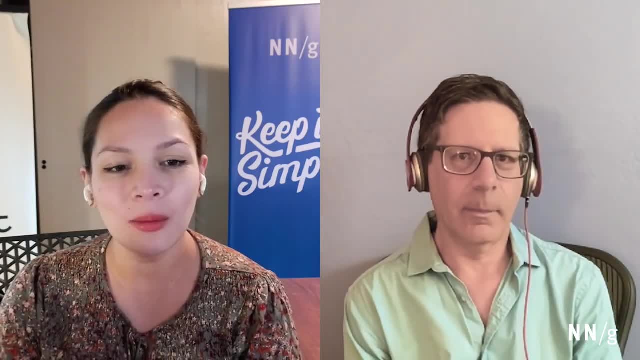 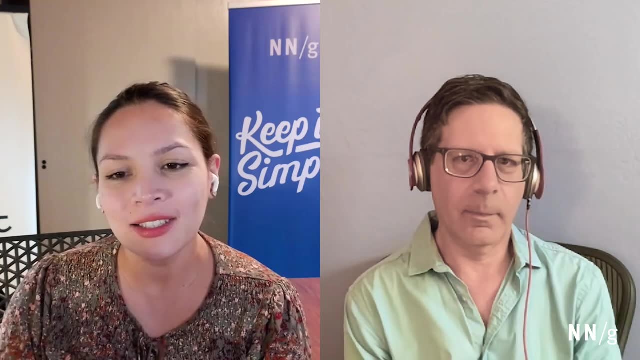 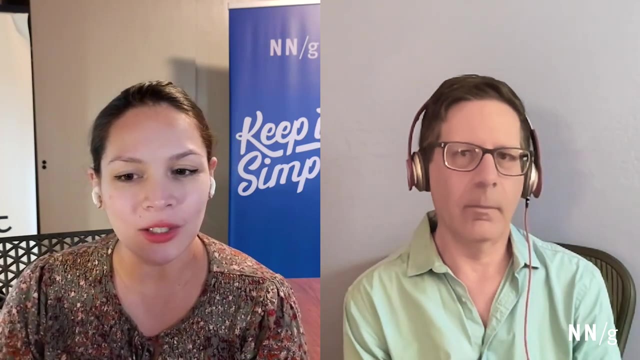 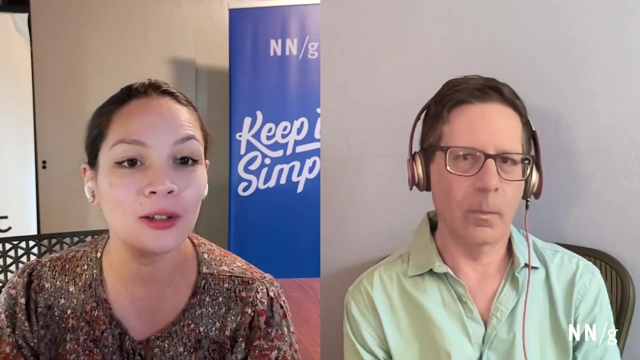 So I think that- And I like how you framed it as trying To help, because I don't think we do this maliciously or narcissistically, but out of this desire to help and connect- And I think, if we can kind of catch it in the moment and find a way to frame the way we're asking questions, as my helping should really be focused on asking this question as clearly and concisely as possible. 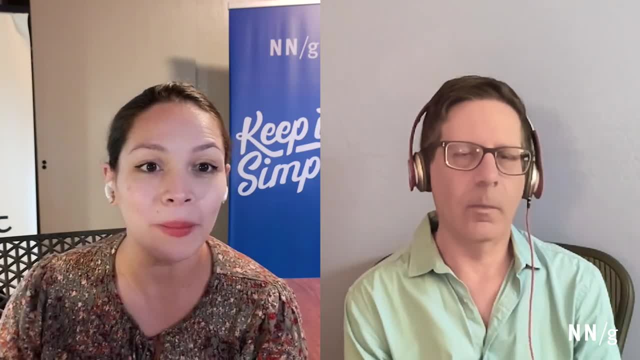 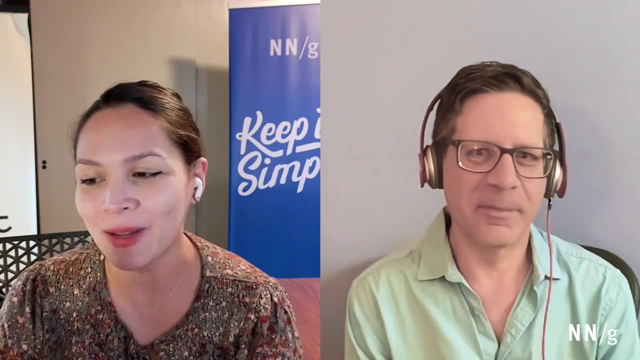 Like that's going to be a much better use of my time and certainly a better way to help. So I appreciate you sharing This, and it did kind of give me a moment of pause too, And maybe I'm starting to get a little nervous now. 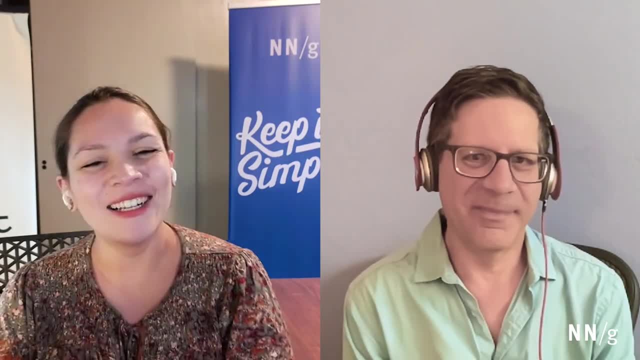 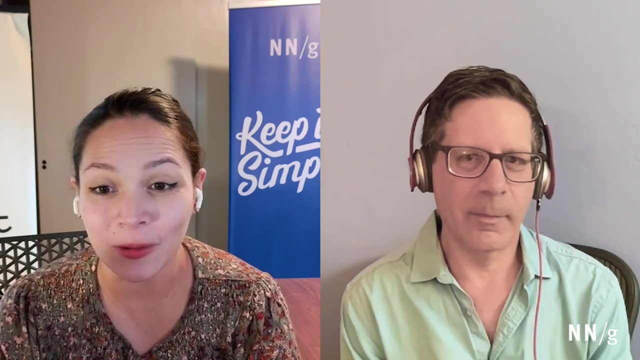 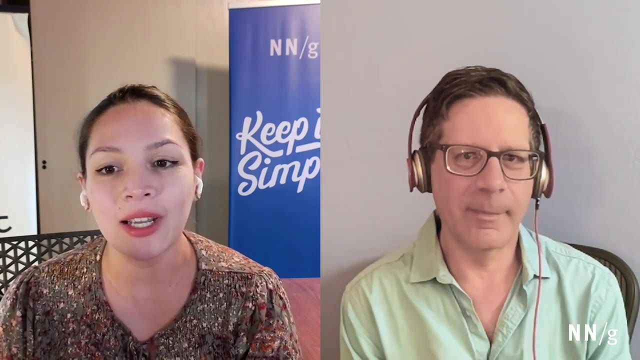 Like, oh no, did I do this for the whole interview? But hopefully I've I've done okay for this batch. but anyway, Steve, I just wanted to say thank you for sharing this advice, for sharing all of these great pieces of insight about interviewing. 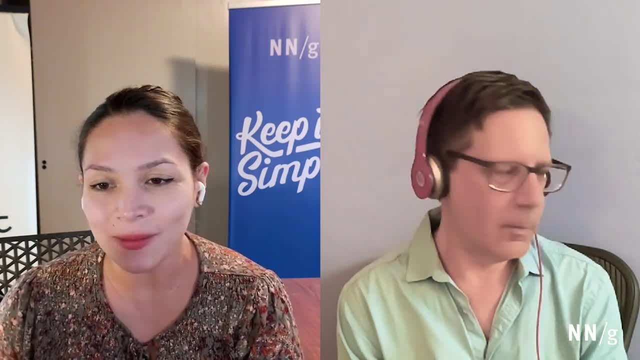 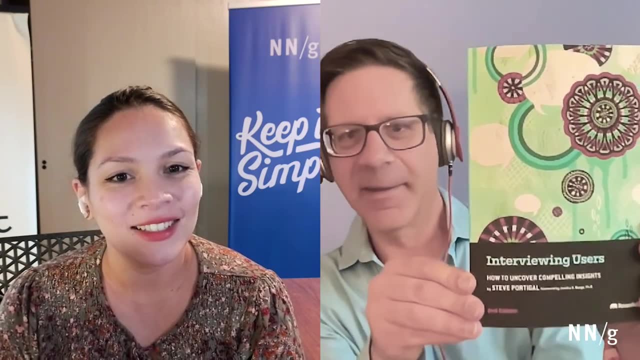 And I think it's going to be amazing to read your book. Um so, for those listening, I'm going to hold it up. Interviewing Users: I'm going to hold it up for those watching. There's a copy, Yes. 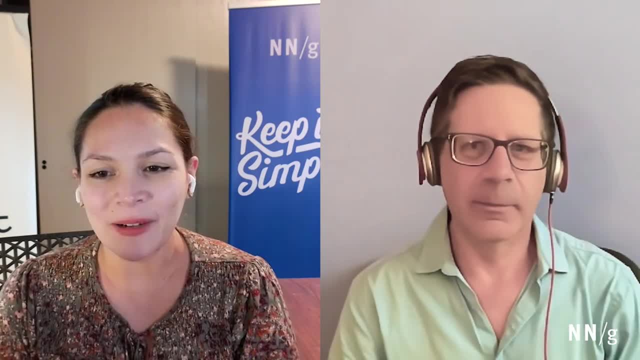 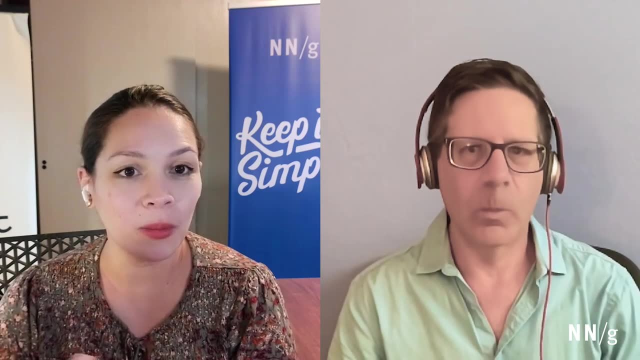 Yes, So this is the interviewing user, second edition. Um, and you know, make sure to check that out. Um, but, Steve, if anyone wants to follow you and your work is there anywhere, you can point them to website. wise social media handle wise. 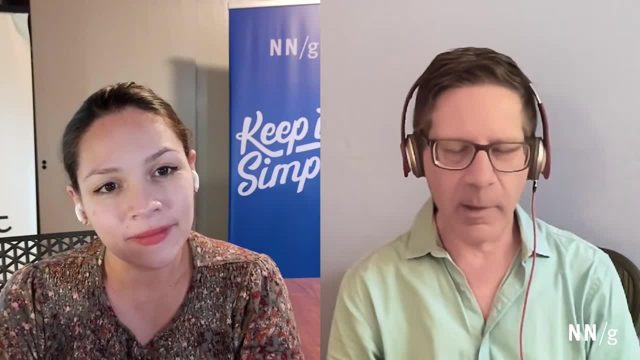 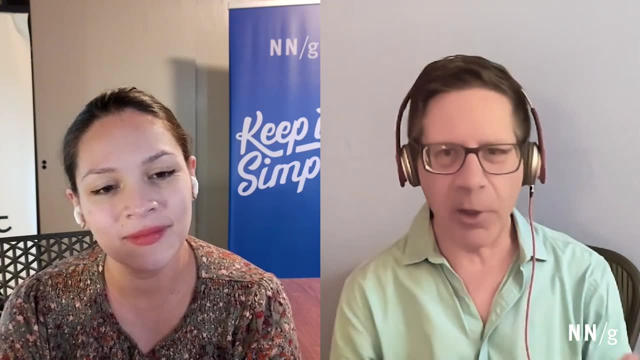 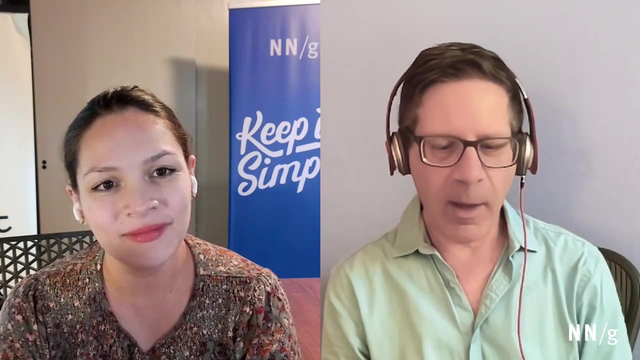 Yeah, Two places. Um, my website is my last name, Portugal, Portugalcom. Um, so you know I post. I'll post this here when it, when it comes out. I try to keep up to date on things that I'm doing that I have to share. um, and you know, social media- probably LinkedIn, I think, would be, uh, the best place. 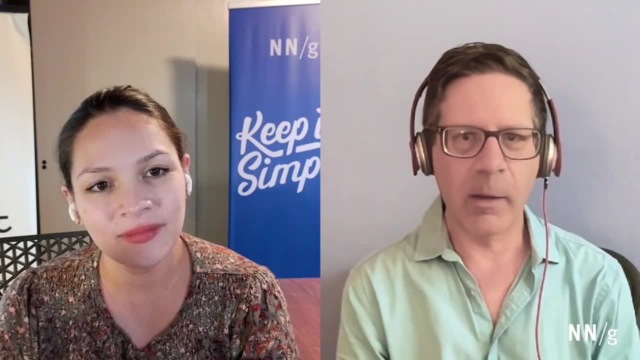 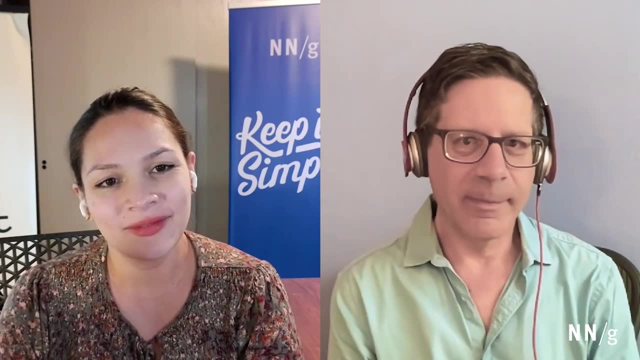 So it's yeah, my name on on LinkedIn. uh, I love people to be there and and uh get to chat with them- Awesome. Well, Steve, thanks so much for your time today. It's been a lot of fun interviewing you. 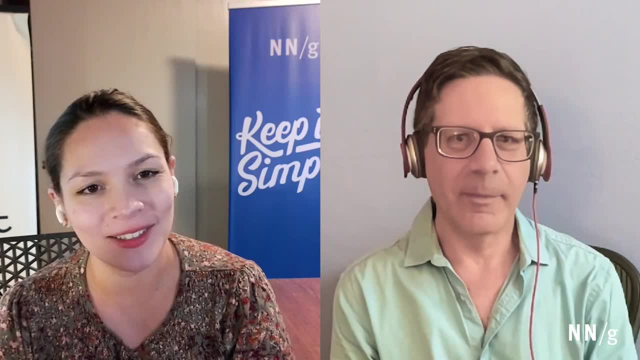 Uh, and it's given me a lot of time. It's given me a lot of food for thought as I think about my own interviewing practice. So thank you so much for your time and hope you have a great day. Thanks, Thank you. 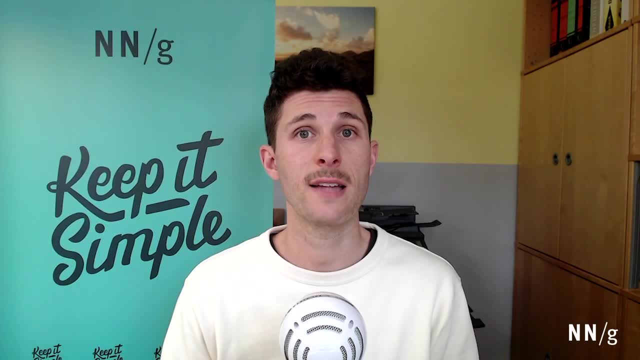 And same to you. Thanks for listening to today's episode. If you want to learn more about UX, a great place is to go to our website. There you can find thousands of articles, videos and reports about UX. This website is wwwnngroupcom. 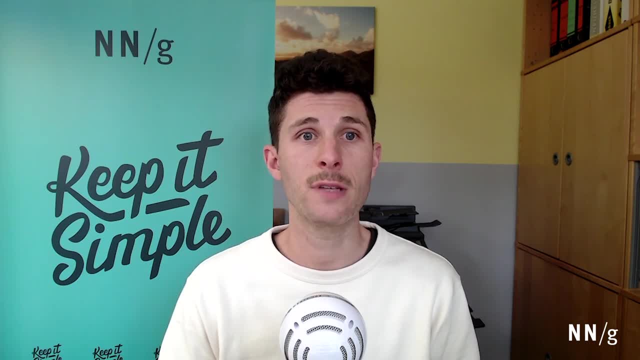 On that note, if you want to stay up to date on our latest research and publications, we do have a weekly email newsletter which features our latest articles, videos and upcoming online courses, And if you enjoy this show, please follow or subscribe on your podcast platform of choice. 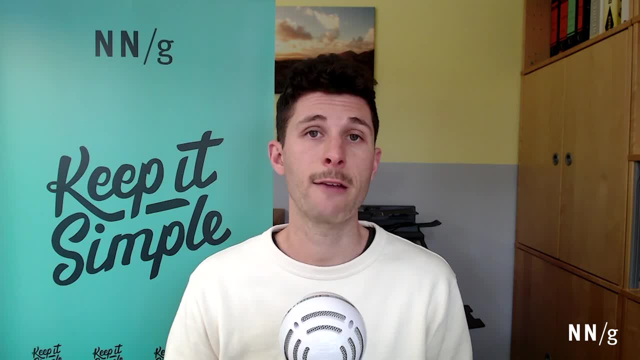 This episode was hosted by Therese Fassenden and produced by me, Tim Noiseson, All editing and post-production. It's by Larry Moore Production Company. That's it for today's show. Until next time, And remember, keep it simple.